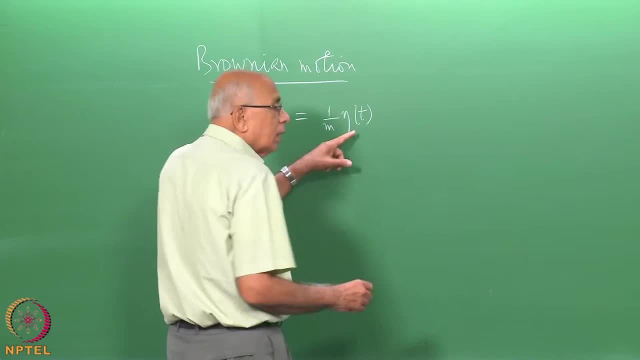 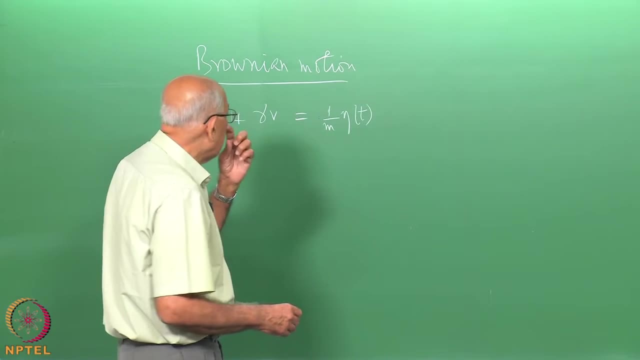 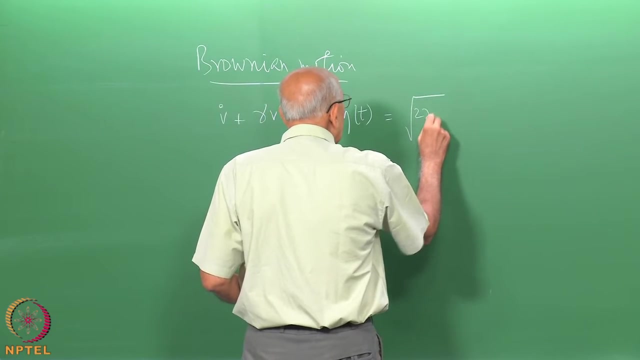 noise, and we also discovered there was a relation between the correlation, the strength of this force and the friction constant gamma. If you put that in we could write this. then we had a capital gamma here. so this would go to 2 gamma k. Boltzmann t over m times zeta. 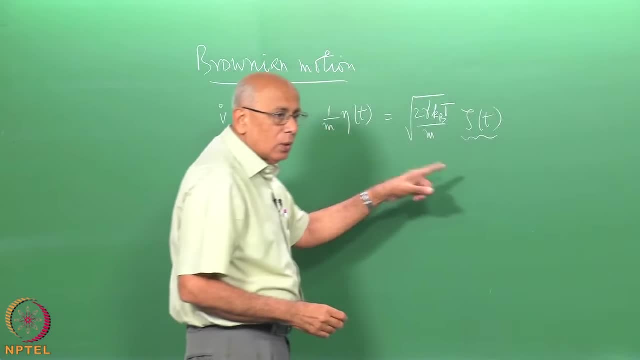 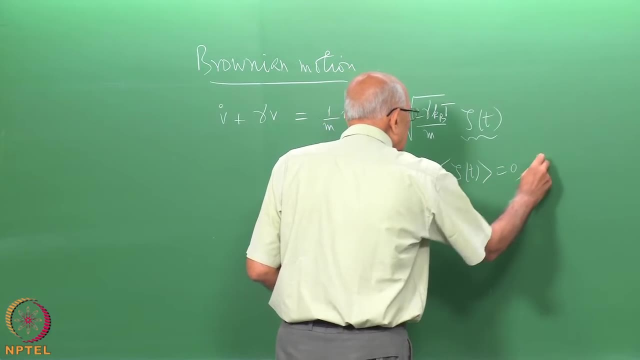 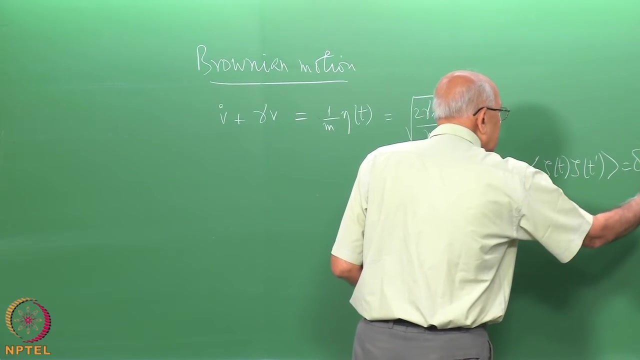 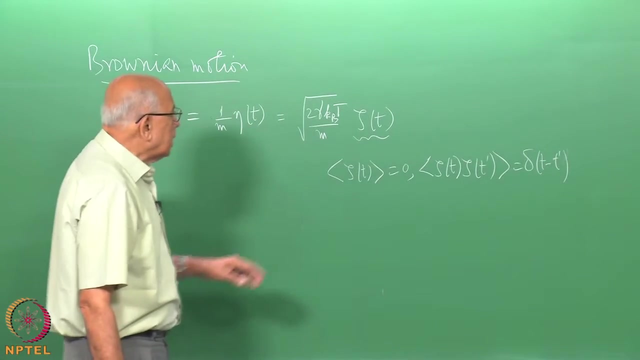 of t, where this white noise had the following properties: it had 0 mean and zeta of t prime was equal to just a delta function: delta of t minus t prime. Ok, I slurred over the fact that this quantity is not very well defined. it is too singular. 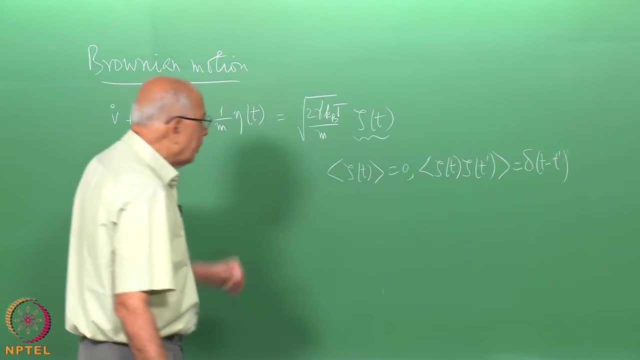 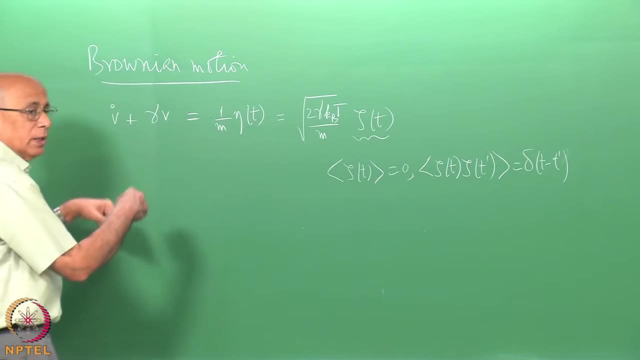 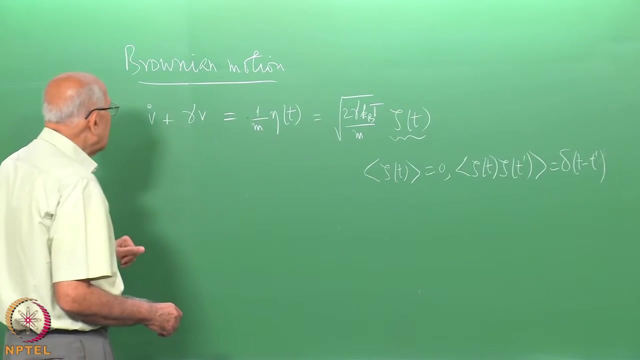 in some sense, That is, in a strict mathematical sense. So we will come to terms with that now and do this little better than what we did earlier. Now, of course, in the diffusion regime what happens is, you know, at long times, t compared to gamma inverse, and then the effect of this. 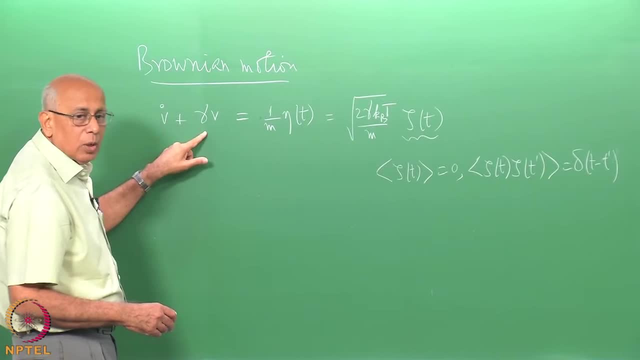 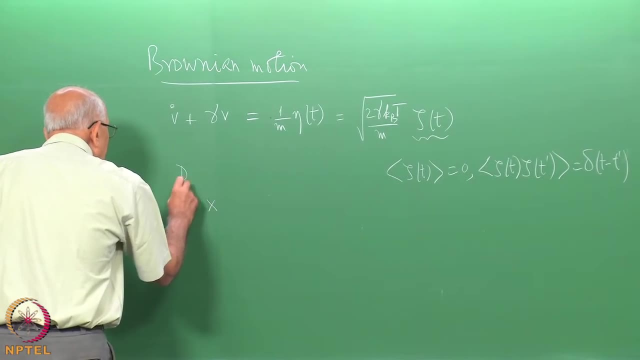 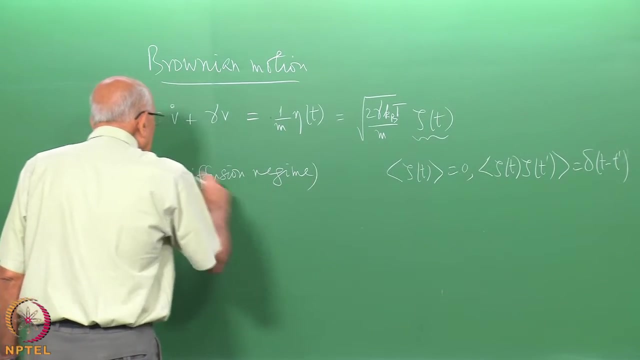 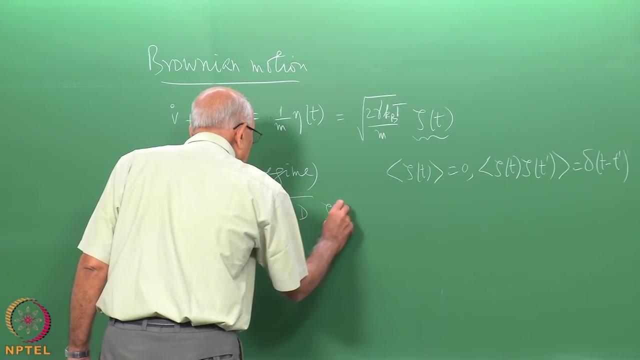 inertia get term gets negligible and this term dominates here. So let me go straight away to the diffusion regime and write the equation in the diffusion regime, What we call the diffusion regime, or equivalently high friction, very high friction. this equation gets replaced by x dot, equal to square root of 2 d times zeta of t, because recall that. 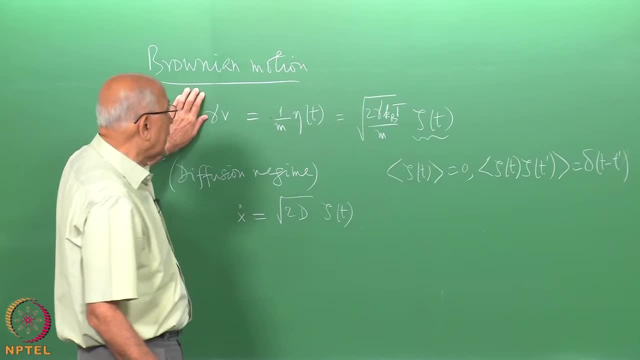 d was k t over m gamma. if I divide through by gamma after neglecting this, you get precisely 2 d here, So all this will be equal to. if I divide through by gamma, after neglecting this, you get precisely 2 d here. So all this is equal to. I am not done, I am just going. 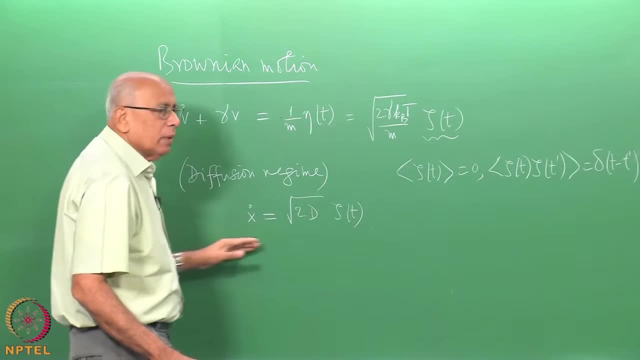 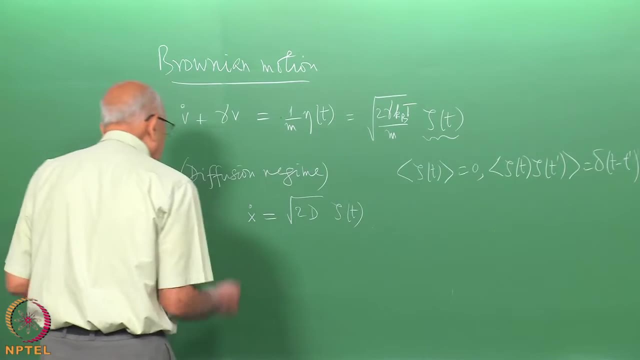 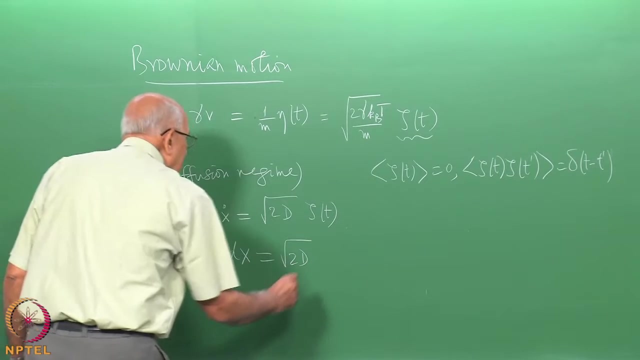 the factors are right. Now this is not a very comfortable equation to work with because it is too singular an object, So mathematicians like to write this in the following form, and I will define this term. So this is written as d x equal to square root of 2 d times d. 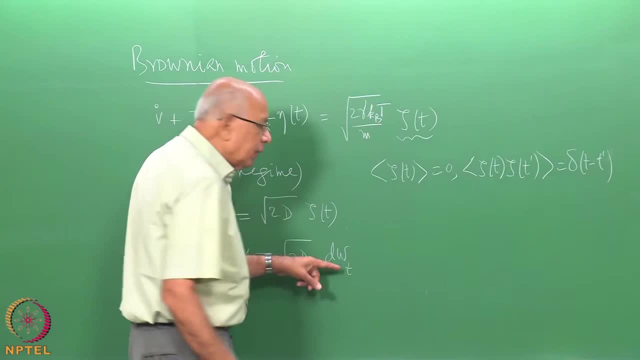 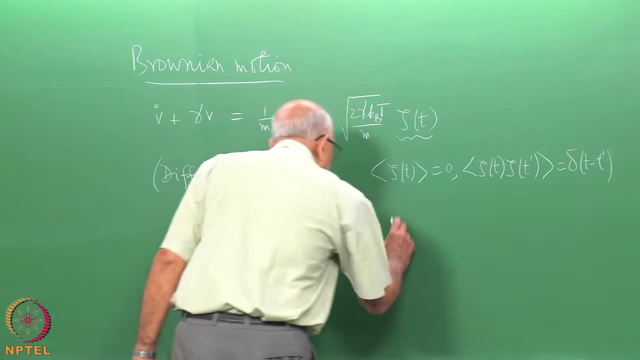 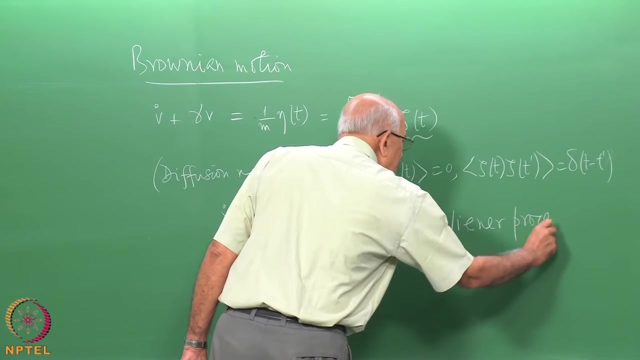 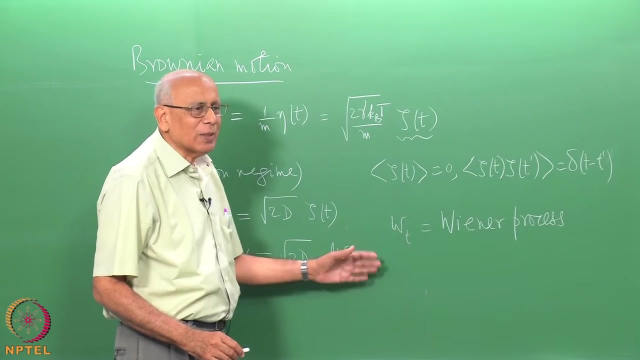 w t. this is called a Wiener process. the w of t is called a Wiener process. let us write that down. I should put a t inside the bracket really, as physicists would, but mathematicians like to put it as a subscript because it is more notationally easier to handle there. 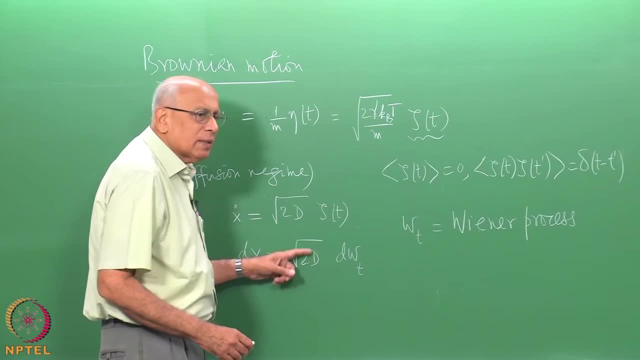 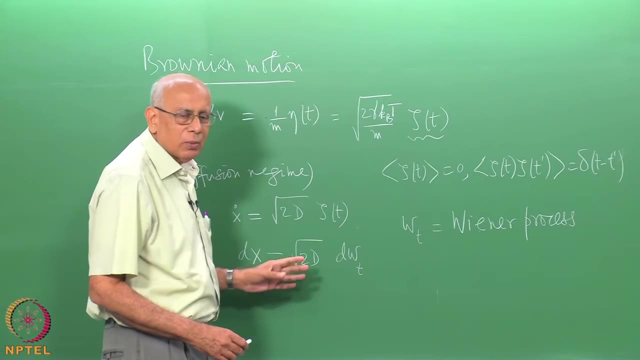 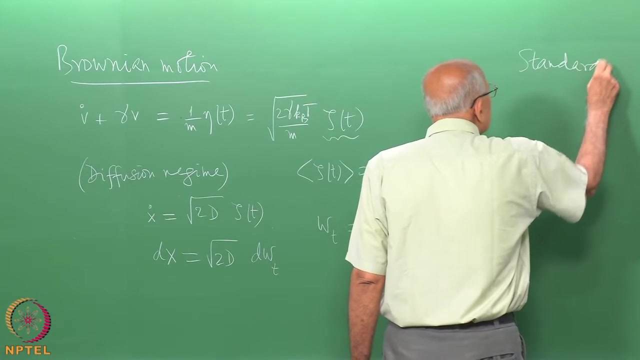 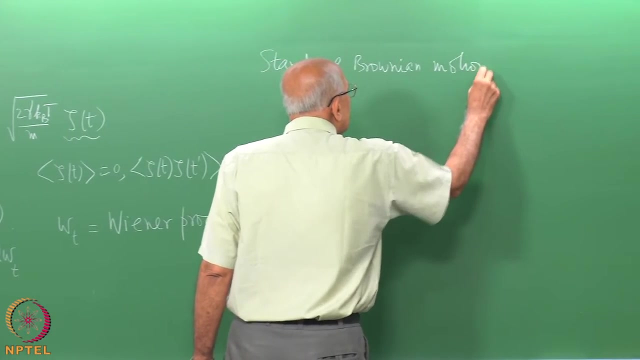 Ok, And the practice, standard practice- is to set 2 d equal to 1.. So you rescale matters in such a way that 2 d is equal to 1 and then it is called standard Brownian motion. So standard Brownian motion or equivalently, a Wiener process. 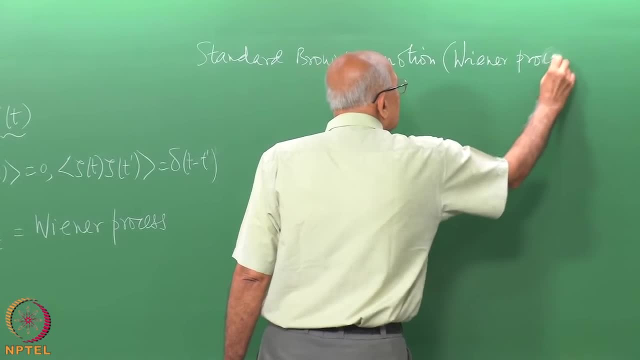 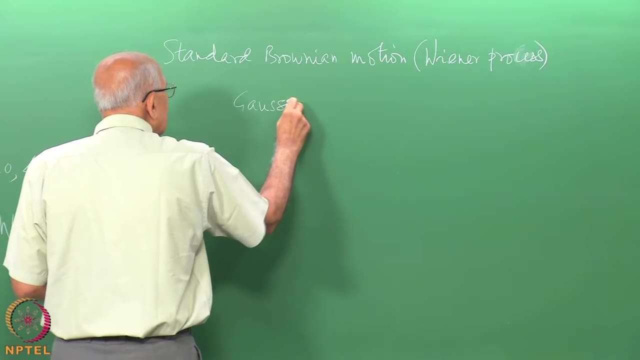 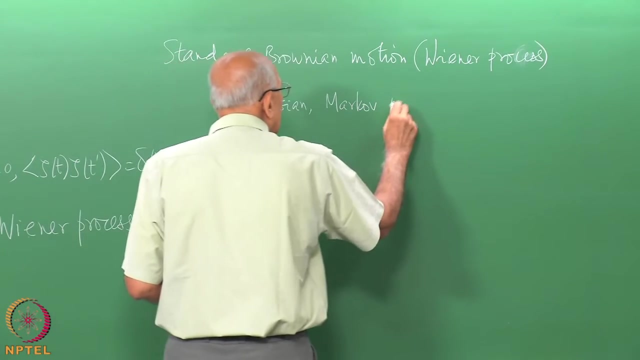 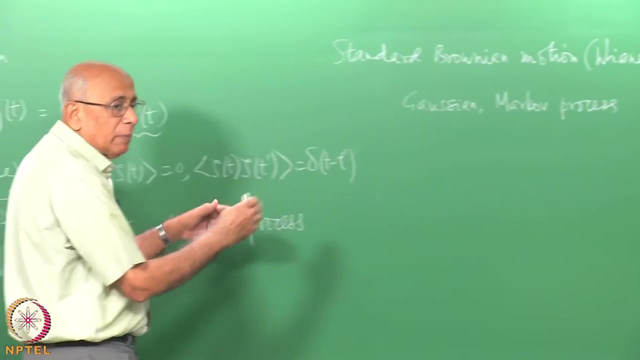 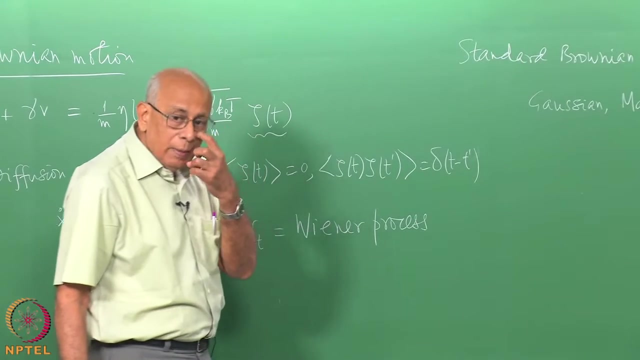 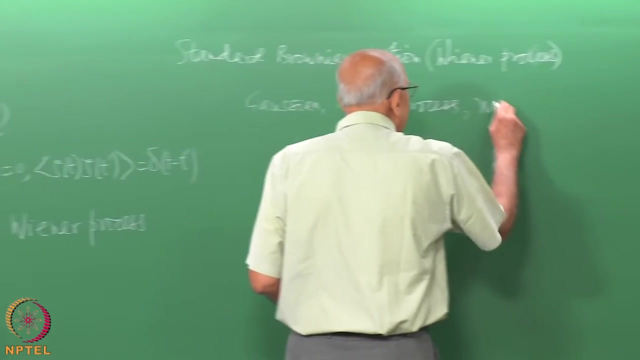 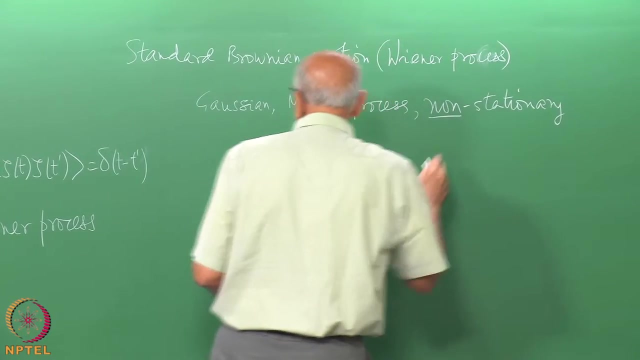 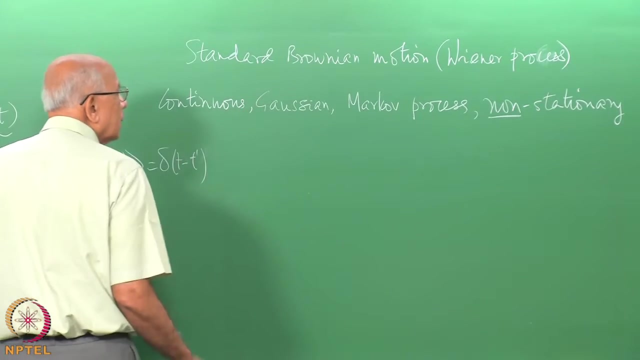 is a Gaussian Markov process that is delta correlated. that is correlated in a specific manner which I will derive in a second. Ok, This Gaussian Markov process eminently has most notable property is that it is not stationary, non-stationary, It is a continuous process. that is important. Ok, with the following: 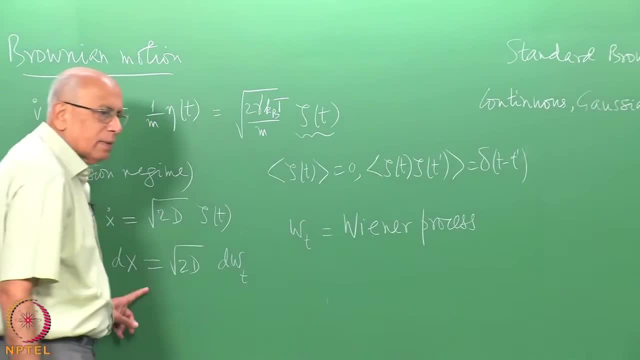 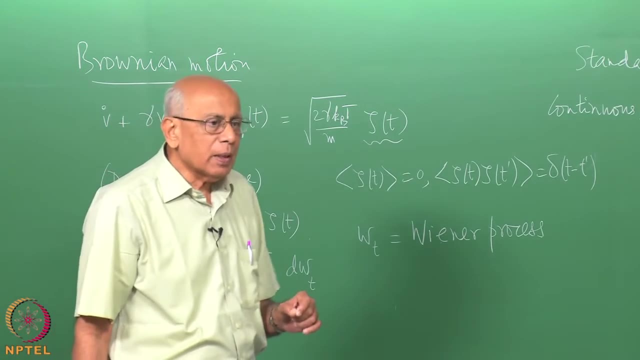 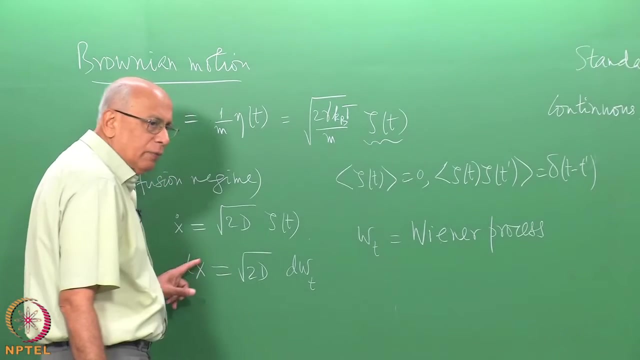 thing. Ok, Essentially it is this: x and x, we recall, is the position, instantaneous position of a particle diffusing on the x axis with the diffusion constant d and the probability density function of this x obeys the standard diffusion equation. delta p over delta t is: 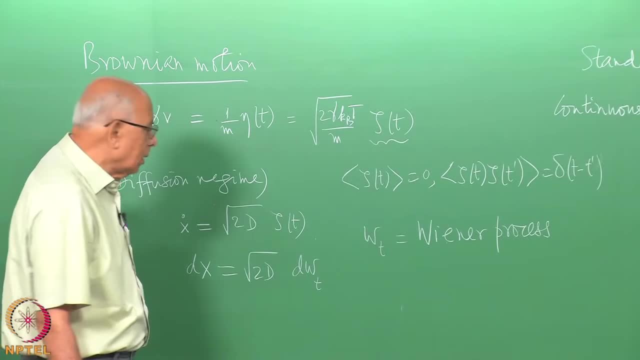 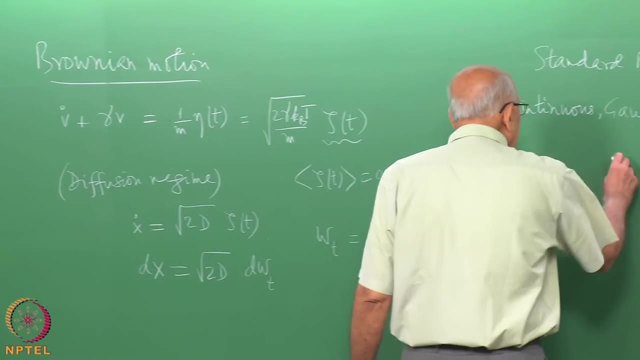 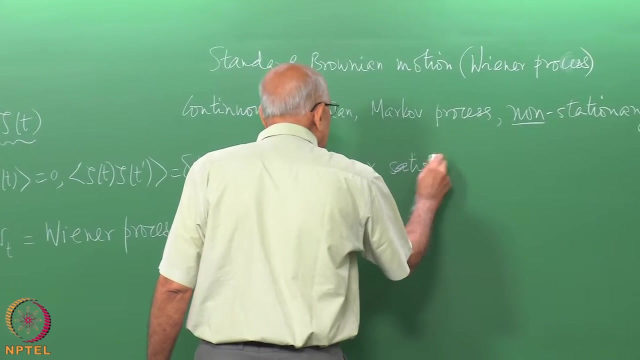 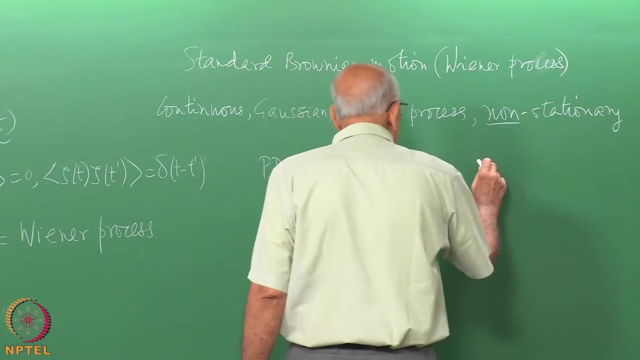 d times delta 2 p over delta x 2. but for this process here we have said 2d equals delta, 2 equal to 1, it is clear that for this w. so the pdf, pdf of x, satisfies, of w say satisfies. 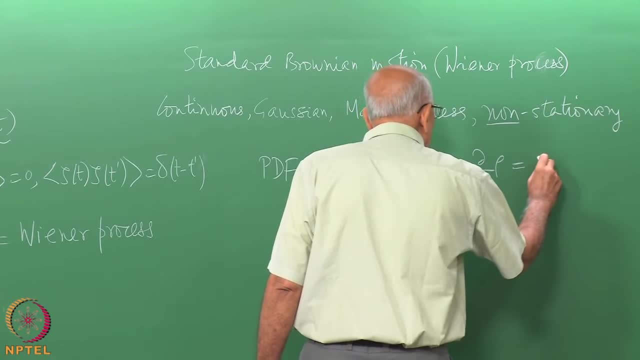 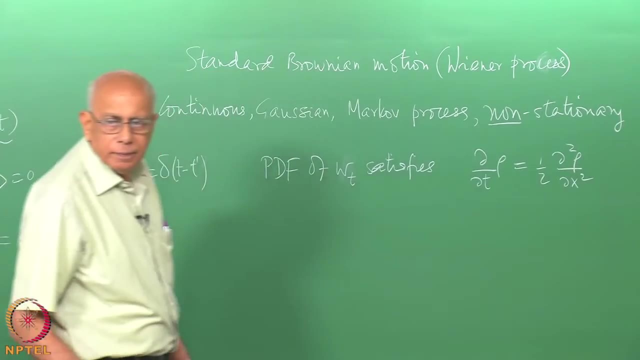 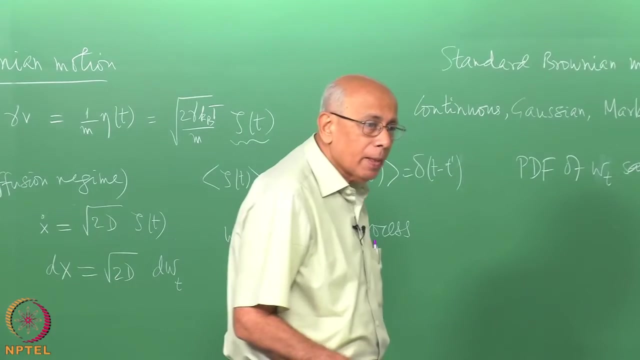 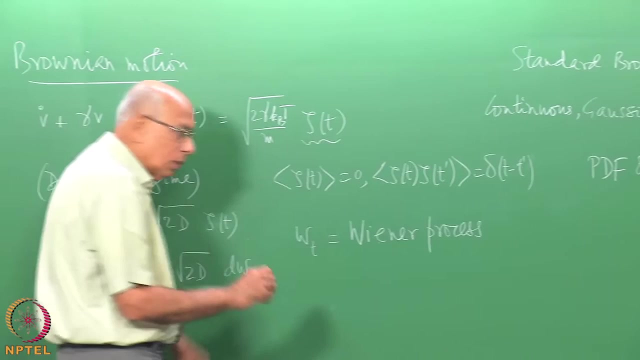 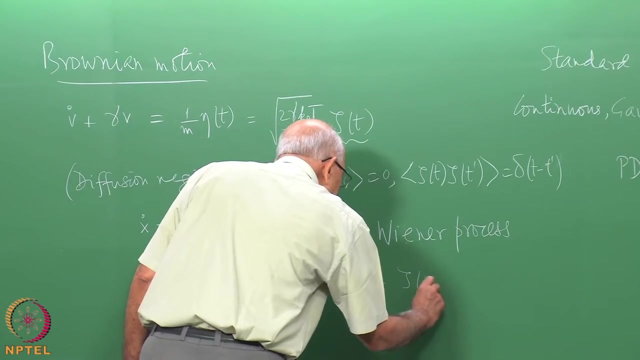 delta over delta t. let me just call it rho equal to 1 half delta 2. rho over delta x 2,. Ok, Pardon me, w of t is not white noise, it is the integral of white noise because in a crude sense, quote, unquote dwt equal to zeta of t, dt. So w of t. that is what I did. 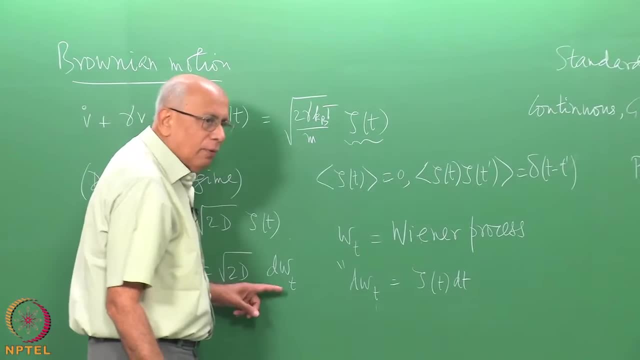 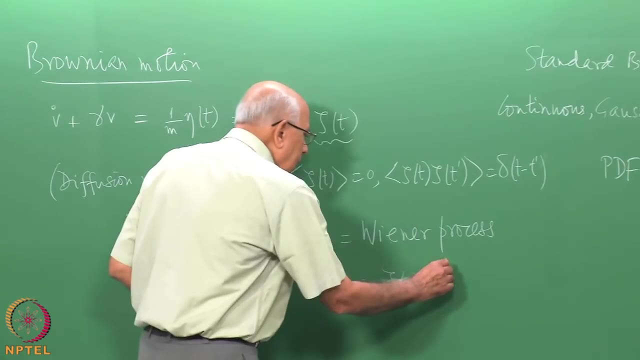 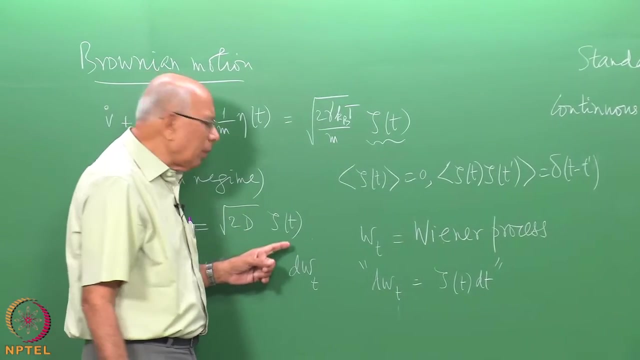 here when I wrote this as dwt. We have to be careful about what I mean by this differential, and that is the whole point, Right? So in this heuristic way of looking at it, this w of t is like the integral of white noise, because that is what zeta of t is. But the problem is that zeta of t is not. 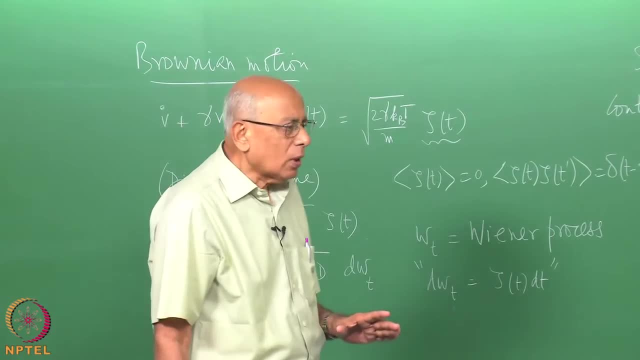 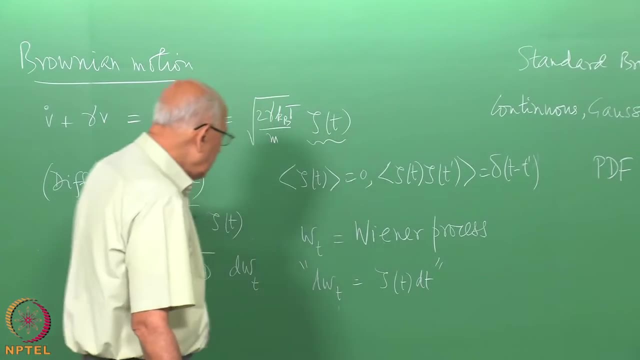 a well-defined mathematical object. It has got a singular covariance, it has got a singular correlation function, a delta function, which is not pleasant. Ok, Now think of what. so w of t is essentially x, the position of a diffusing particle. Ok, 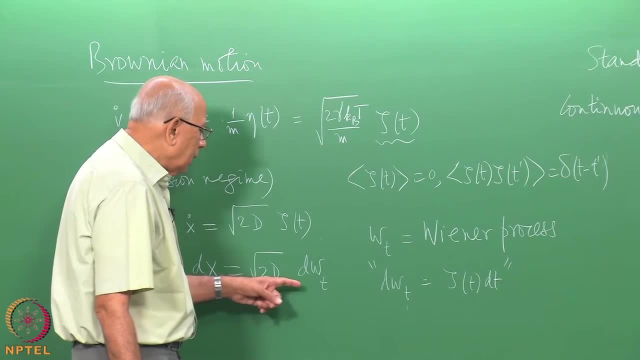 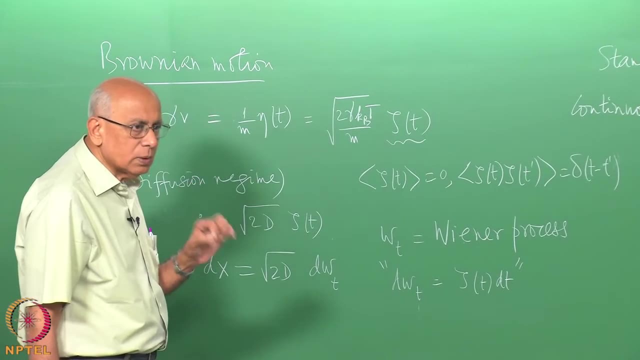 That is it, Apart from this constant here, But think we know already what this guy does. We know that it is not a stationary process and if the particle starts from zero, the origin at t equal to zero, then the position is a Gaussian and distributed by a Gaussian with. 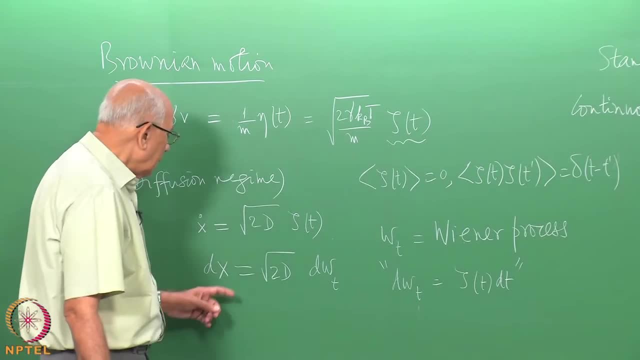 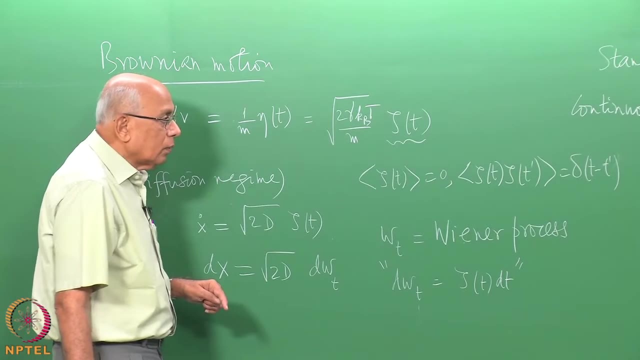 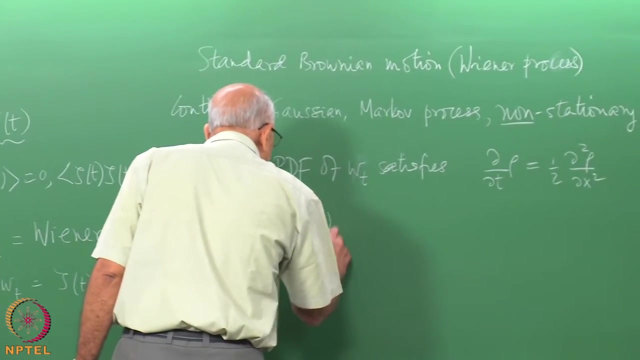 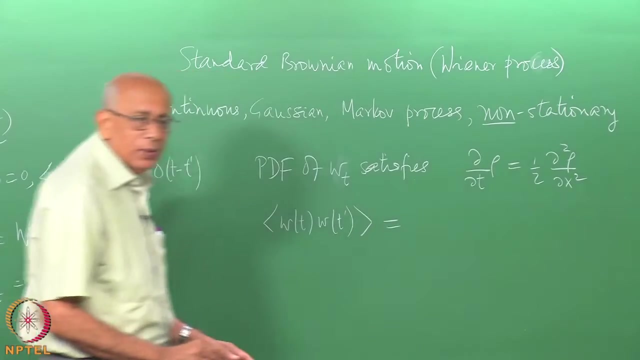 a variance increasing linearly with time, etc. And we also know that this process has an autocorrelation function which, eminently, is not stationary. So this tells you. so, w of t, w of t prime, the average is equal to. do you recall what? 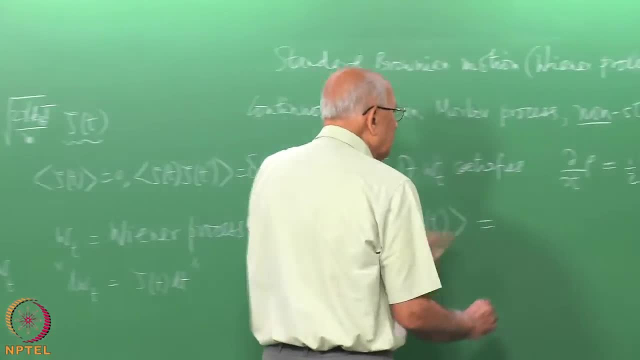 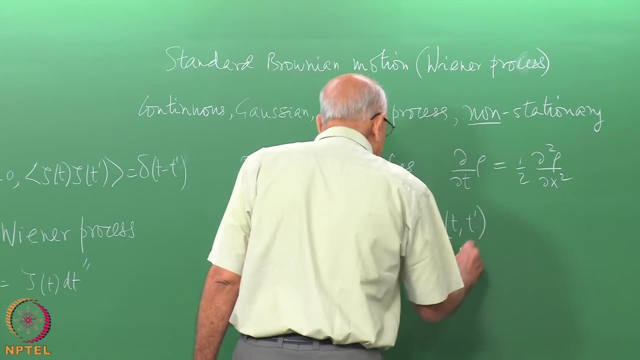 it is Minimum, Yeah, the minimum, the lesser of the two. Now we have set this 2d equal to 1, so with that normalization it is minimum of t- t prime. We are only considering positive values of t and t prime, right. 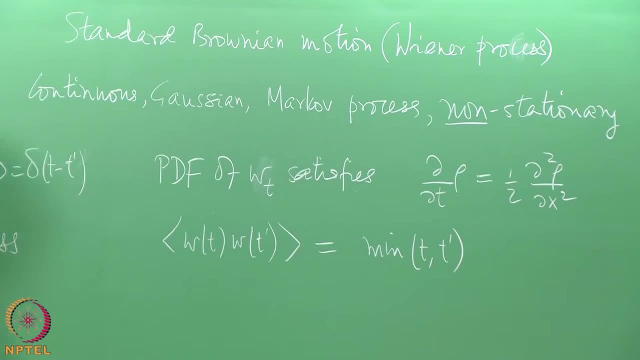 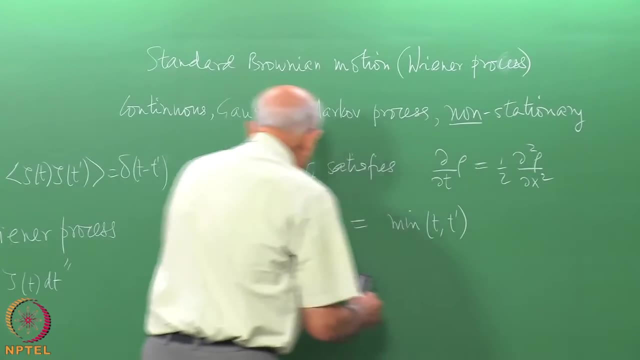 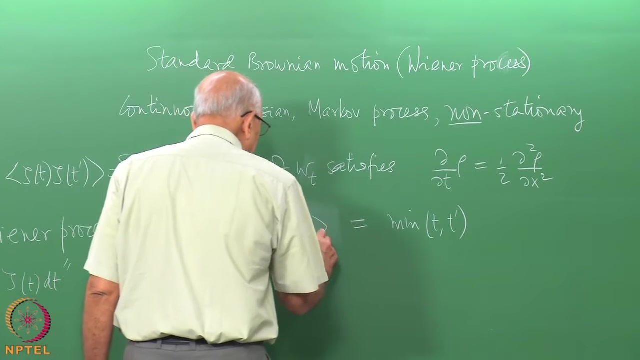 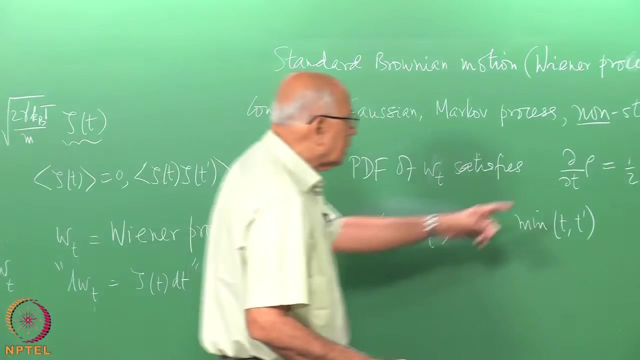 Ok, So it is clearly not stationary because autocorrelation function has this behaviour here. So let me, let me stick to standard notation like this: And this chap here has got the standard Gaussian solution, if you recall, This is implies Ok. 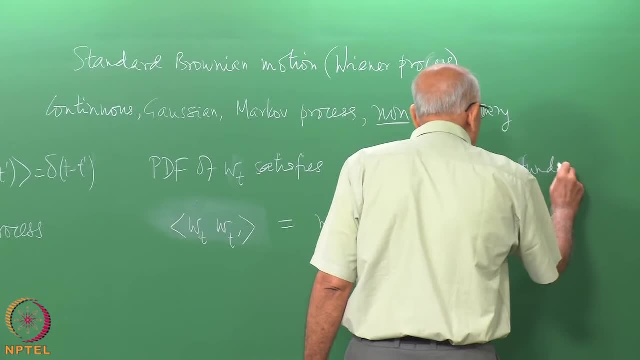 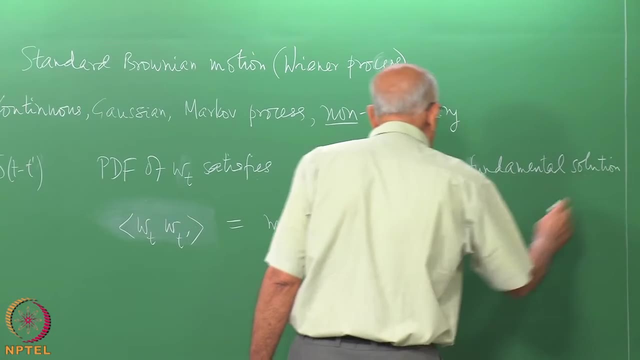 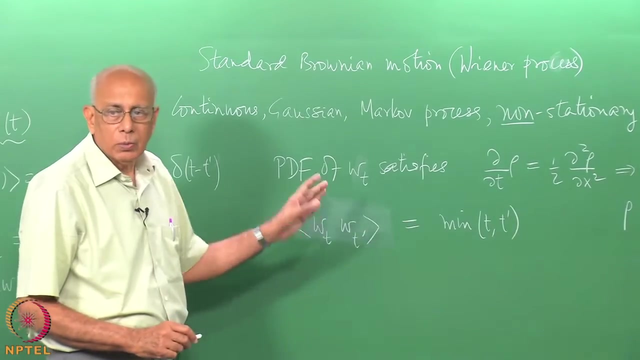 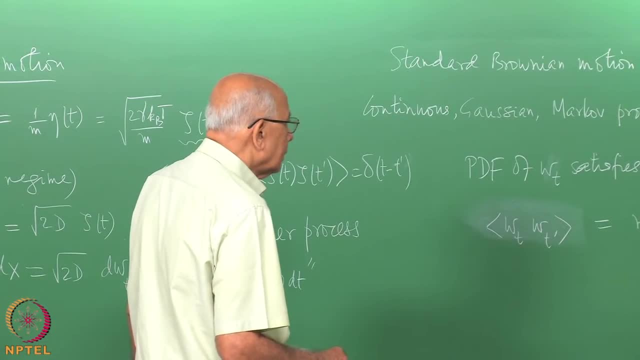 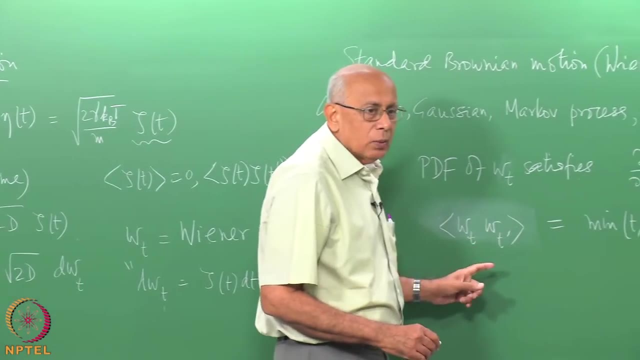 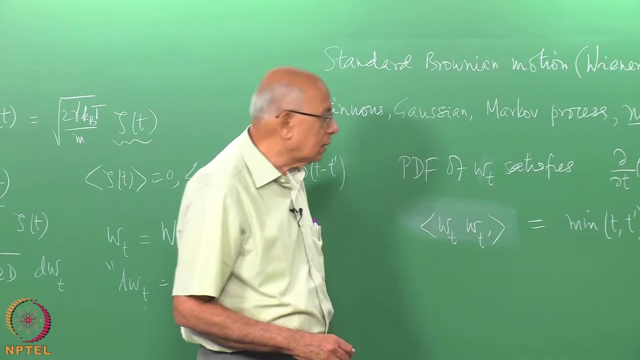 Thank you, Thank you. So this is where it came from. Now let us try to understand this a little better, What this thing is. this is the covariance of t and t prime. that is the word for autocorrelation function in statistics. If you divide it by the covariance of this, the and the standard. 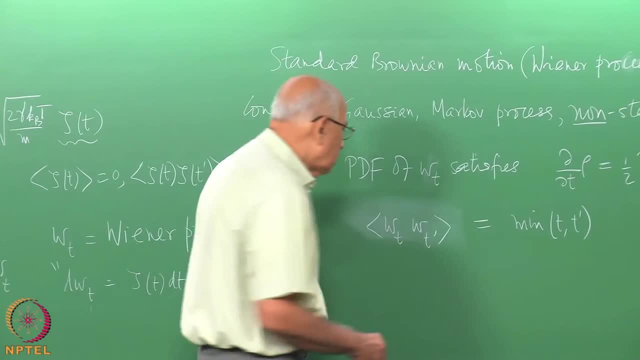 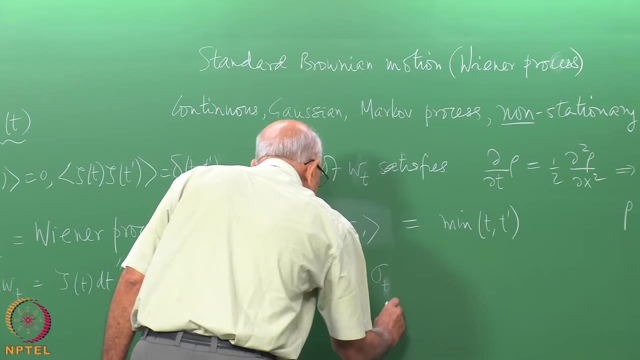 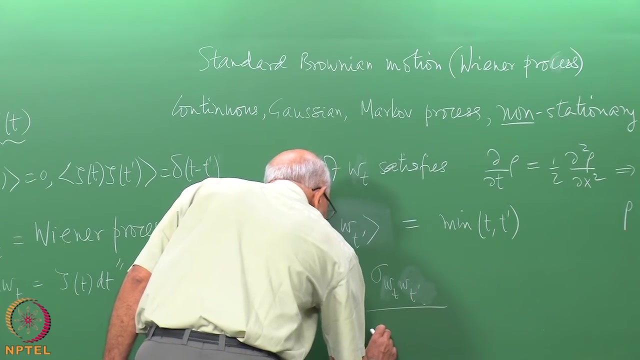 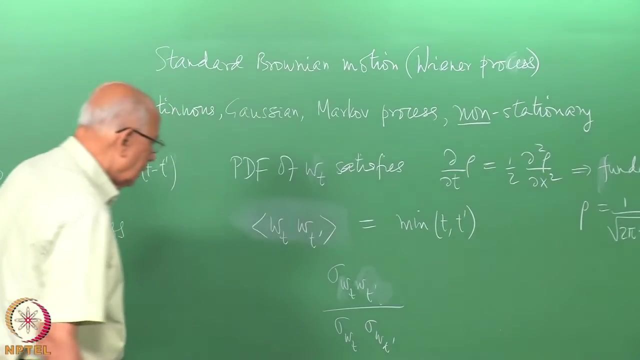 deviation of this and that, so as to normalise it. So if you write it as sigma x 1 plus sigma t, so how should I write this? Sigma W t, sigma W t prime, W t prime here over sigma W t, sigma W t prime, where this is the standard deviation of W t and that is of W. 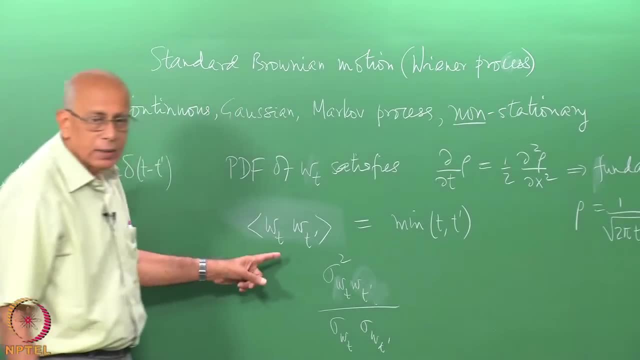 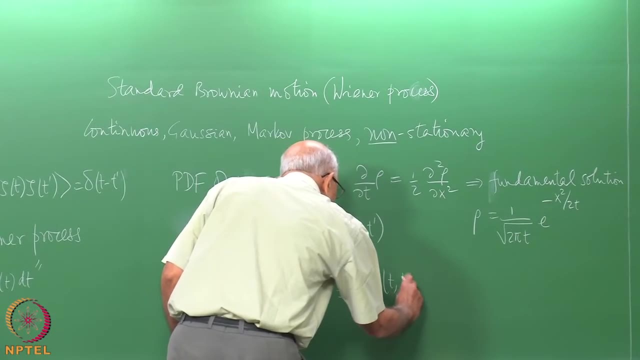 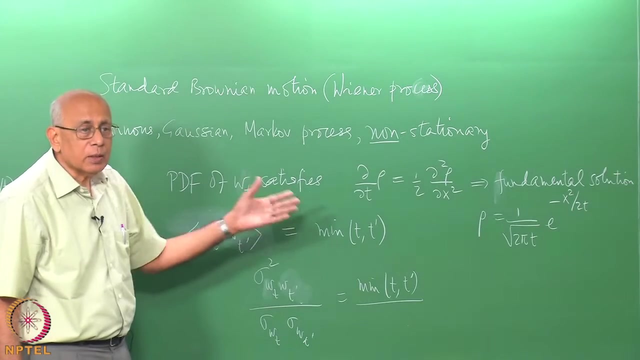 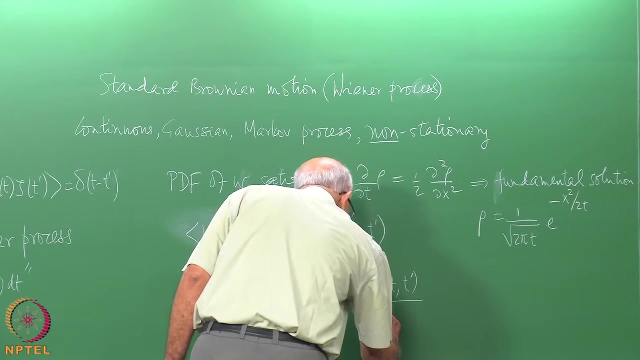 t prime. it should be sigma squared here. by definition, it is equal to this quantity. Then this is, of course, equal to min t t prime over. and we know what this is. the square of this is 2 d t, And this is not equal to 1, right, So this is equal to t. square root of: yeah, square root. 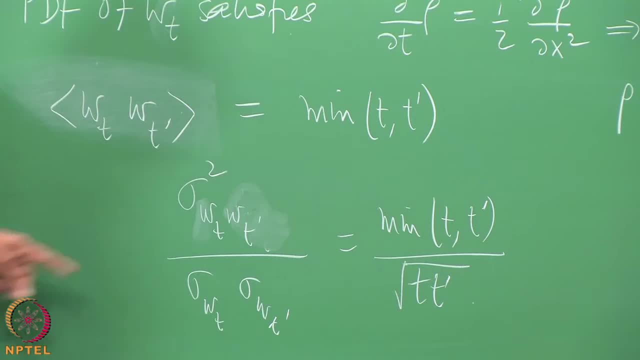 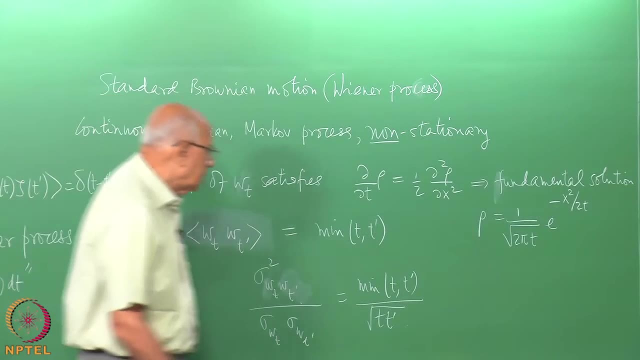 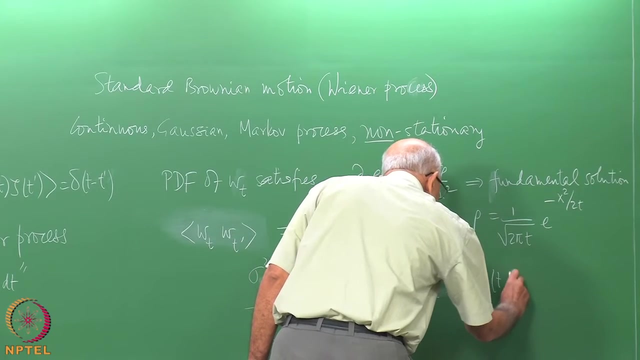 of t t prime. This is 2 d t and this is t prime and we are taking the standard deviation. so root of t t prime and it is easy to see that this is equal to min t t prime over max t t prime. the whole thing square root. That is a convenient way of writing, easy way of. 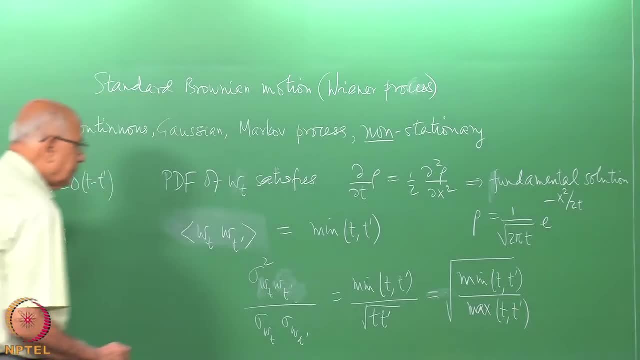 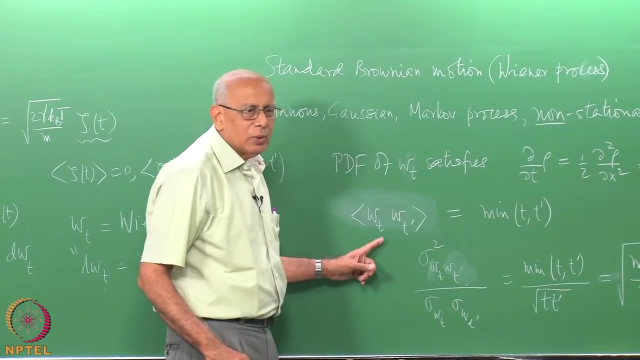 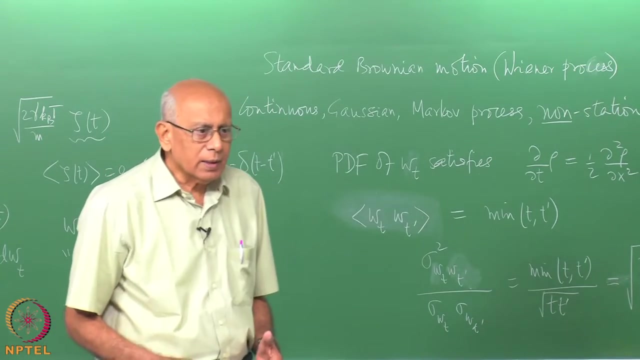 remembering this. Now, what can we say about the paths of this W? t? Ok, It is clear formally that the Brownian particle has got Brownian motion has infinite velocity. It is a very important part of the problem. Now, what can we say about the paths of this W? t? It is clear formally that the Brownian 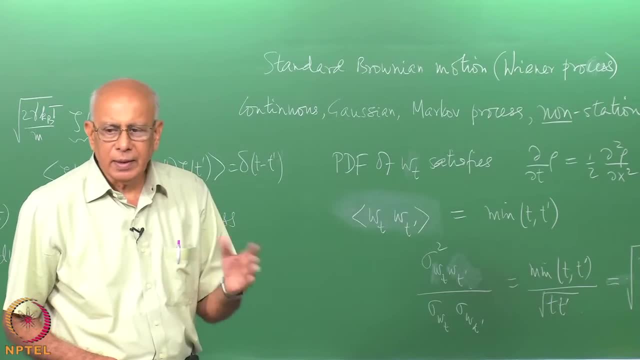 particle has got Brownian motion has infinite velocity. Now what can we say about the paths of this W? t? It is clear formally that the Brownian particle has got Brownian motion, has infinite velocity Because x square scales like t, not x, and therefore delta, x over delta. 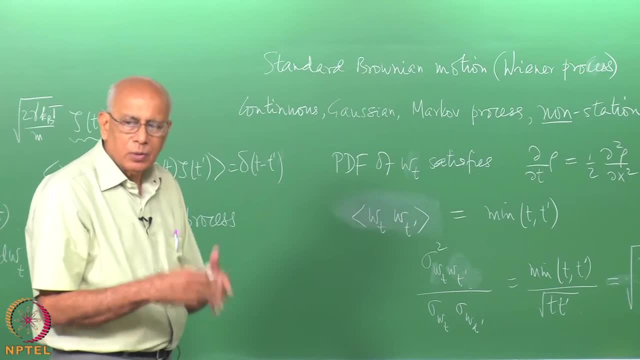 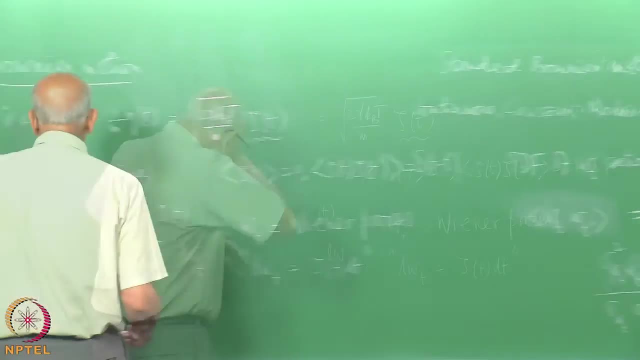 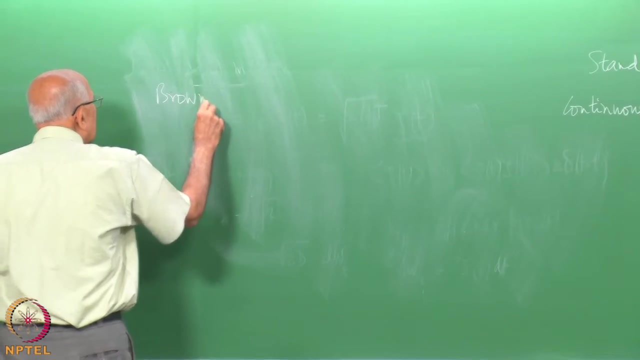 t is formally infinite, you need to put another delta x on top in order to bring it to a finite value, right, Ok? So what do these paths look like? That is worth looking at, and a number of results are known In one dimension. Brownian path or sample paths are known in one dimension. 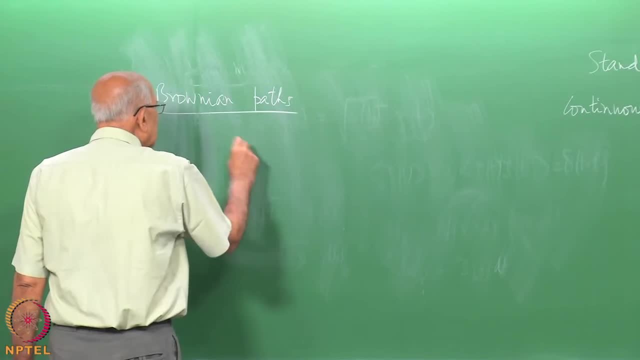 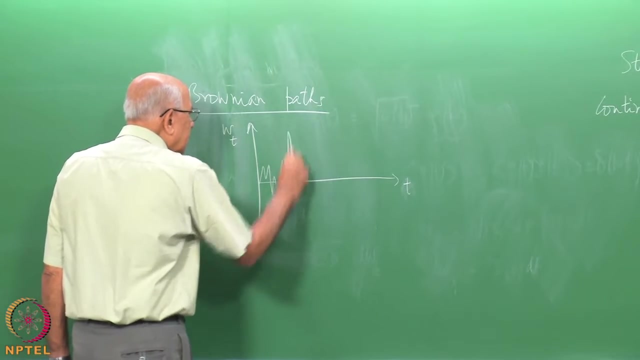 Sample paths of Brownian motion. we are talking about Brownian motion starting at the origin. So here is x and, sorry, here is t and W, t, the Wiener process starting here, and this process takes off and does this kind of crazy thing: it goes up and down, etc. And the following: 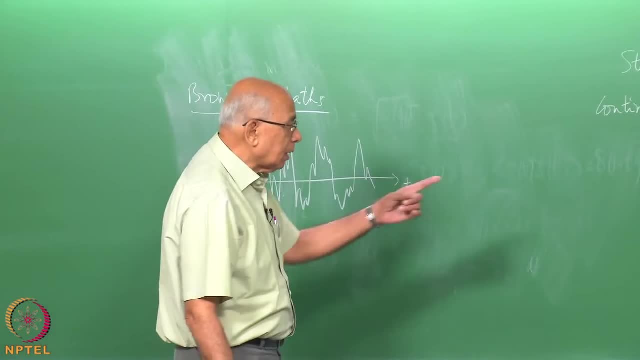 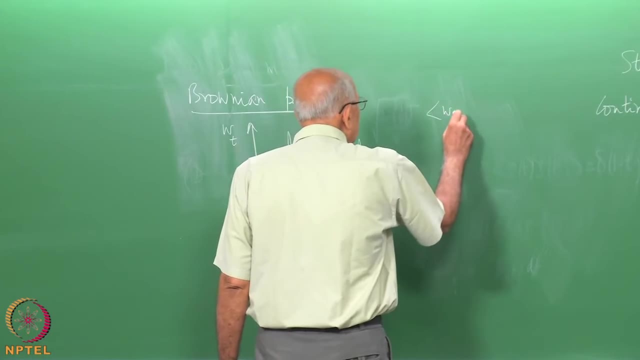 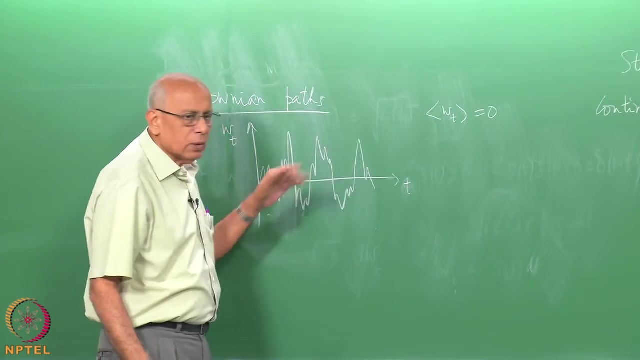 can be established rigorously from the properties of the Wiener process. Ok, The average is 0, we already know that. So over all such sample paths you take the average, it remains 0 here. Ok, But the question is: is it differentiable or not? Is this differentiable? 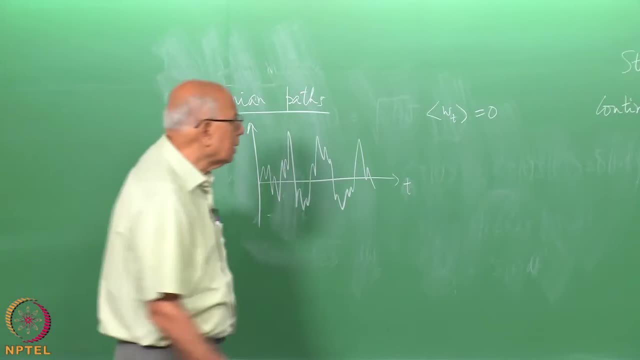 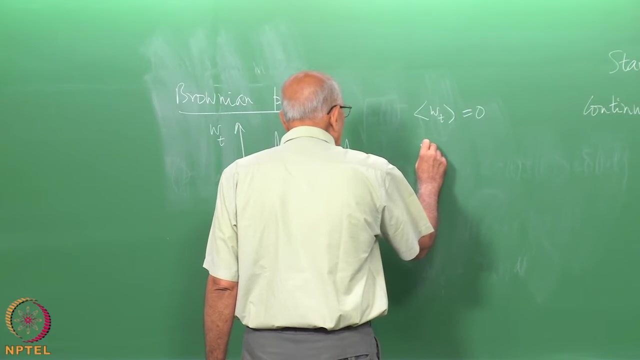 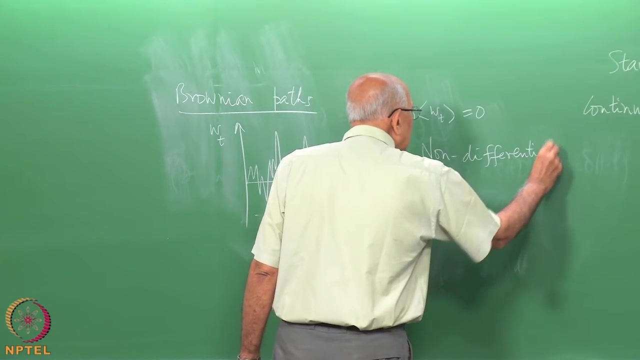 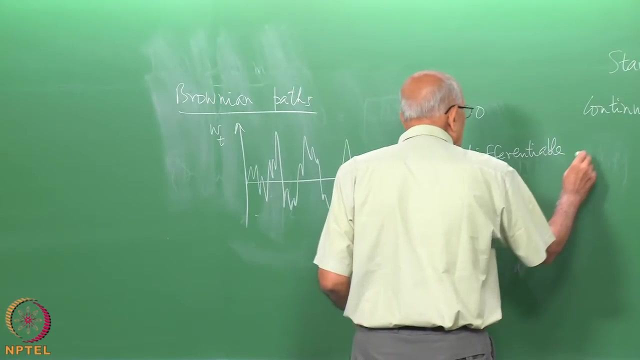 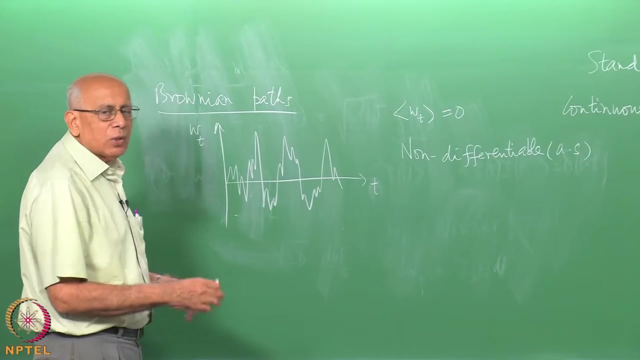 And the answer is no. I will just quote a number of results here. So nowhere differentiable, almost surely So non-differentiable, Except on sets of measure 0, non-differentiable, almost surely. How badly is it non-differentiable? 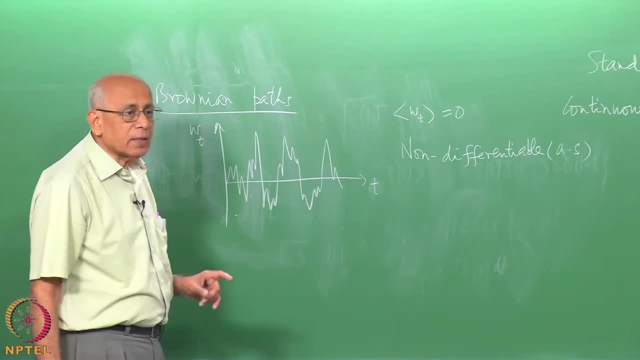 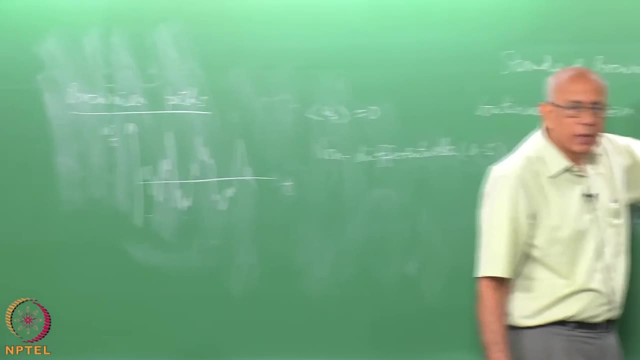 And there is an answer to that. It is a continuous process and that is very, very important to remember. Uh, So had we dropped this and had we required it to be stationary, what would the process be? Pardon me On Steyn-Nolenbeck. 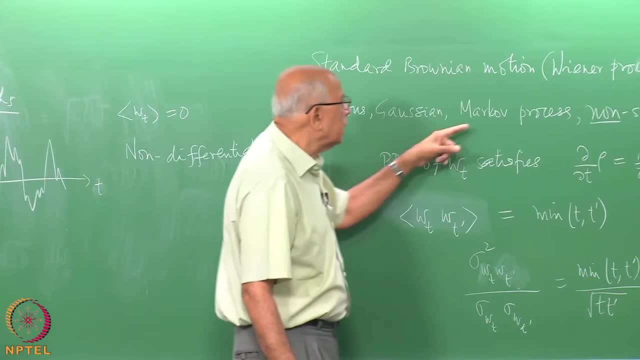 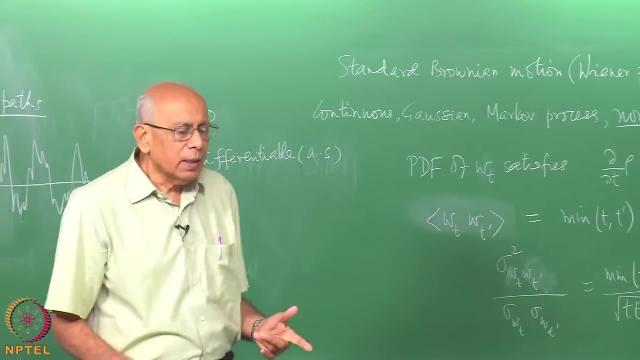 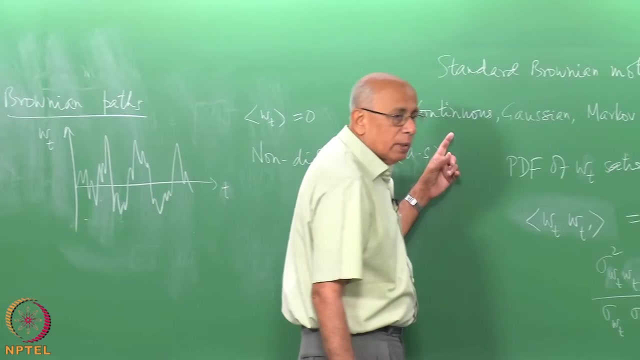 On Steyn-Nolenbeck. That is the only continuous Gaussian stationary Markov process And it follows that it has an exponential correlation, and vice versa. the converse is also true in that case. But the moment you make it non-stationary but require it to be continuous, then you will. 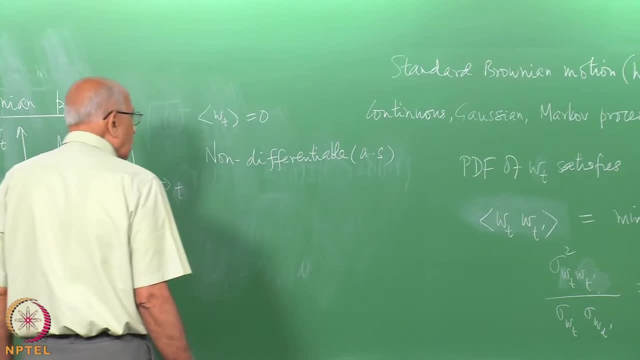 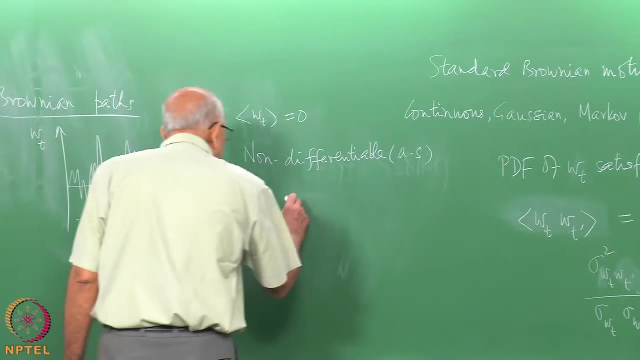 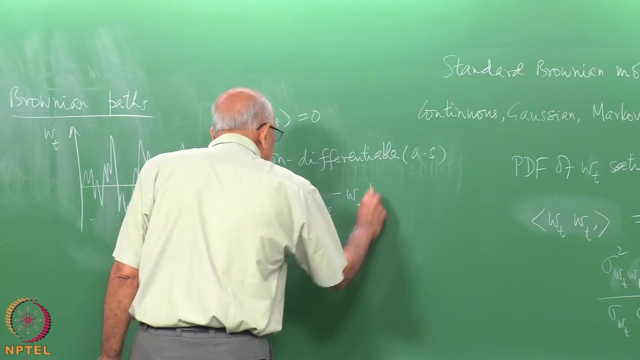 end up with Brownian motion. Ok, It is non-differentiable, but it is continuous. therefore there must be some kind of Holder continuity for this process. Now it turns out that the continuity looks like this: W of t plus epsilon minus W, t modulus is less than or equal to some. 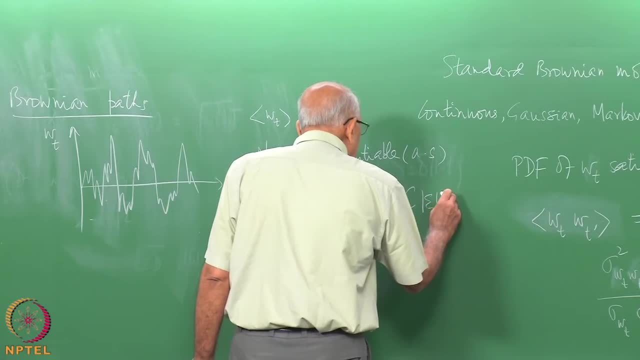 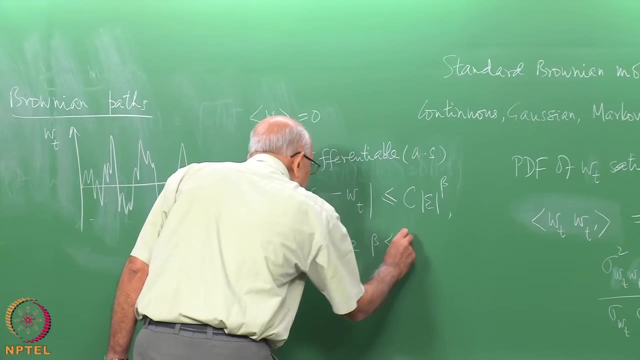 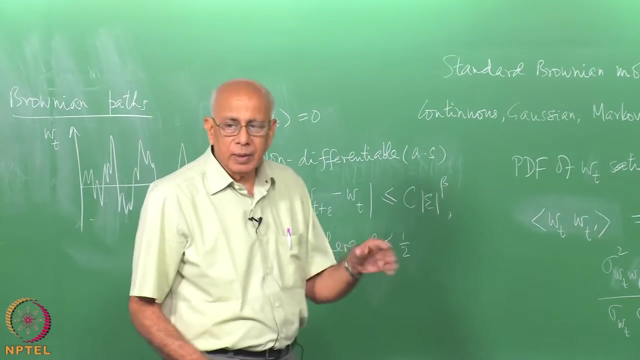 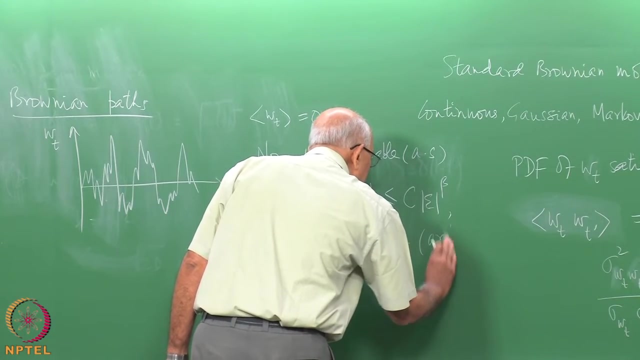 constant times: epsilon mod: epsilon to the power beta, Where beta is less than half but can be arbitrarily close to half and not half, except on sets of measure zero Arbitrarily Close to half from below. So this is a non-differentiable. 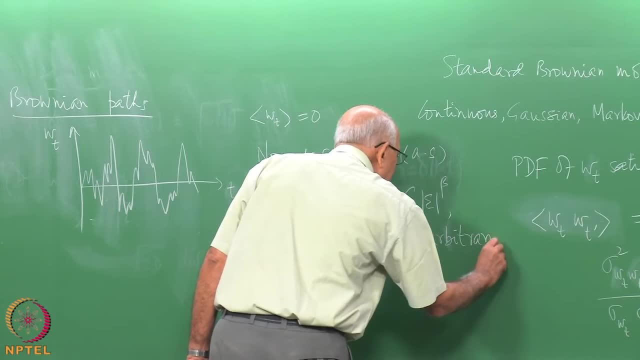 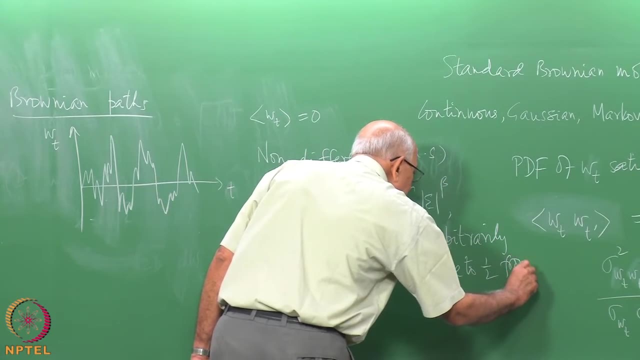 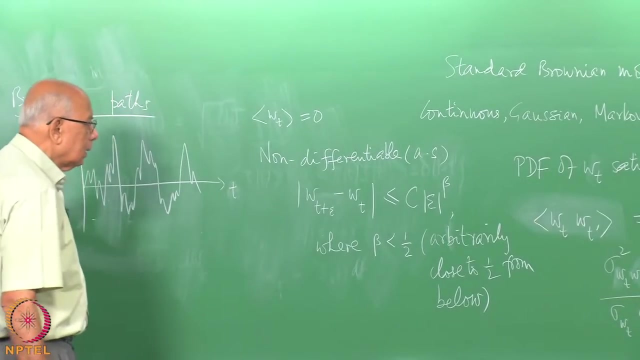 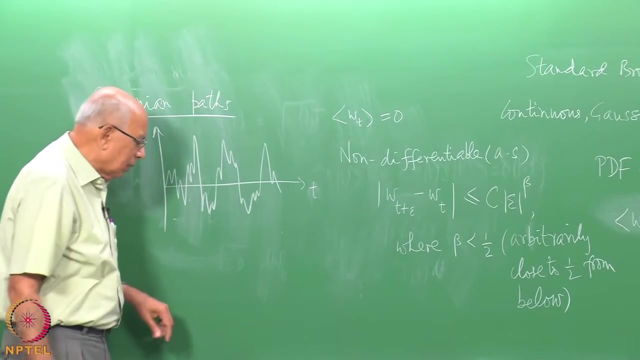 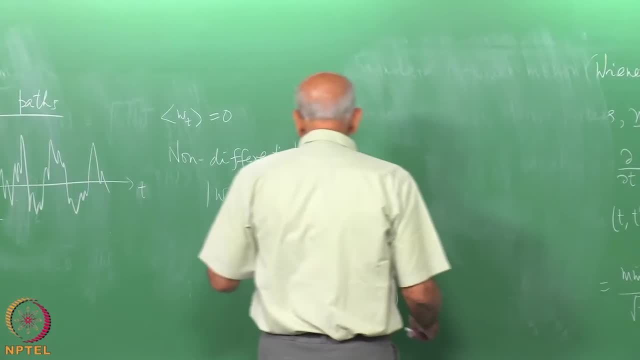 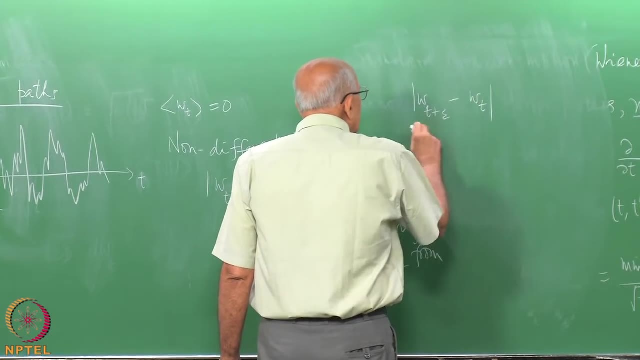 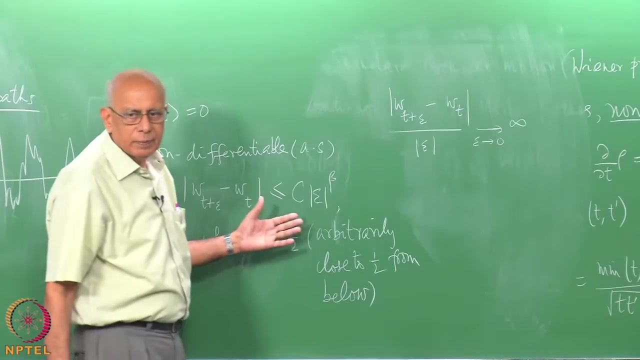 for differentiability. yeah, if you divide by epsilon, so it is clear that W t plus epsilon, Uh minus W t divided by moderate, Uh minus W t divided by mod, epsilon tends, as epsilon tends, to zero, it tends to infinity. because of this property It is going like half. so you divide here you are going to get 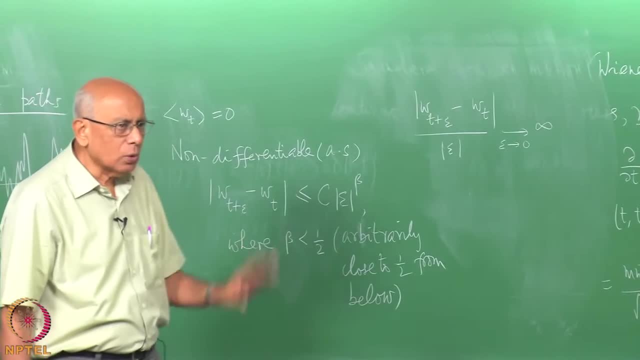 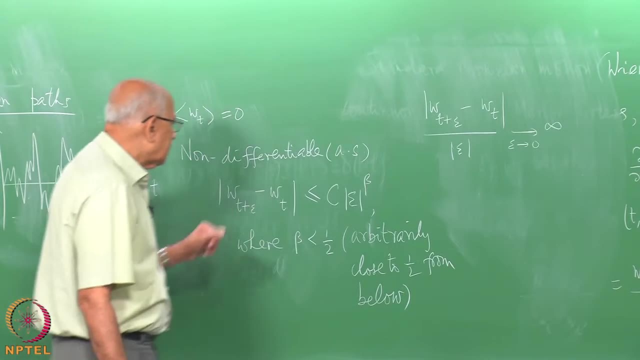 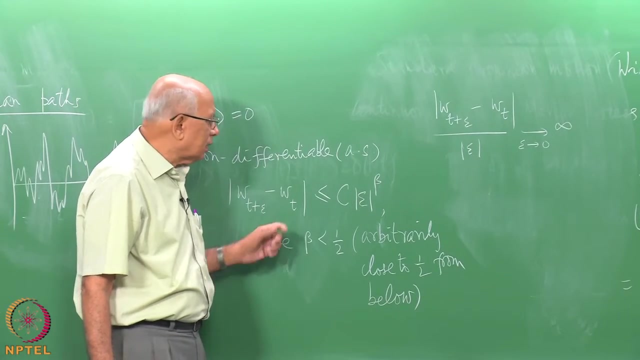 a half, little more than half in the denominator and it is going to go to infinity as epsilon goes to zero. So it is therefore not differentiable. But this weirdness that it is holder continuous with an exponent which is arbitrarily close to half from below means that this increments. 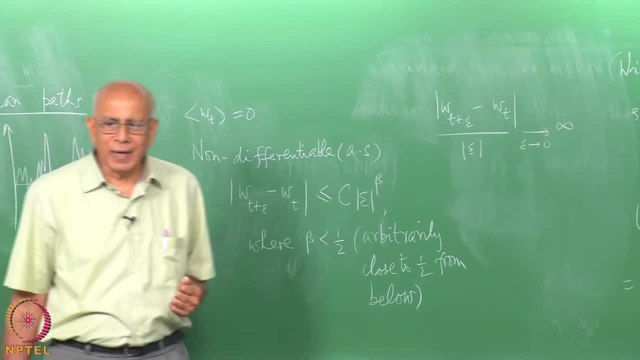 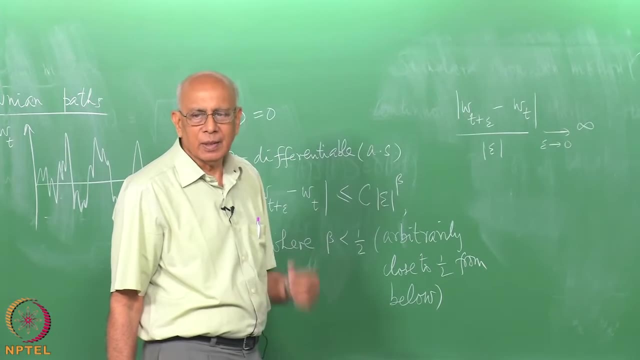 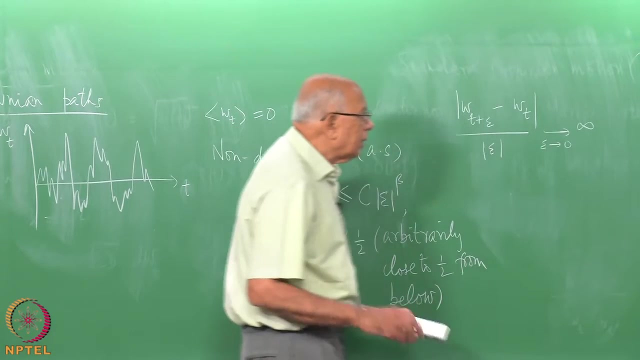 in this process are acting somewhat like square root of time. This epsilon is like the increment in time, right, So it is acting like the square root of d t, the infinitesimal d t. One can formalize that and then you have to be a little careful. but by a clever amendment of the rules, 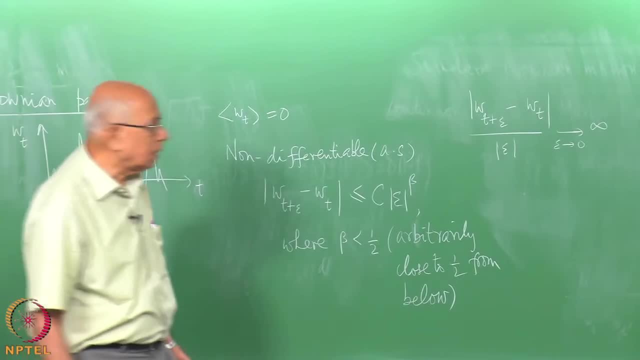 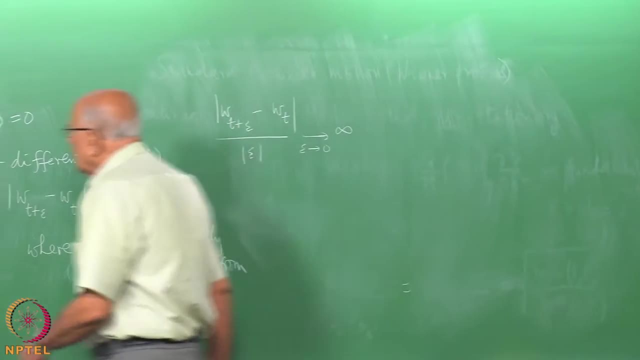 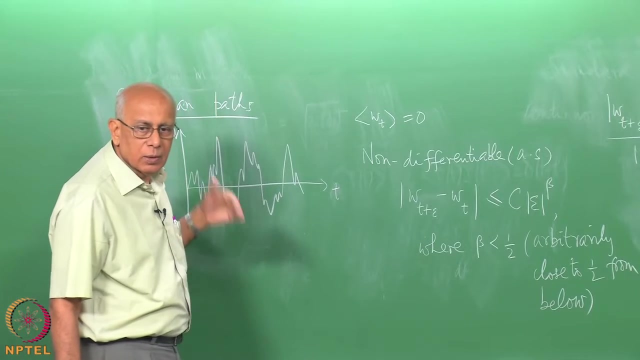 of calculus, one can actually handle this process quite rigorously. Here is what happens. Or to continue on the sample, another property of the sample path, you can ask: when does it cross zero in a given time interval, how long does it stay above the axis and how long? 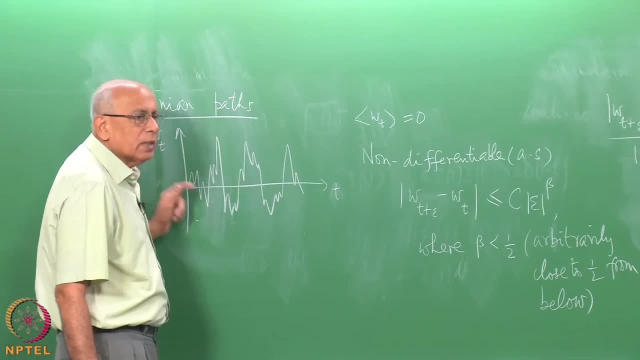 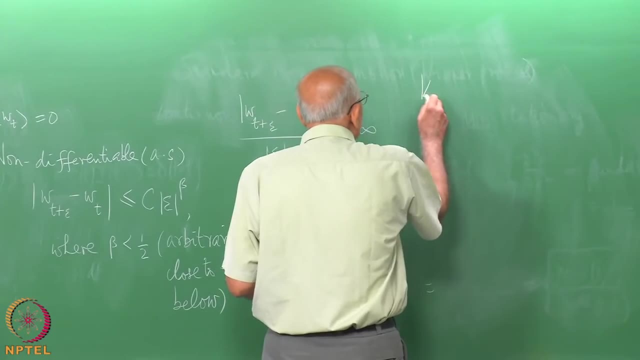 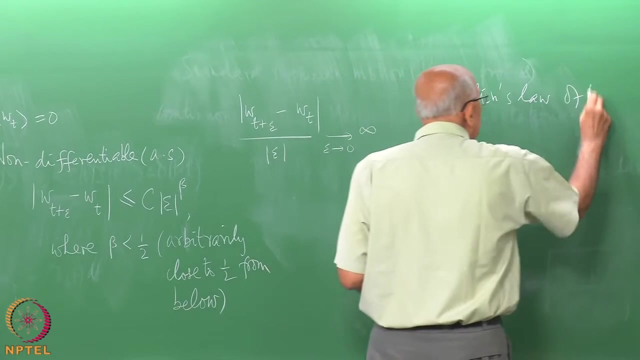 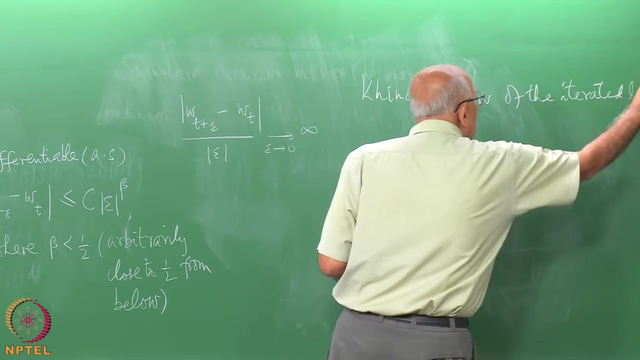 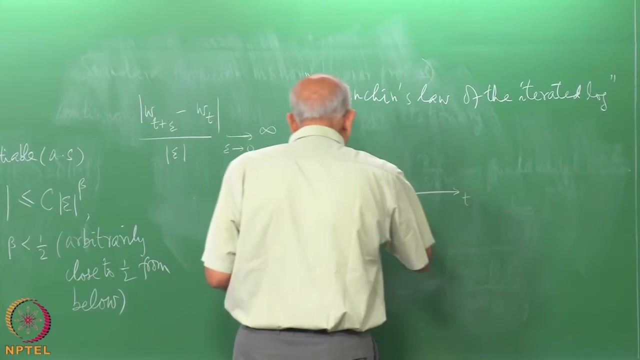 below on the average, and so on. In fact, you can ask where is this particle going to be most of the time? and it turns out there is a law of the iterated logarithm. This is Kinchin's law. Ok, So you plot for Brownian motion starting at t equal to zero. you plot the following: 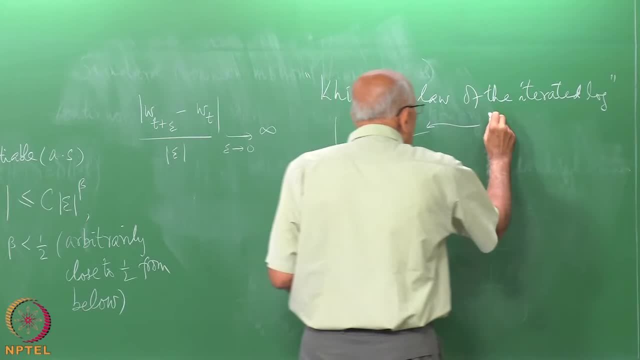 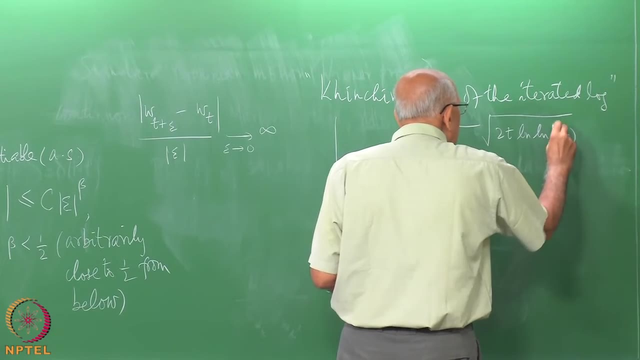 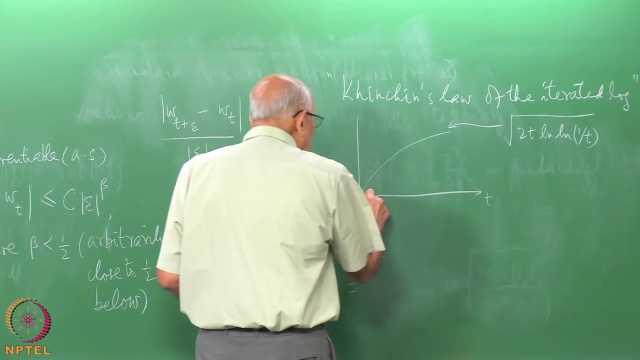 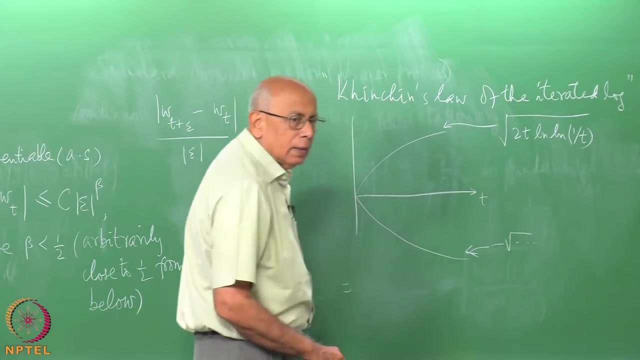 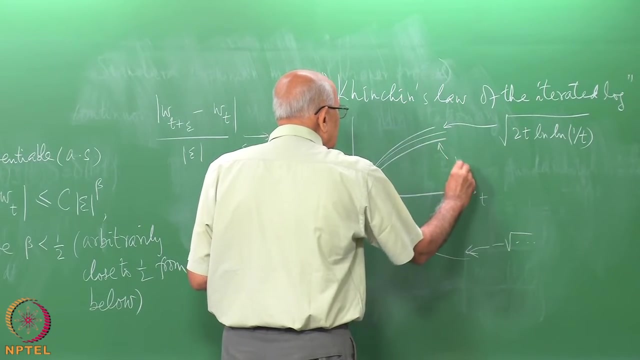 function. This function is square root of 2 d t log log 1 over t for small t, sufficiently small t. Plot this Ok, And you plot the negative of this function. This is minus the square root of this stuff And if this is 1 plus epsilon times that function, and that is 1 minus epsilon times that function. 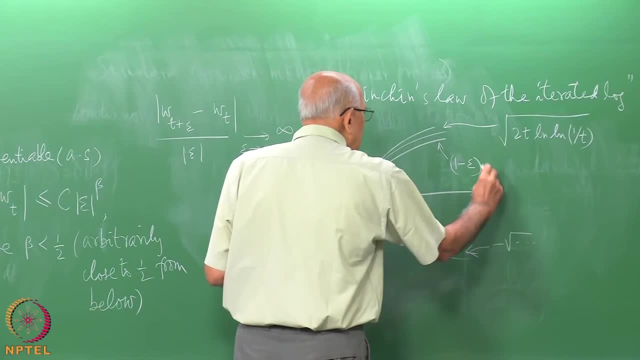 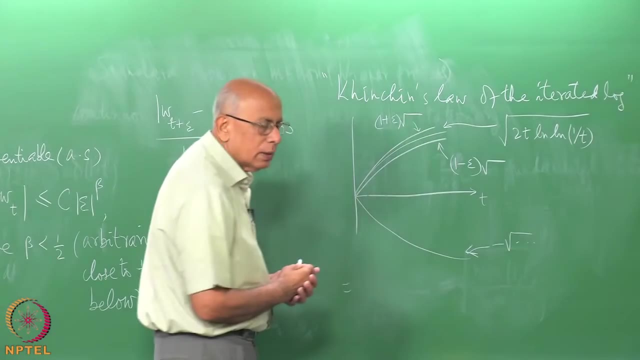 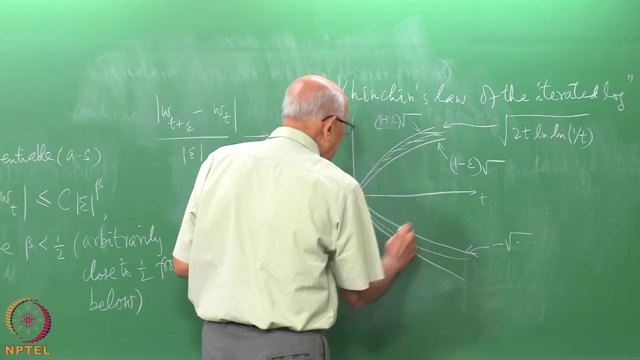 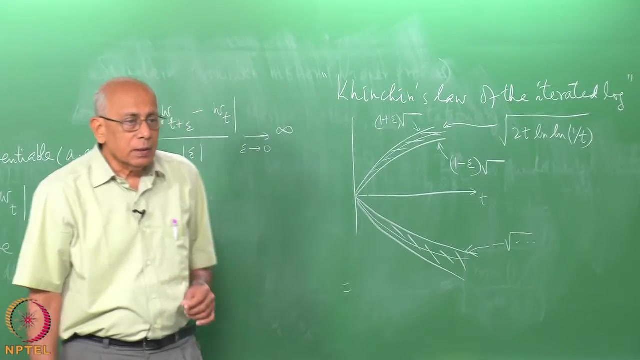 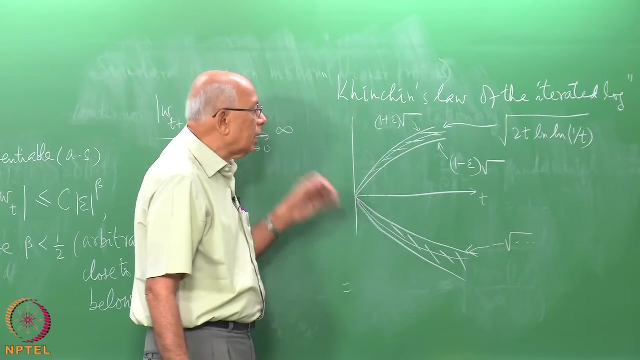 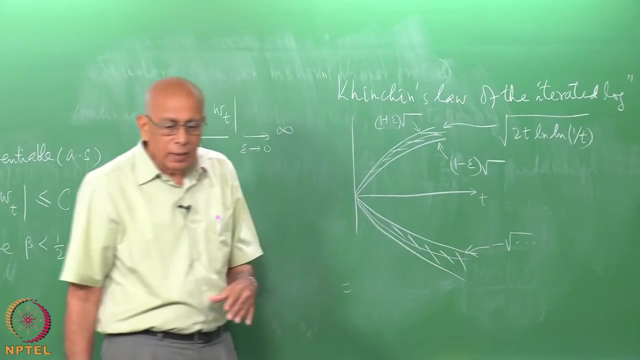 so this is 1 times square root and this fellow is 1 plus epsilon times the square root, And similarly here: Ok, Then the statement is: almost surely the particle is either here or here in this range for arbitrarily small epsilon. Ok, So you not only have a statement about the probability density function. 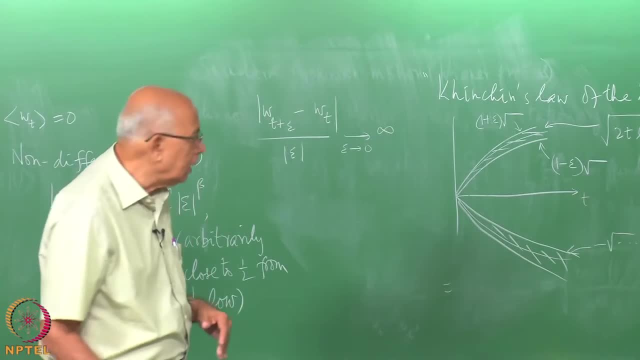 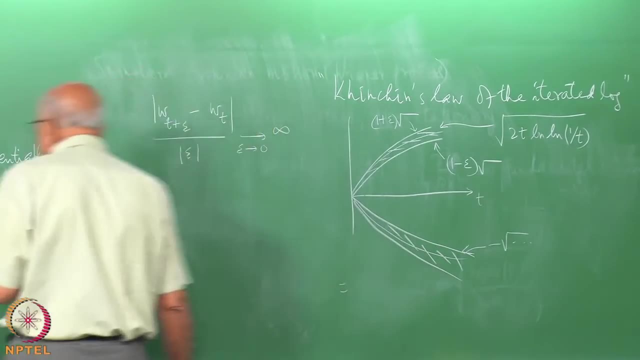 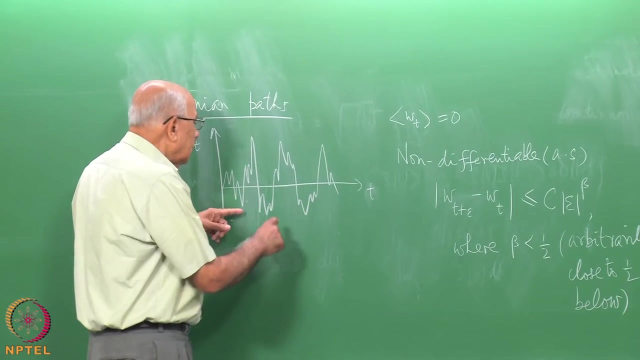 of this, x as a function of t or w as a function of t, but you also have a statement about where it actually is what this part does. and yet, and yet. the particle crosses the axis an infinite number of times. It does so in any arbitrarily small interval, and you can. 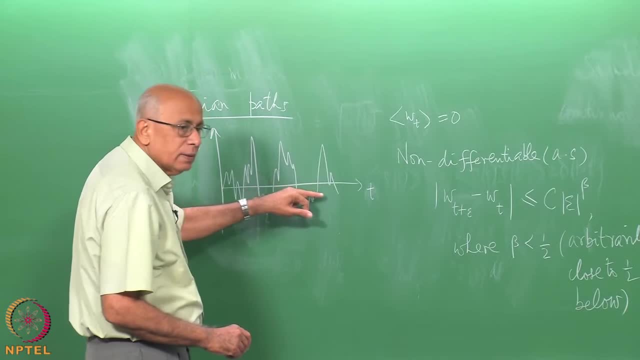 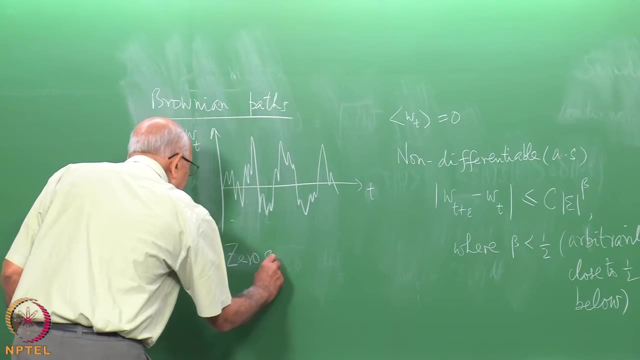 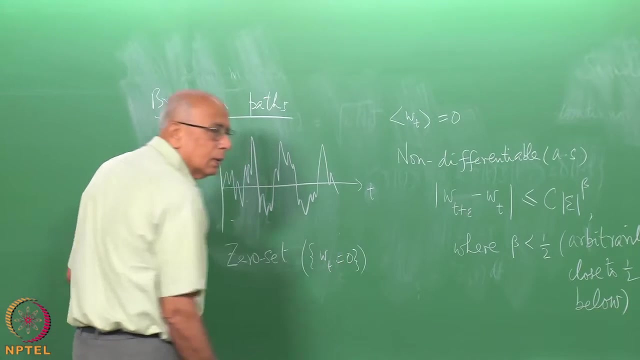 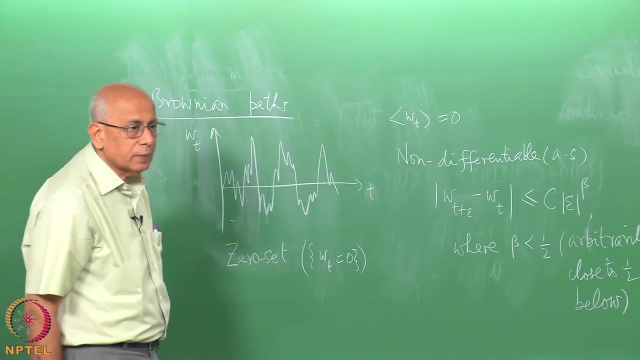 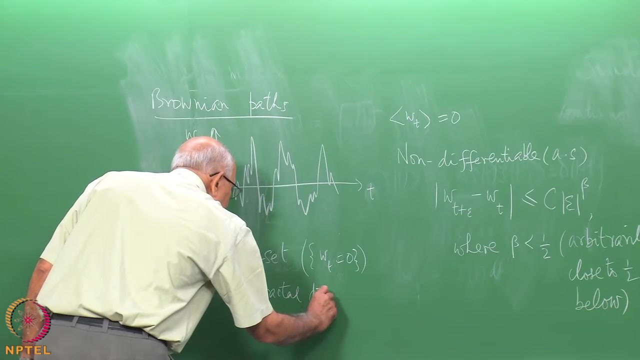 in fact ask: what is the measure of the zero set? the set of points where it crosses the axis. So zero set, This would correspond to the set where w t equal to zero. Ok, That zero set in the limit has a fractal dimension which is a half. 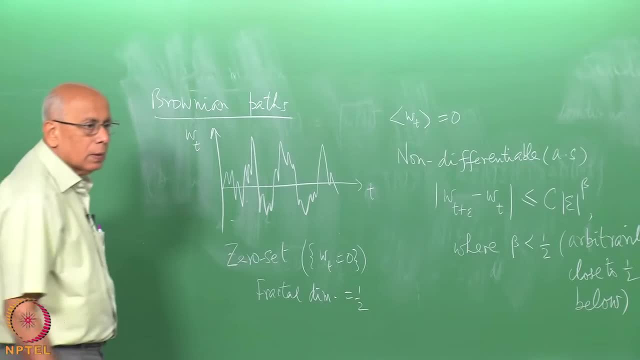 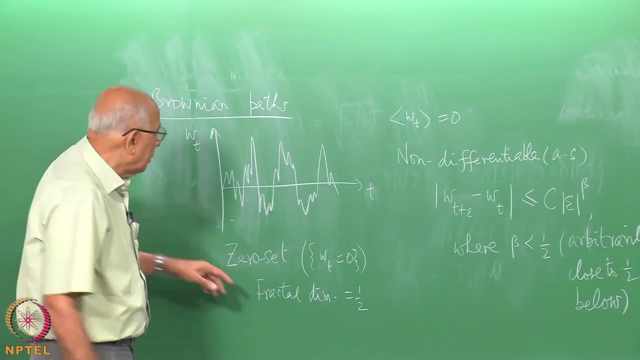 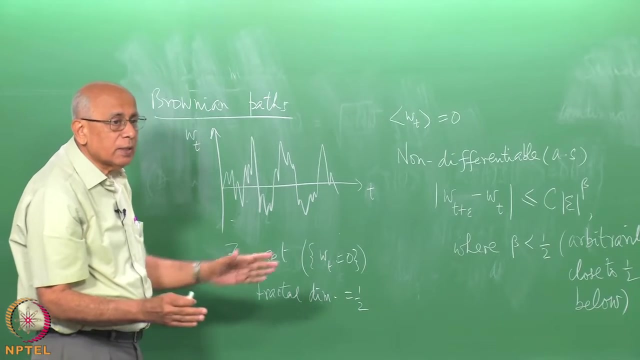 Ok, So while it can go arbitrarily far away, the zero set is such that, by the way, this thing, the fluctuations, obviously they are going to go way up there, way down here, and that is why the variance itself will increase with t, because the fluctuations are such that 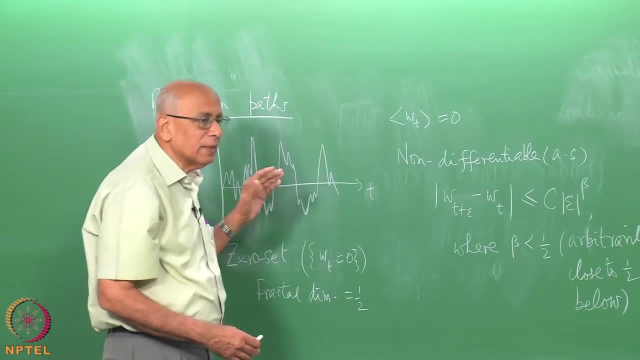 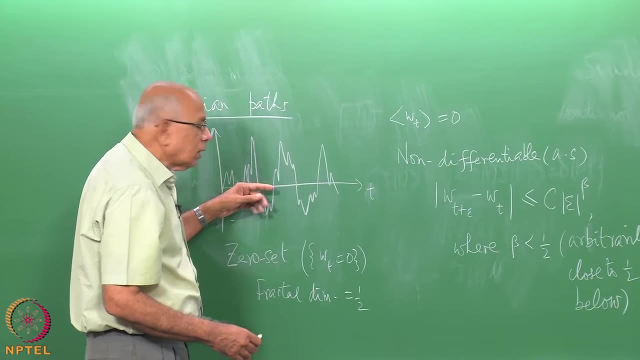 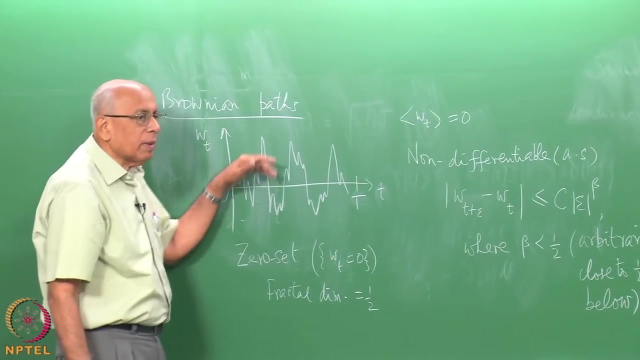 it is getting. it is diffusing, although the mean remains zero always. You can ask further interesting questions. You can ask: what is the given given some t here? what is the fraction of time for some some capital T starting at zero? what is the fraction of time that it spends above the? 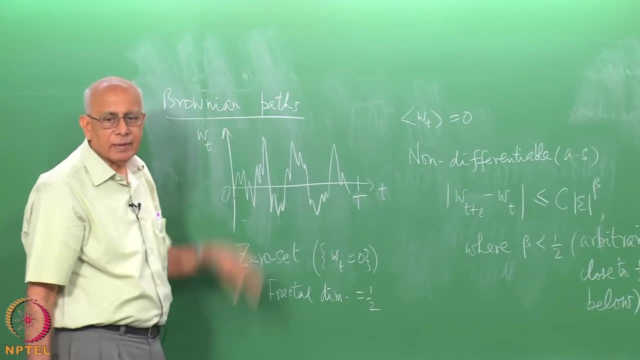 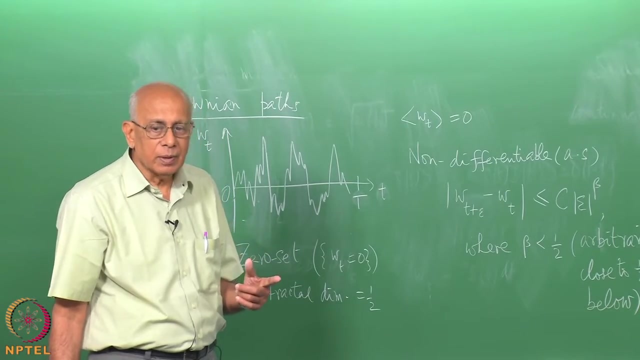 real axis above the on the positive side and what is the fraction it spends on the negative side? That is a random variable. It should be equal. right, It is yes, but it is a random variable. Yes, Ok, One can ask what is the probability distribution of that random variable? So let's suppose 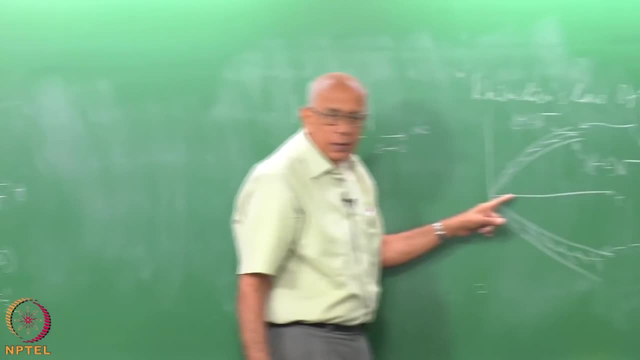 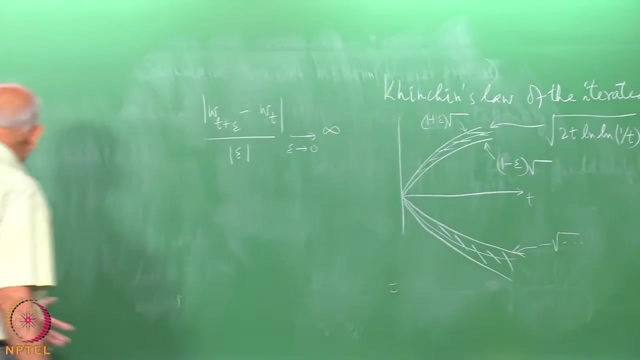 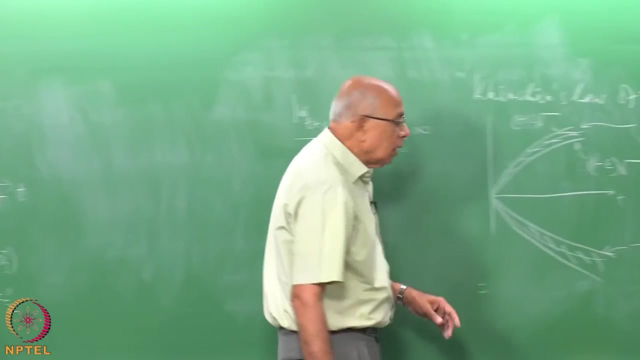 so I am being incoherent. You could ask: what if t is very large? You have a law of iterated logarithm for t large as well. All you have to do is to replace that log log 1 over t by t. Ok, But the crucial point is not that. The crucial point is this process is reinventing. 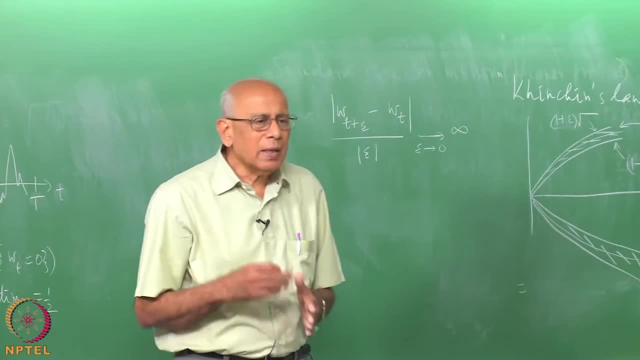 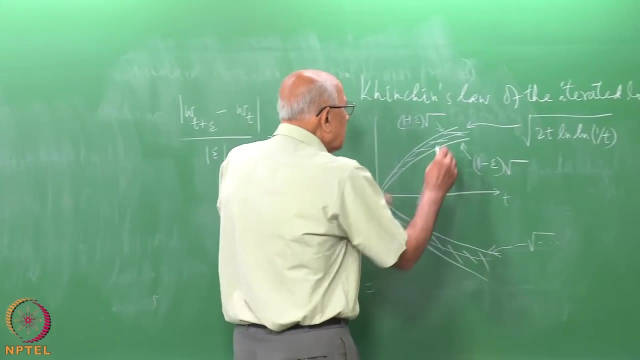 itself at every instant, Ok, Ok, At every instant of time. It is what is called a martingale. I am not going to talk much about that, but we will see some consequences of what it does. It means that if you are 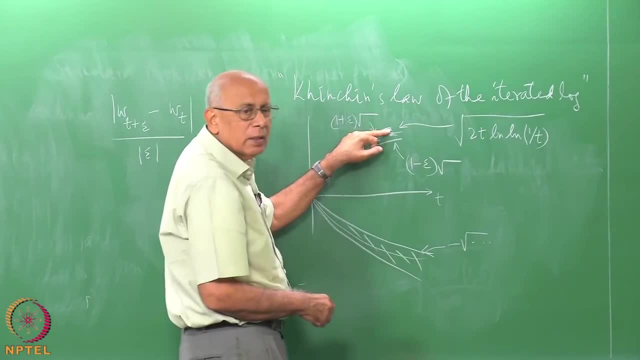 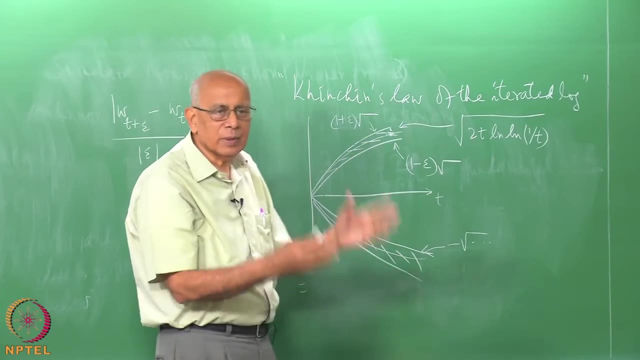 here at this point, say you are here at that some instant of time, then the Brownian motion is as if it starts from there at this instant of time, and it again behaves in precisely the same fashion as it behaved earlier here. So at every point there is a law of the iterated. 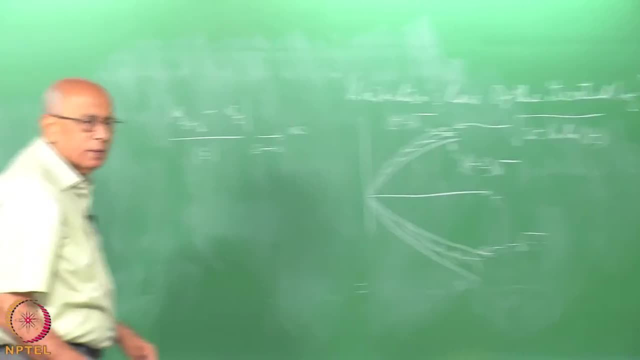 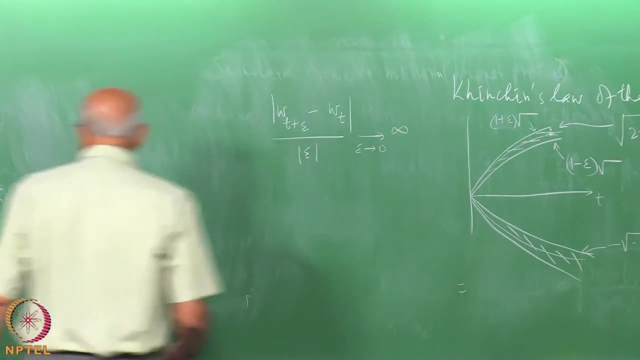 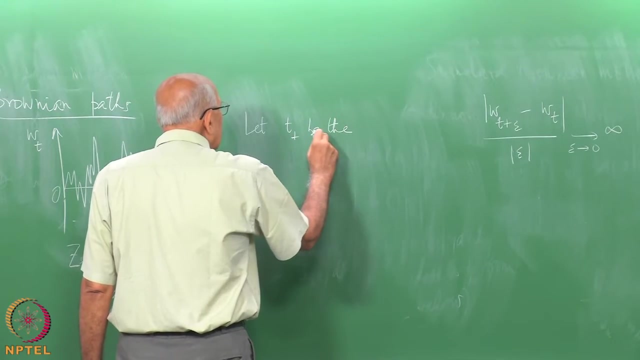 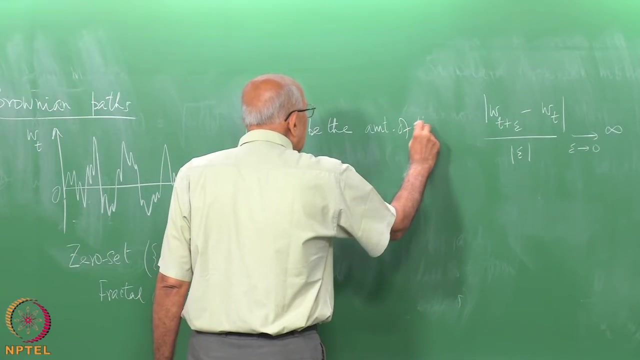 logarithm at every time. Ok, This is the memory is very short, It is a Markov process. Ok, Now one can ask the probability distribution function. So let t plus be the, be the amount of time, such that w t is greater. 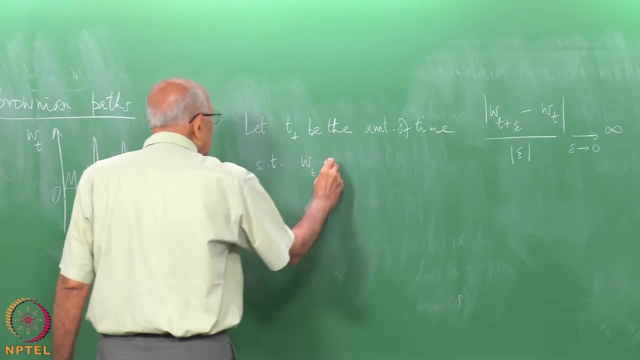 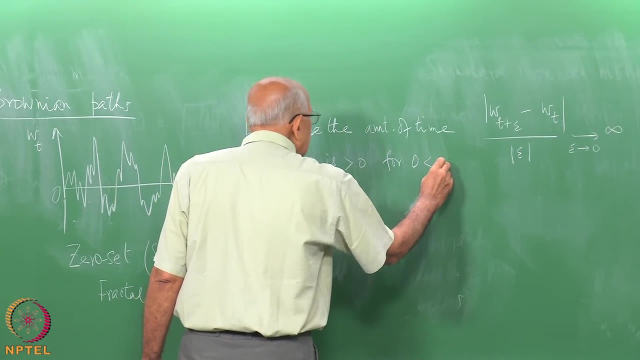 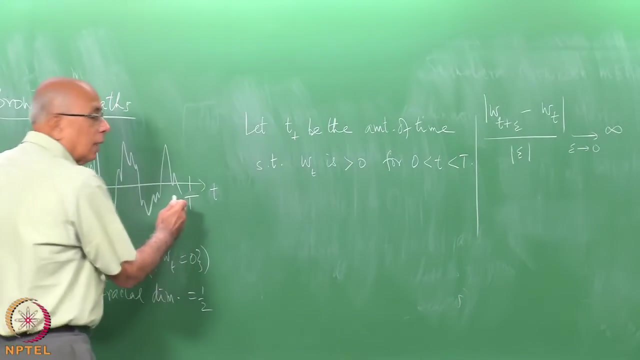 than or equal to t plus Ok, Ok. Ok. So w t is greater than zero for zero, less than t, less than capital T. Ok. So we look at the Brownian motion up to some capital T and ask: what is the total time spent where? 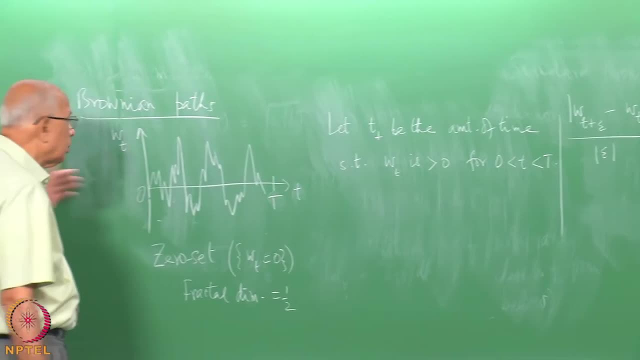 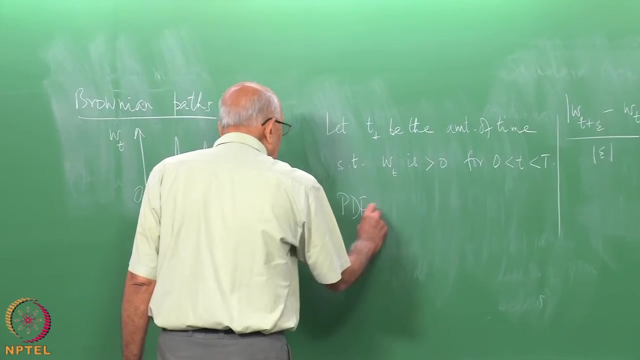 it is on the positive side and what is the total time spent where it is on the negative side of the x axis? The PDF of the x axis, Ok, The PDF of t plus and, similarly, as you say, t minus, it is completely symmetric. PDF of. 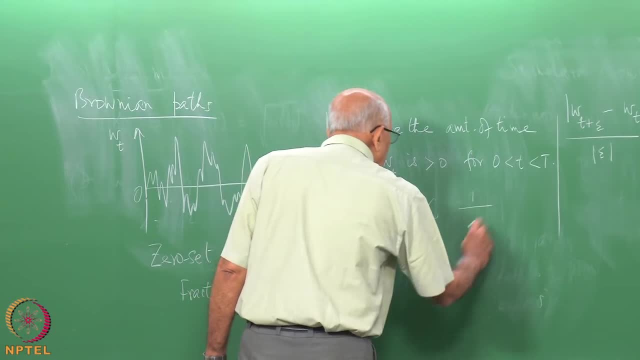 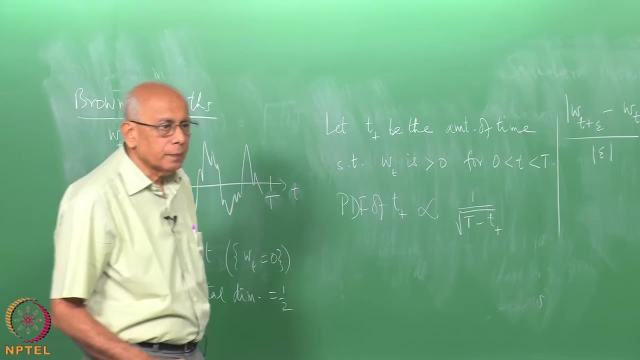 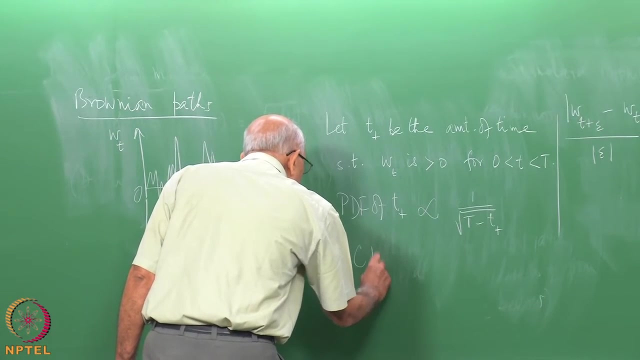 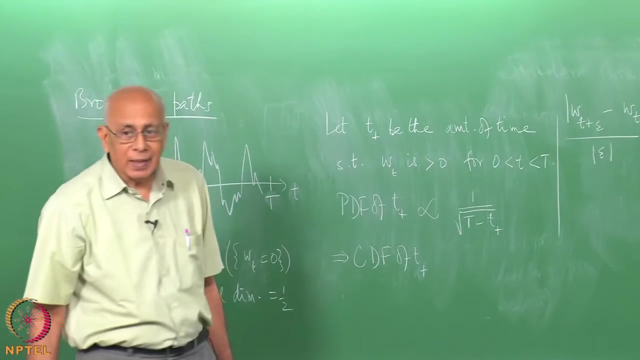 t plus is proportional to 1 over square root of t minus t plus. Ok, Which implies that the cumulative distribution function C, Df of t plus. It looks like the oscillator. Yes, It looks very much like the oscillator. yeah, the time instead of if you have a regular. 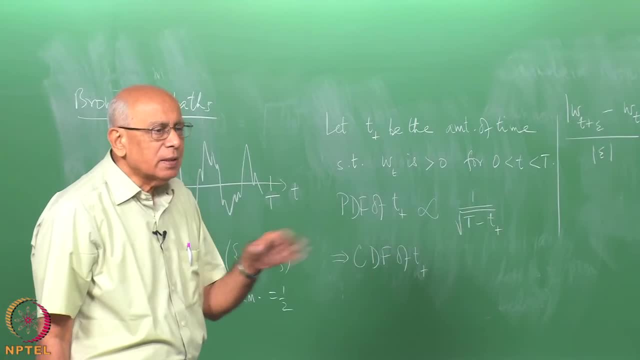 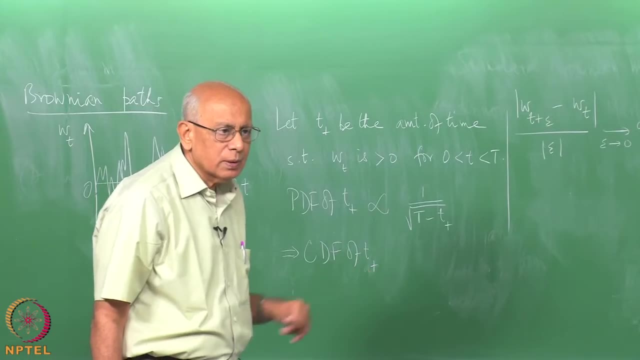 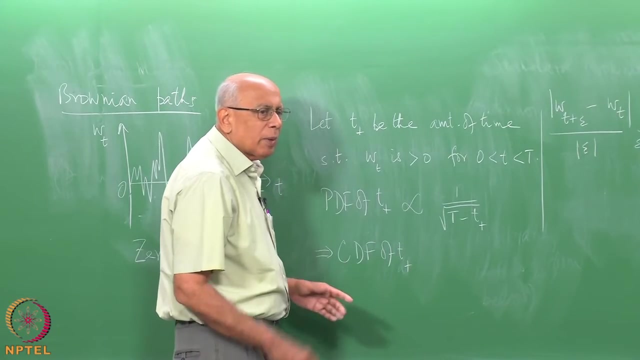 oscillator and you ask: dt t is distributed uniformly over a period. you ask: what is the distribution of the angle? it is precisely this: 1 over square root. here, many such distributions. Now the cumulative distribution function, namely the probability that t plus is less than equal. 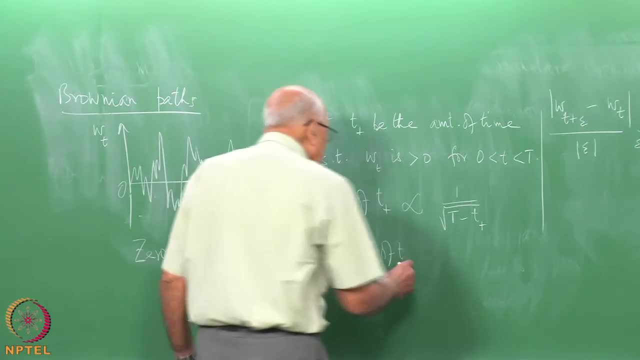 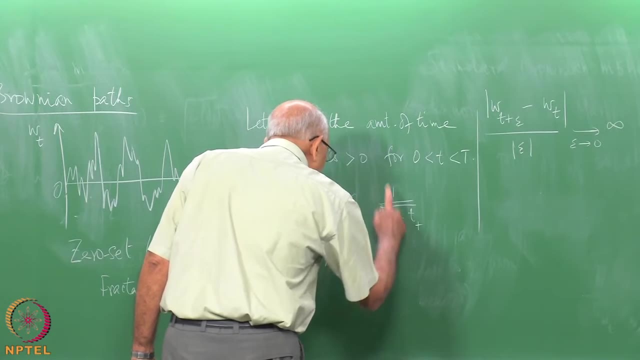 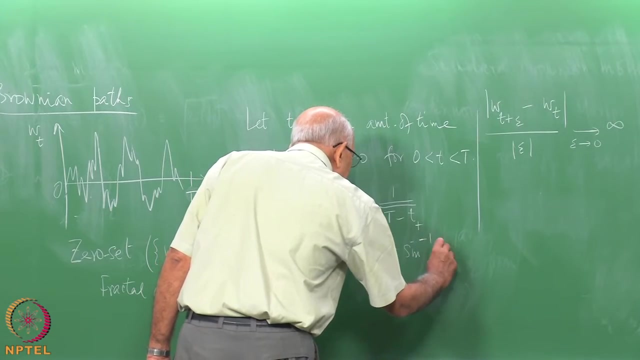 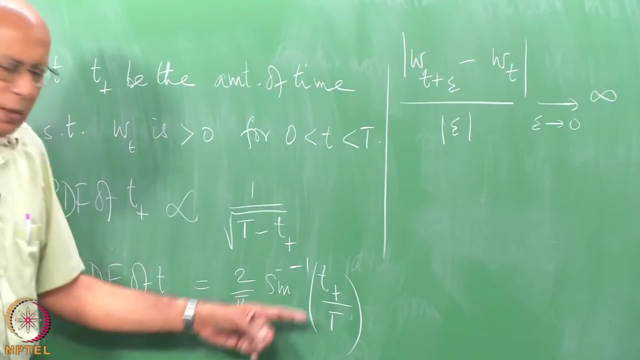 to some given value t f. this thing here of course now is equal to: if you normalise it and you integrate this fellow to 0 to t plus, you get 2 over pi sine inverse t plus over t. It should of course be 0 when t plus is 0 and it should be plus 1 when t is t plus. 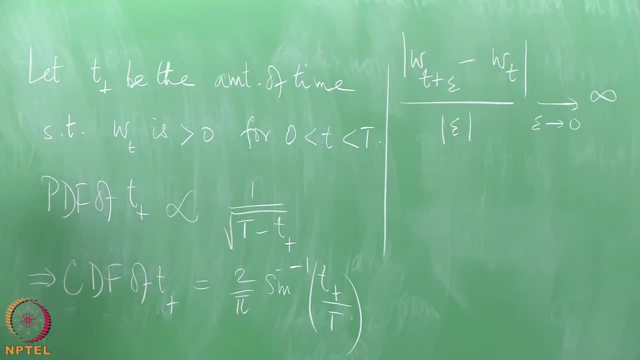 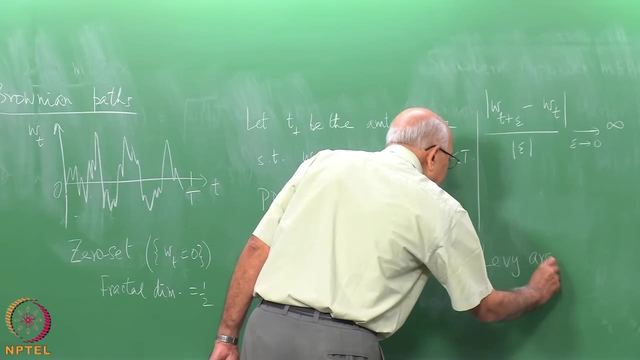 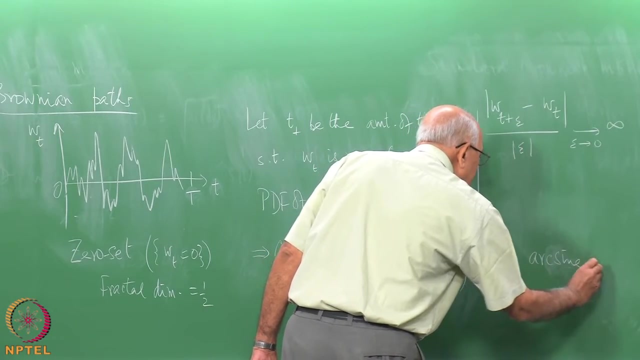 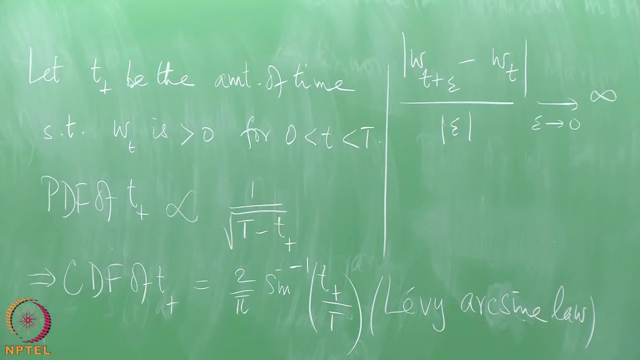 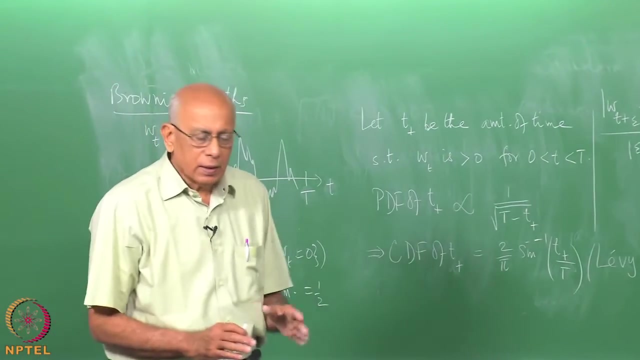 equal to capital, U, Total, t. Okay, Probability must be equal to 1, right, This is called the Levy arc sine law. okay, Now let us see what the fact that this, The fact that these sample parts are irregular, very jagged, they have very specific kind. 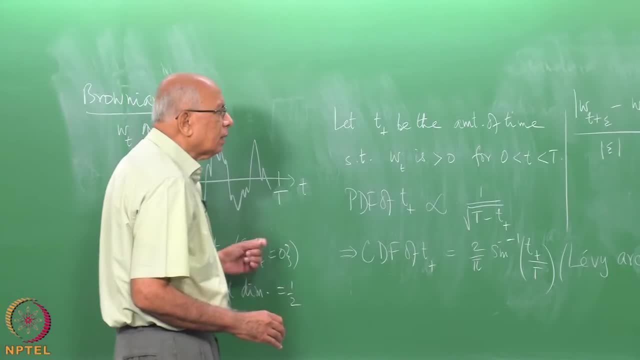 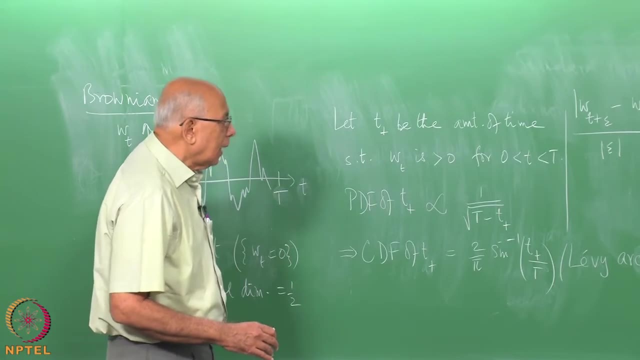 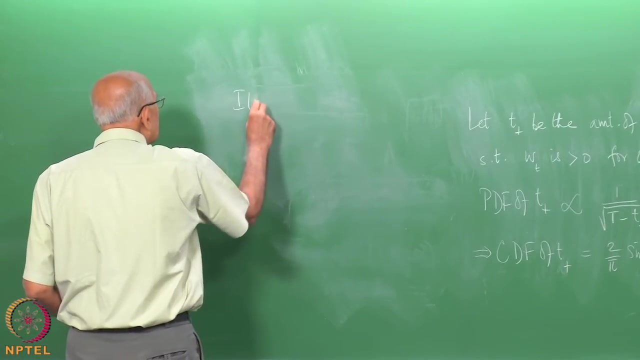 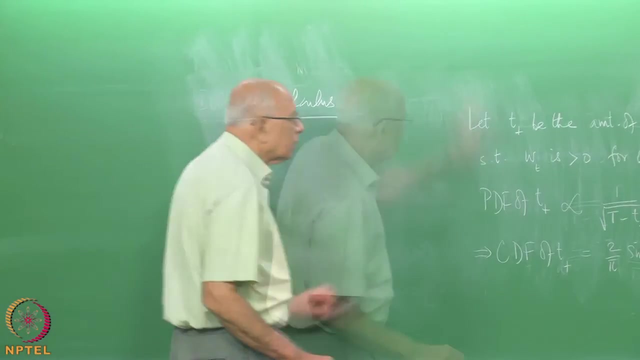 of irregularity essentially characterised by the fact that the the Holder continuity is half, essentially half. That says that the following property can be rigorously proved, and this is part of what is called Ito calculus, And I will mention only the rudiments of it: 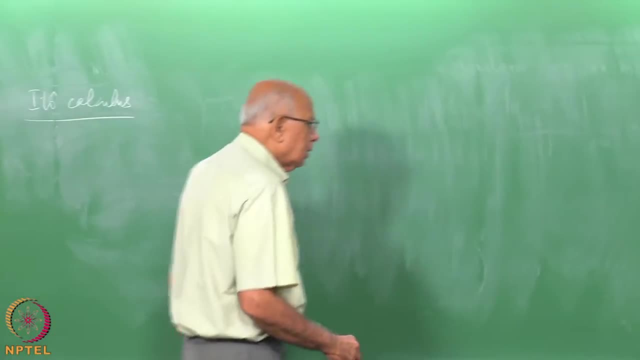 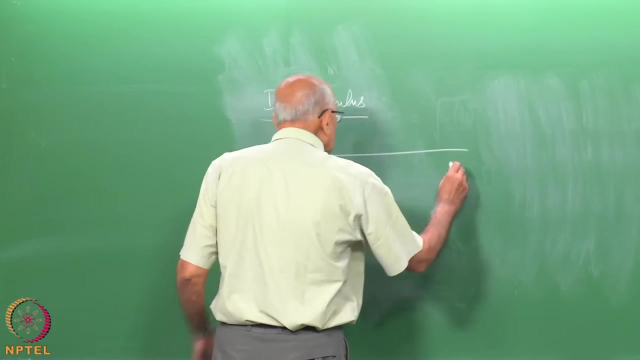 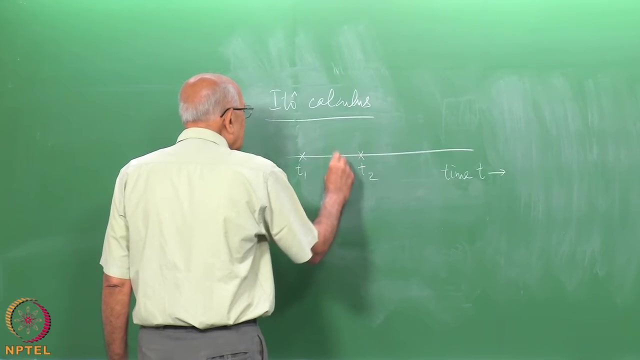 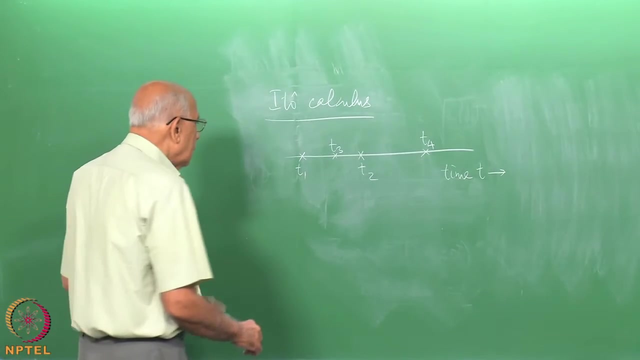 of it, essentially one formula, and it is the following: What one can prove what one can prove is that for Brownian motion or a Wiener process, if you have on the time axis any four points, so let us start with t1, some point t2, and then some maybe t3 and some t4. 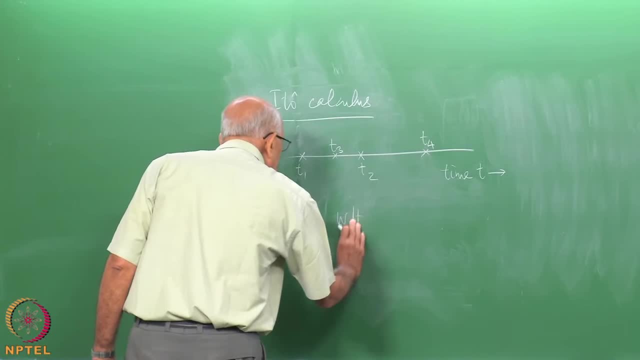 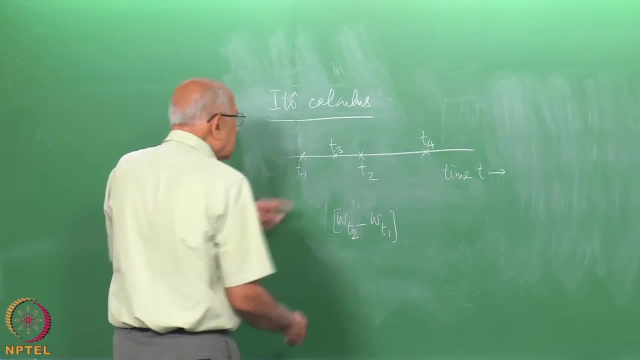 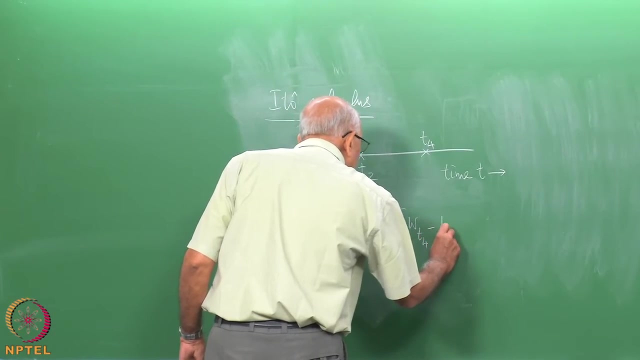 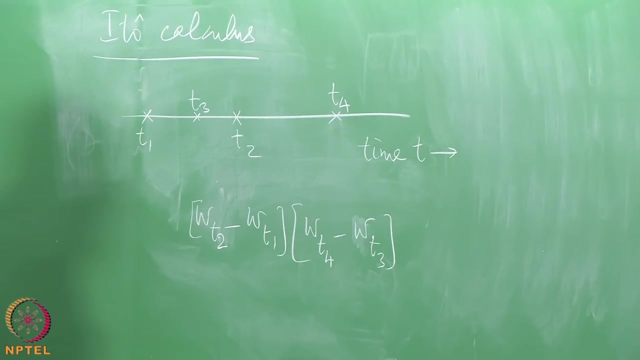 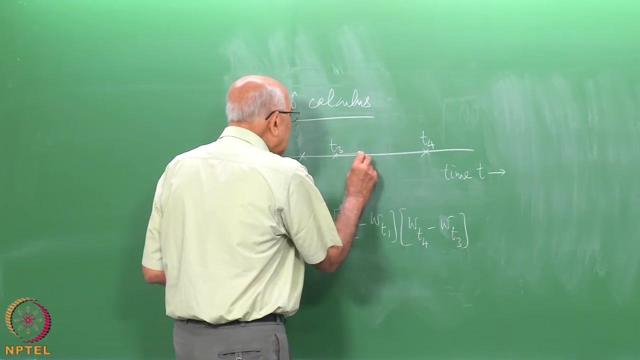 and you ask: what is this quantity W of W t2 minus W t1, so this minus that. and you multiply it by W t4 minus t2.. So W t3 is this thing here. the value of this product here is equal to the overlap between: 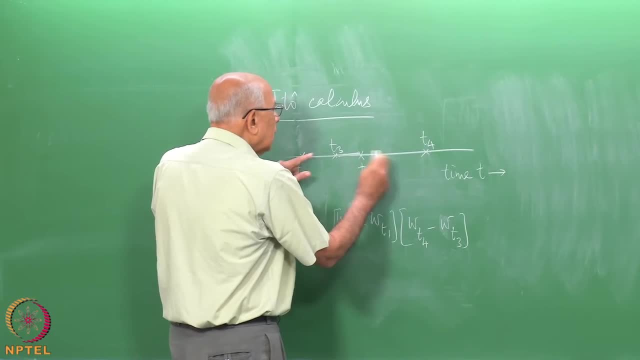 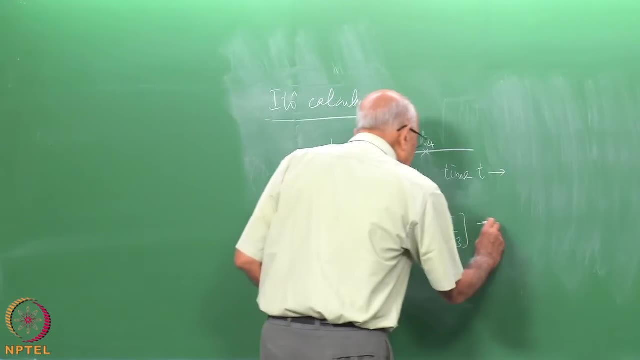 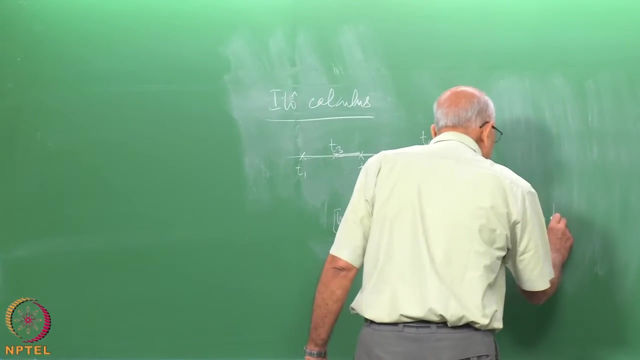 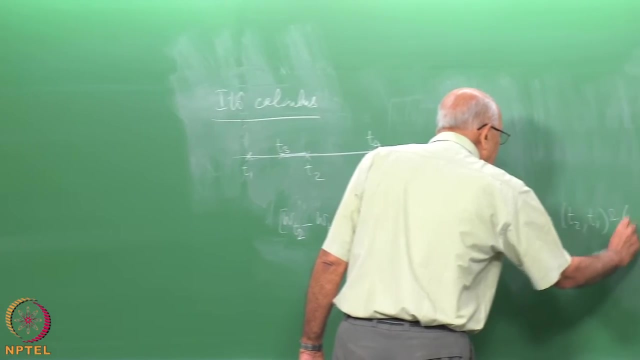 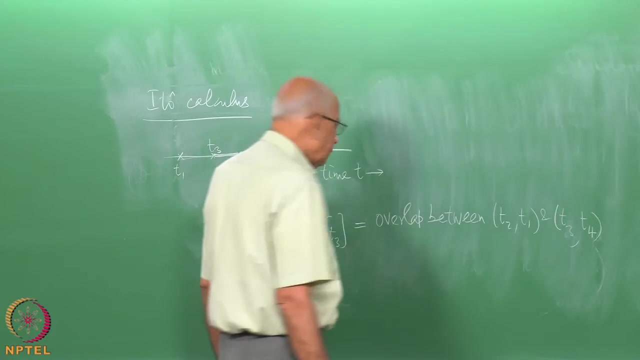 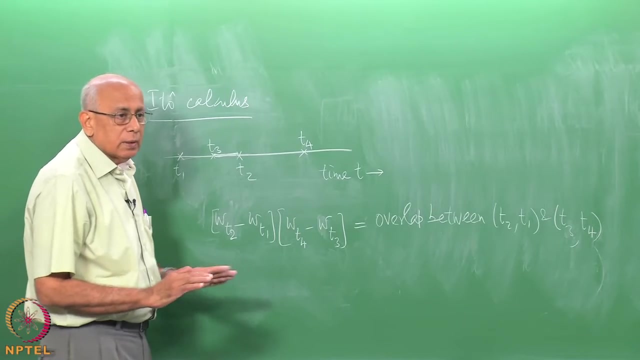 the two intervals. So you have one interval from t1 to t2, another interval from t3 to t4 and the overlap between these two is this guy here. So this is equal to overlap, length of the overlap between t2, t1 and t4, t3, t4. It has an immediate consequence. This, by the way, this statement. 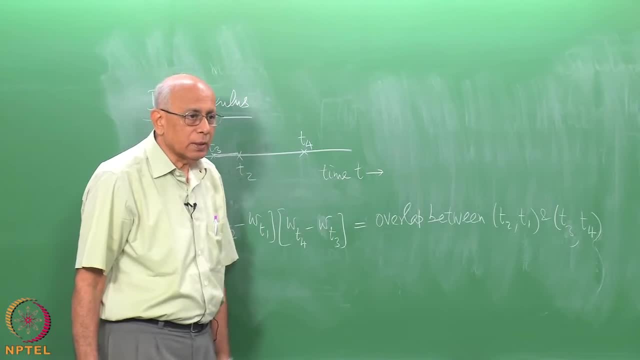 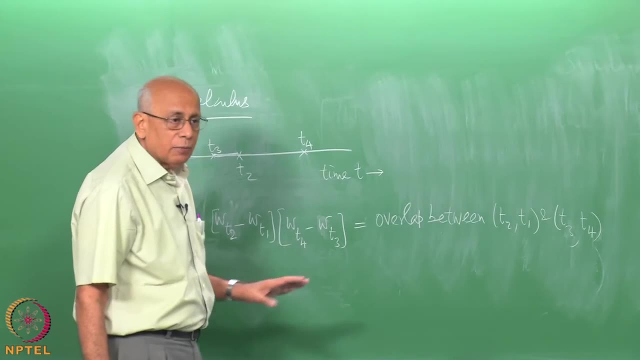 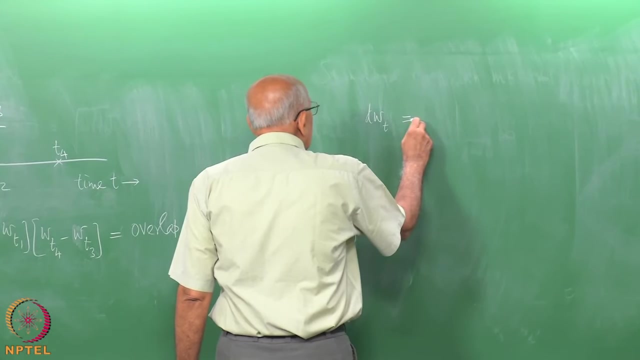 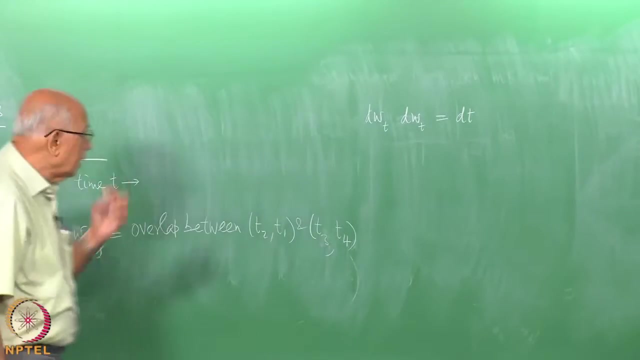 can be proved by looking at the correlation, the autocorrelation, Ok. And then it is a very simple proof here. Now this has immediate consequences. The first consequence is that dwt, dwt, dwt, equal to dt. Ok, because imagine a completely overlapped, infinitesimal interval. 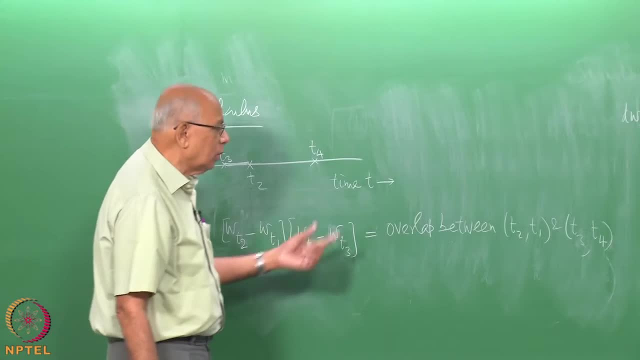 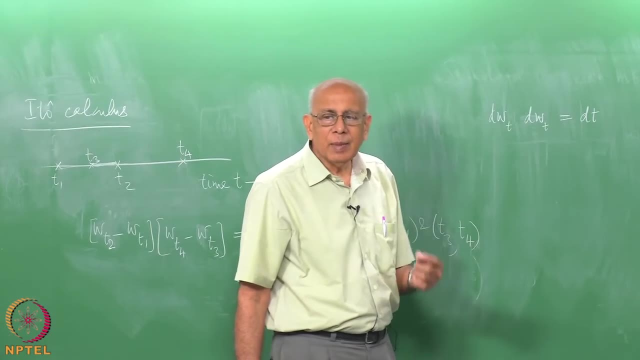 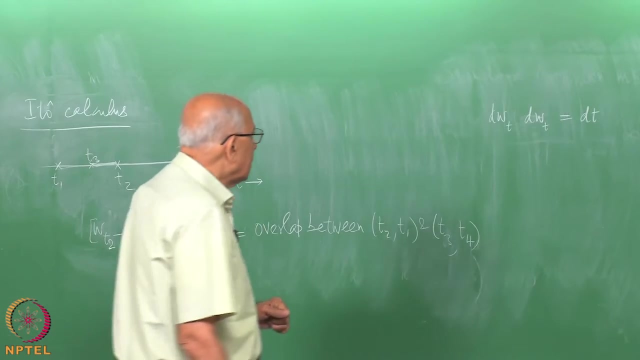 The length of it is dt and that is the square of dwt. So this is the one that formalises the fact that this dw, the increment in the Wiener process, is like the square root of the increment in time. Ok, This immediately has the following: 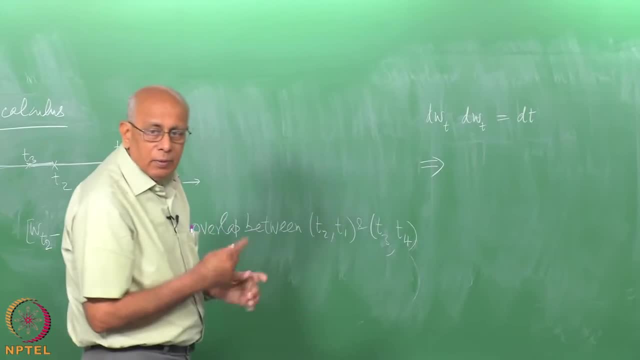 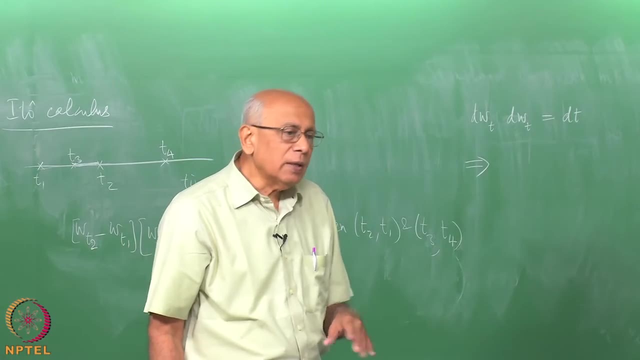 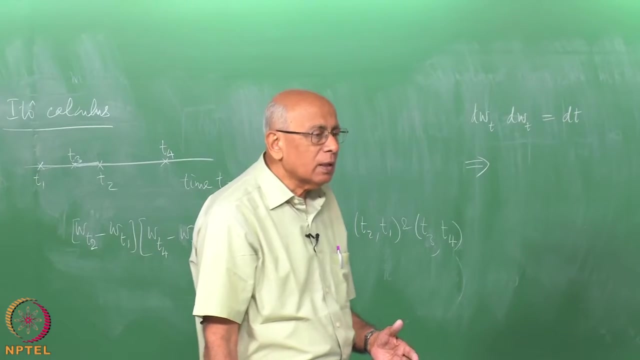 consequence. There are several ways of doing this. What we are interested in is asking for the behaviour of the properties of functionals of Brownian motion. Ok, X is a random variable in the normal diffusion problem. Now you ask: what does f of x look? 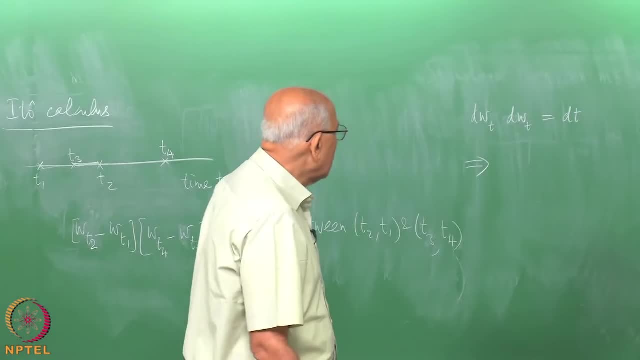 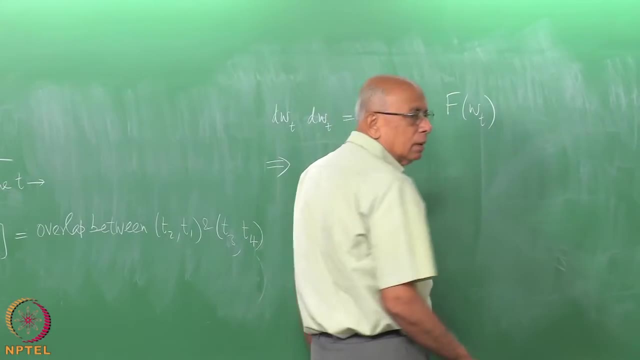 like where f of x is some function, etc. So we are going to consider what happens. if you had a functional, just write it as fwt. you could extend it to the case where it has an explicit t dependence as well. we will do that in a second. What happens to this? 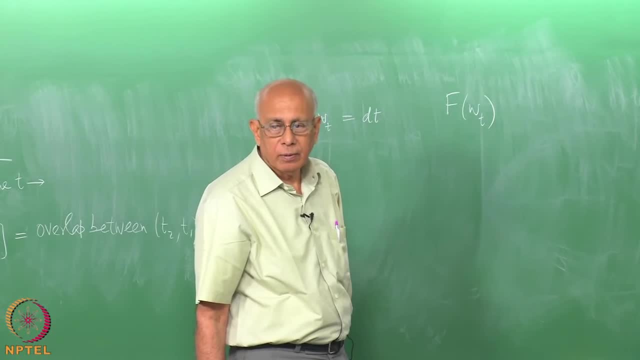 functional and what does its differential look like? Ok, What you have to do is to do a Taylor series, So it doesn't matter if the t dependence is a t or t is not there. it is always a t. This is how it works. 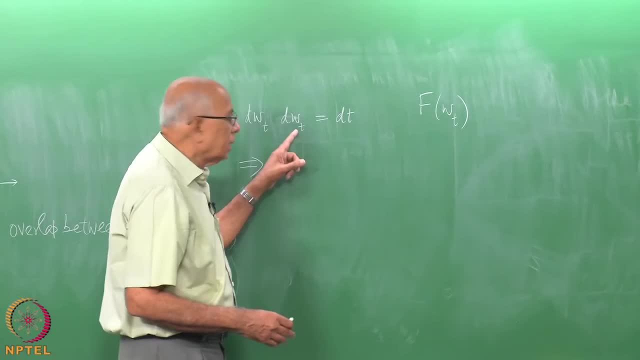 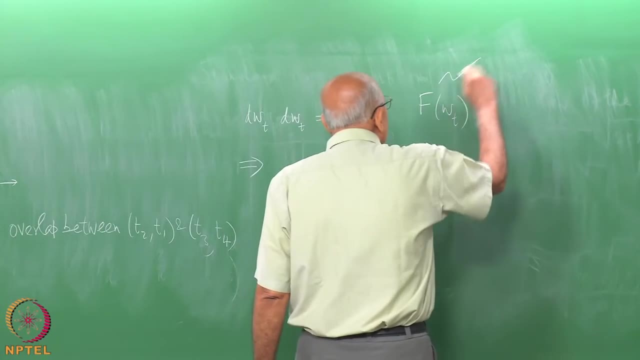 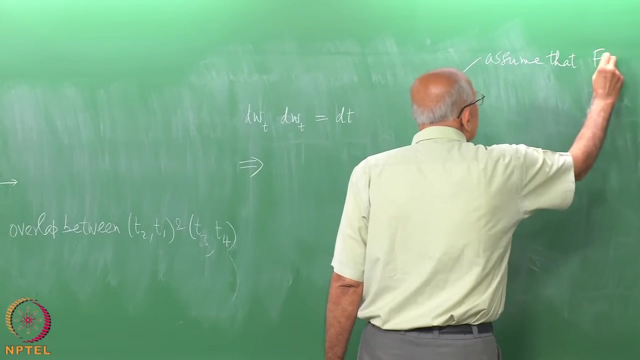 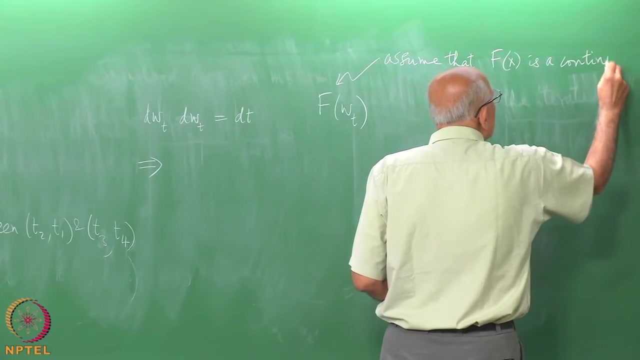 The wwt. the wwt is basically the wwt on this field, So you don't have to worry about any particular point And keep track of the fact that this thing here is like dt. Ok, So we will assume that. assume that f of whatever argument, f of x is a continuous twice p. 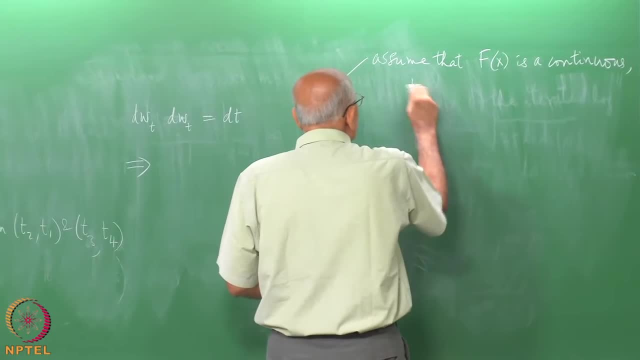 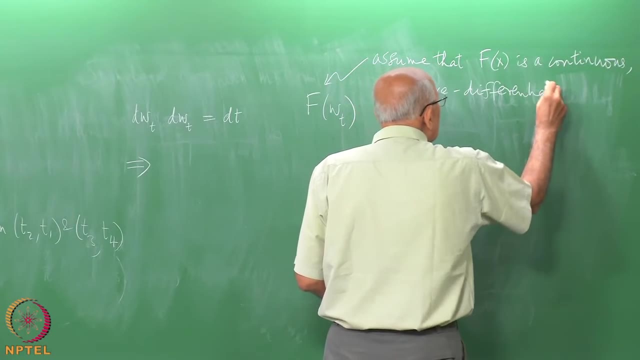 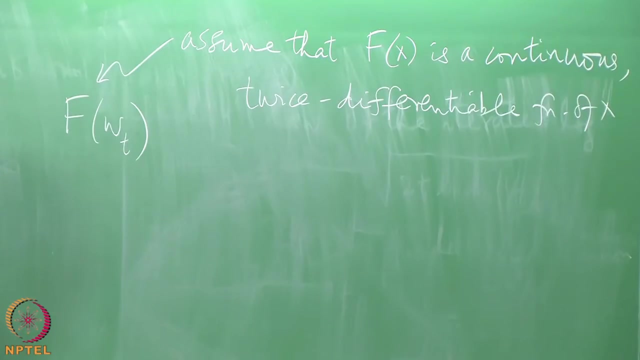 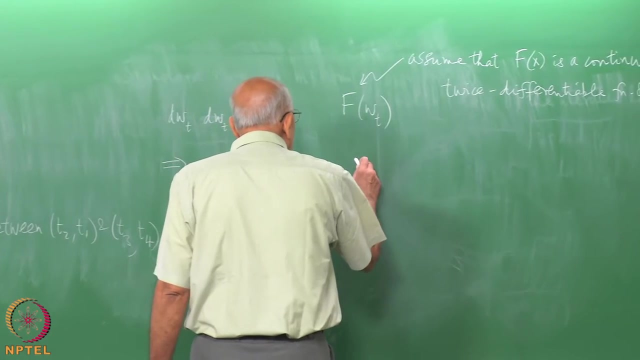 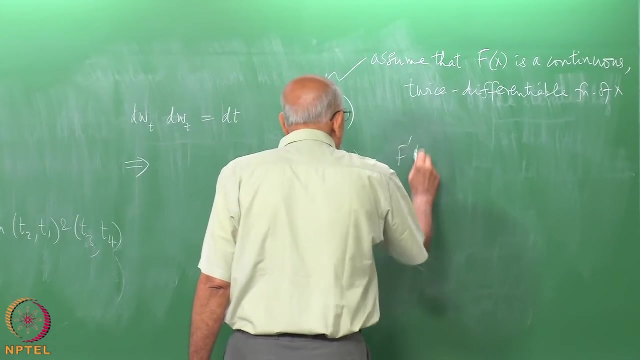 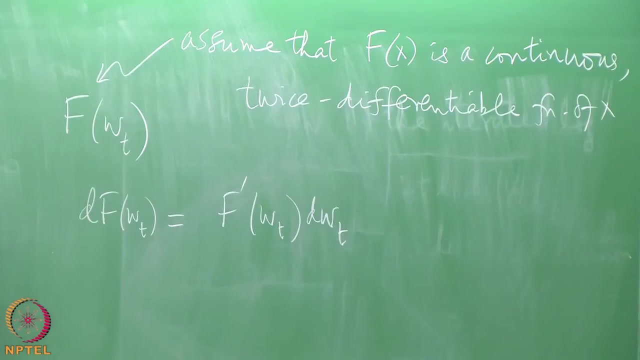 x, No, No differentiable at least twice differentiable. We will consider functions which are at least twice differentiable, functions of the argument. Then we could ask: what is d, f, w, t? This is equal to f prime, w, t, d, w, t. that's the first term, right. But that's not enough, because 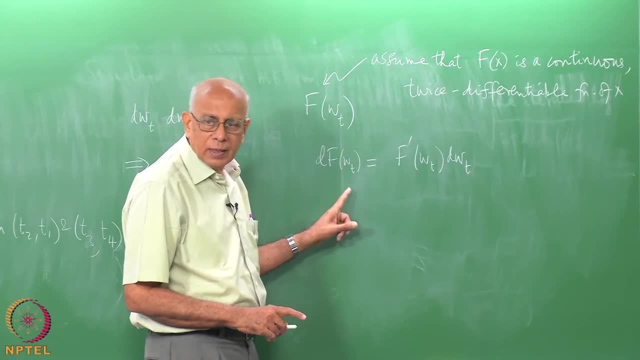 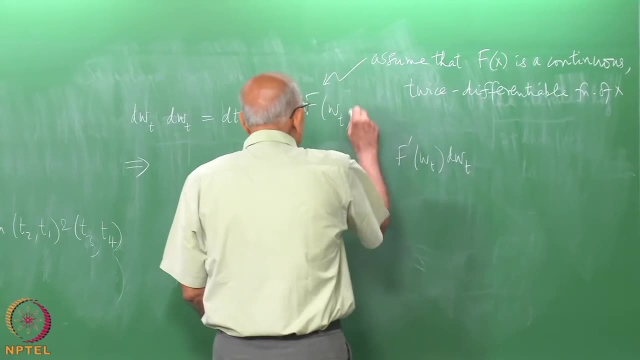 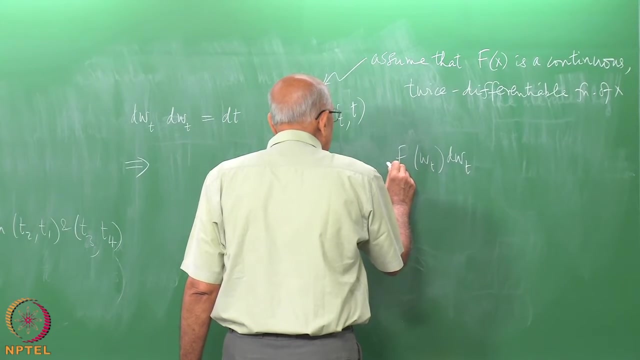 it's a function of a function. There could also be an explicit time dependence here, So let me in fact write that time dependence. Let's look at the more general case where you have 1. This then is: well, let me use the following notation: f prime, and I will explain this. 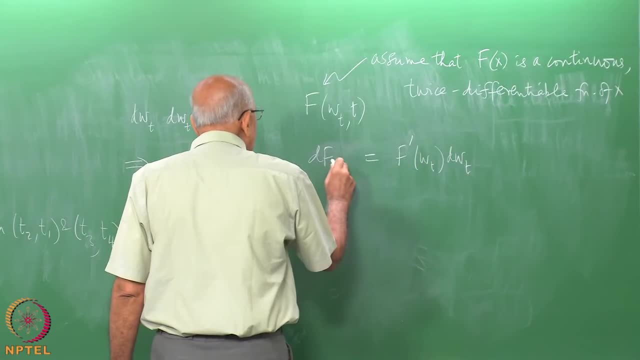 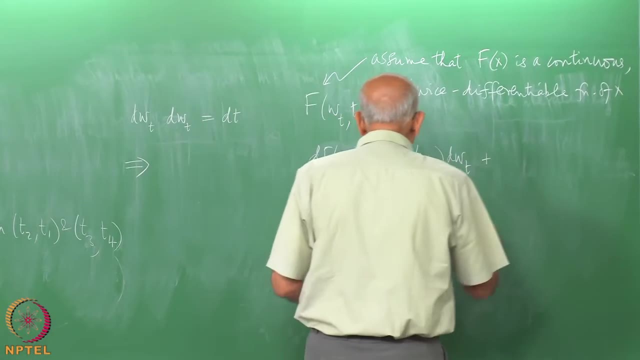 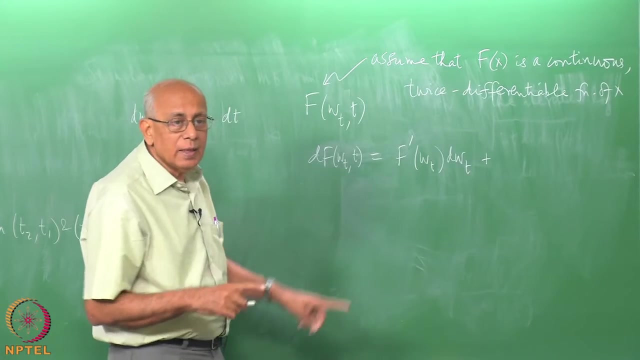 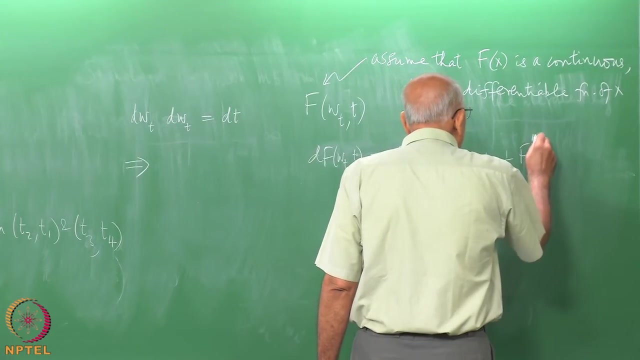 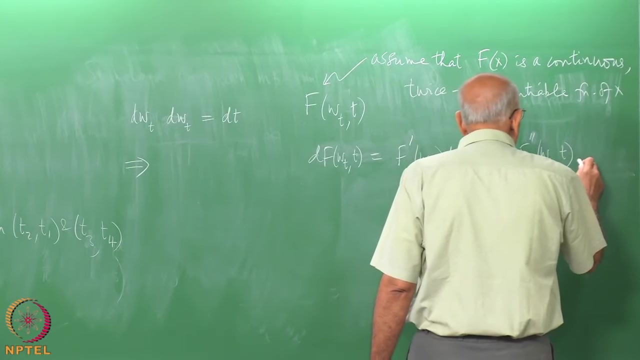 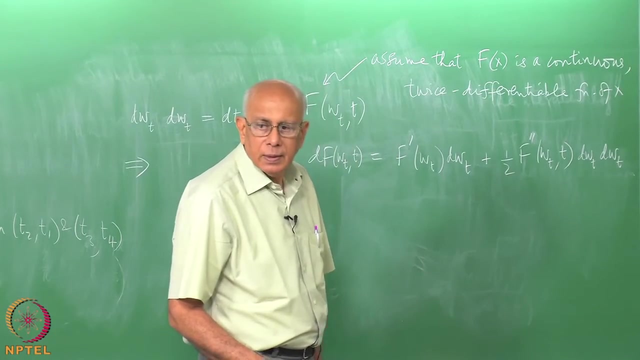 notation in a second So d f of w t t equal to this, plus a portion coming from the fact that the second term in d w t will still be of order d t. Then that term turns out to be one-half f double prime: w t t, d w t, d w t. Ok. 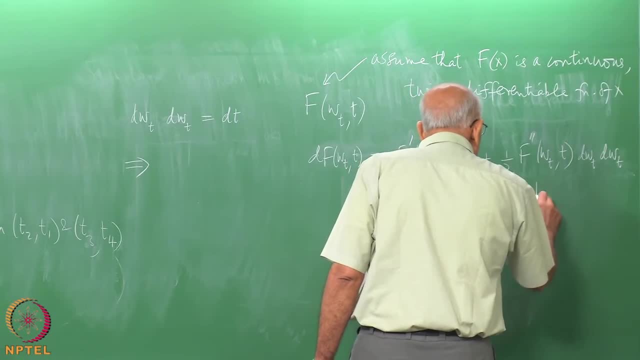 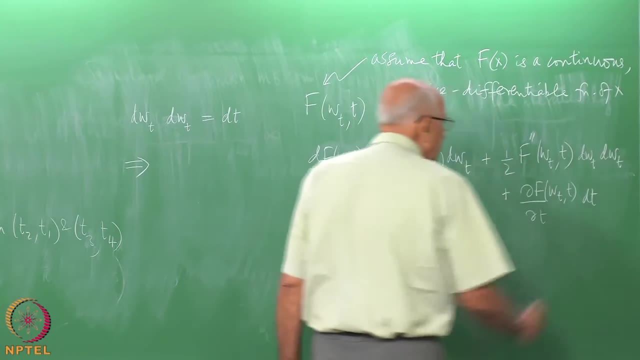 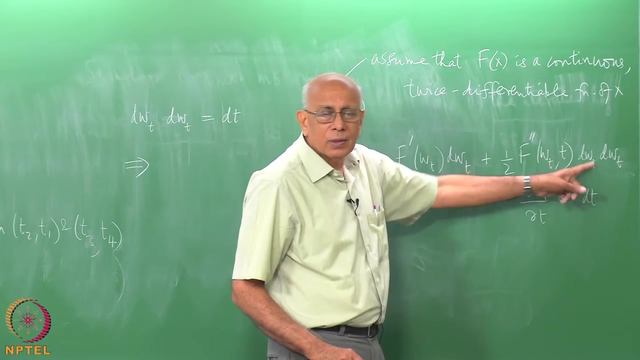 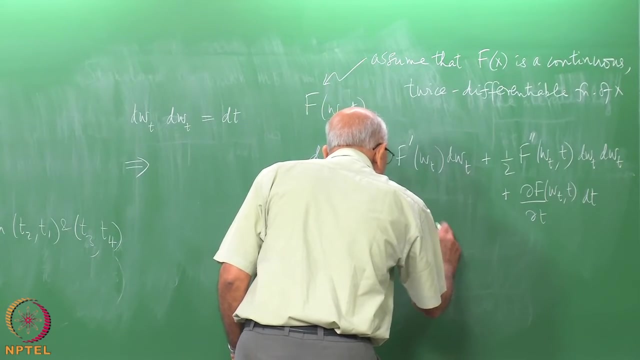 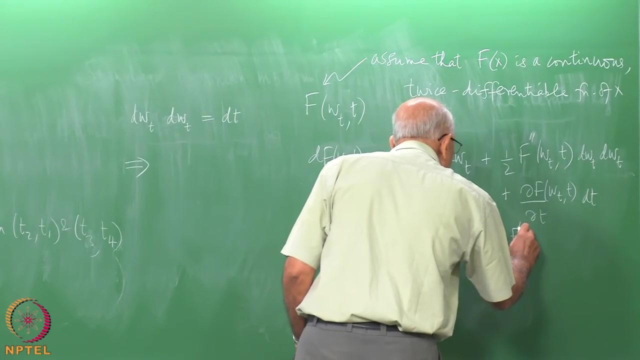 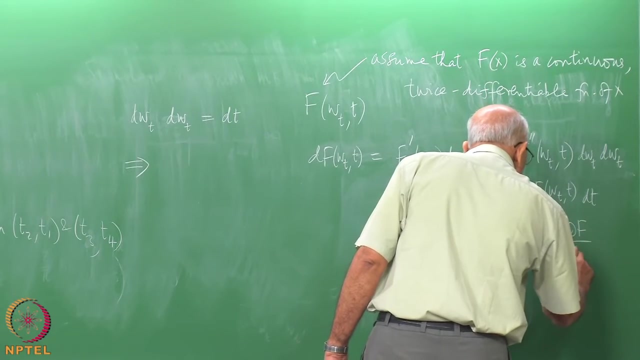 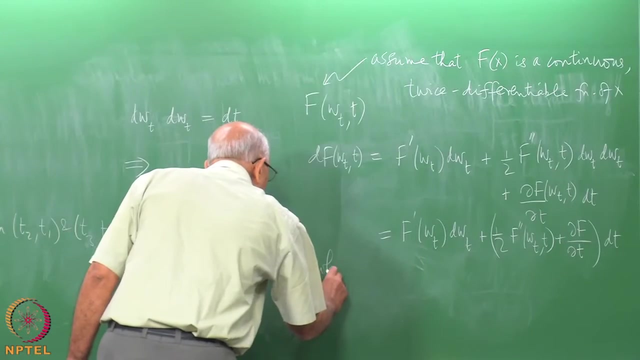 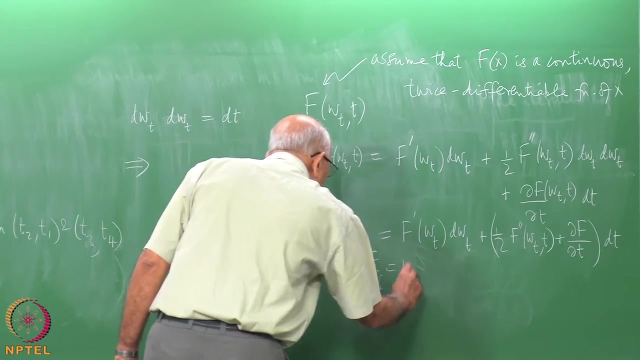 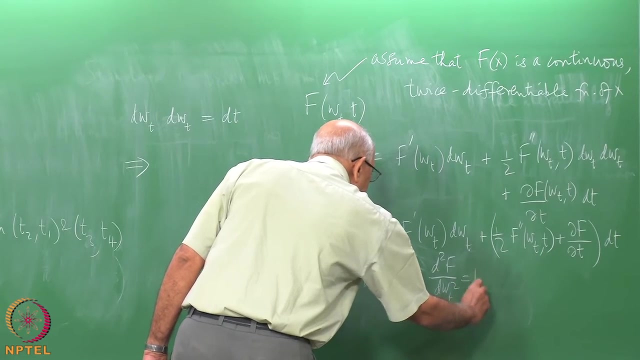 Plus the time dependence of W t t over delta t d t. Ok, But we know that this is d t, so it gets added to this term. Ok, Now, this is the fundamental rule of Ito calculus, where Ah d f over d W t is equal to f prime d to f over d W t. So you differentiate with respect to. 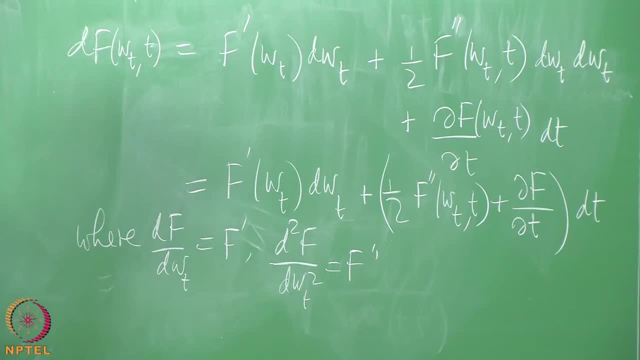 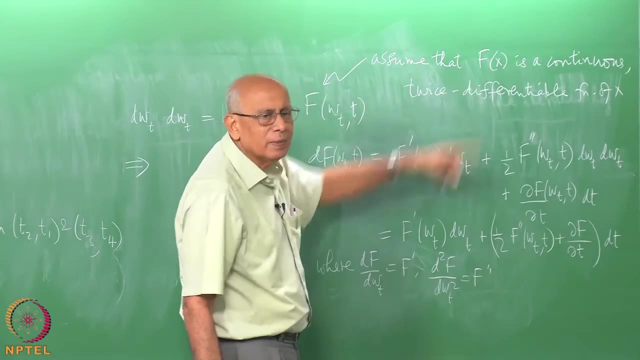 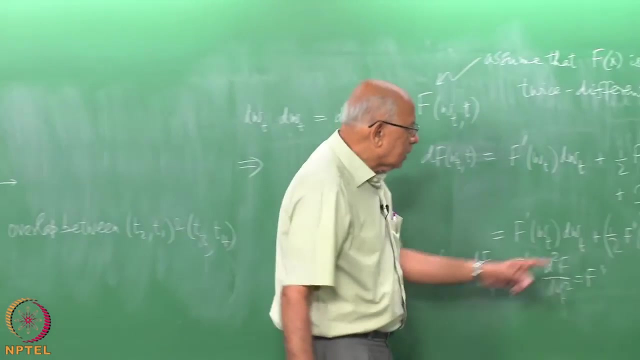 W, t alone, Those are the 2 derivatives. You already assumed that. well, I should really write f of x. t is twice differentiable in x, Ok, Ok. Now the addition of this extra piece here helps you. that is the amendment that the 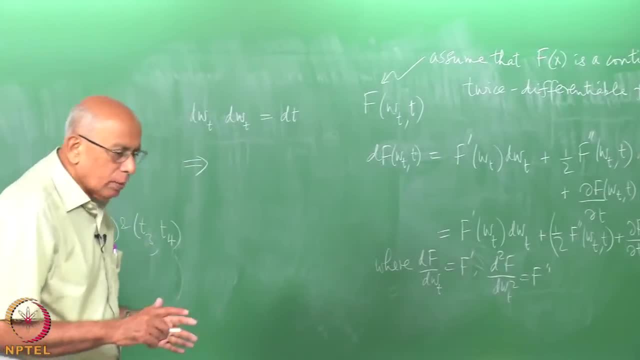 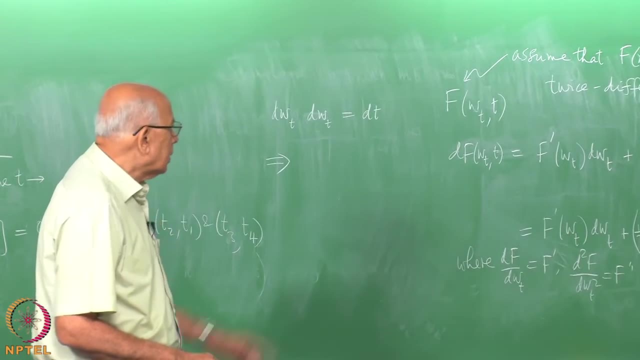 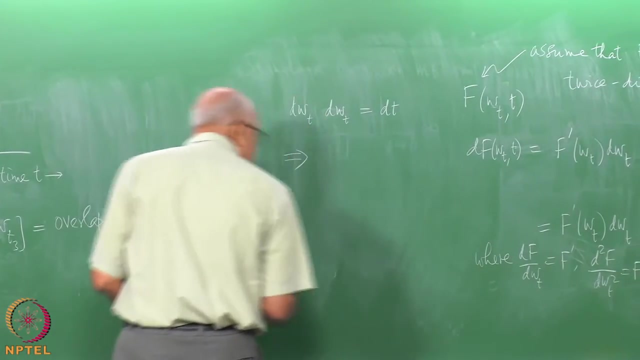 rules of calculus need in order to be applicable to as singular objects, as Brownian parts, as a Wiener process, Because this is the differential form, the integral form of this will tell you what the correction is in normal cases. So remember this rule, this here. Now let's. 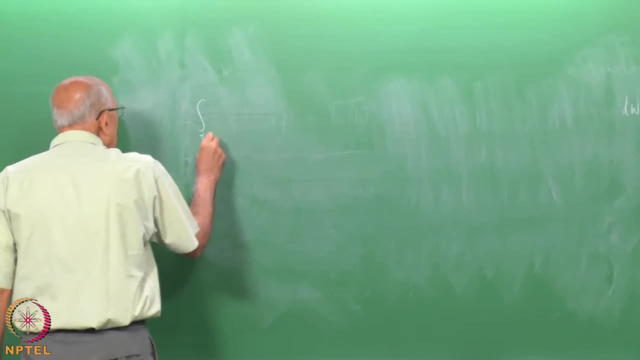 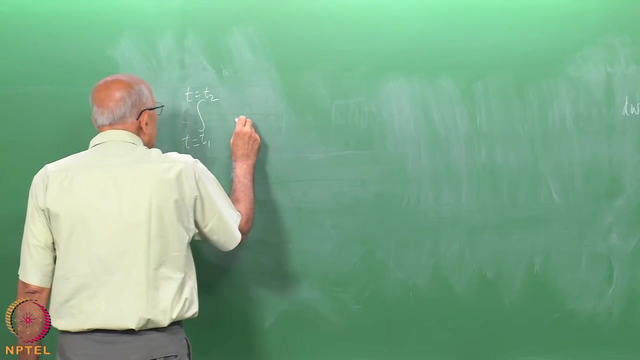 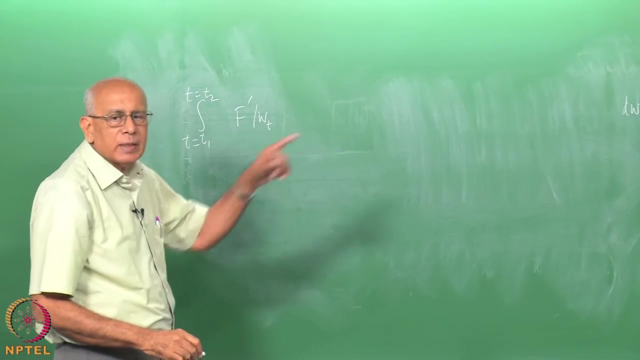 look at. Let's look at the integral of, say, t 1 to t 2, t equal to t 1 to t equal to t 2, of something like f prime of W t. Let's look for the moment at functions which are not explicitly time. 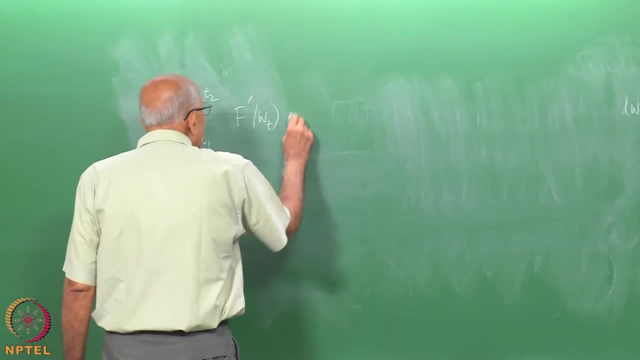 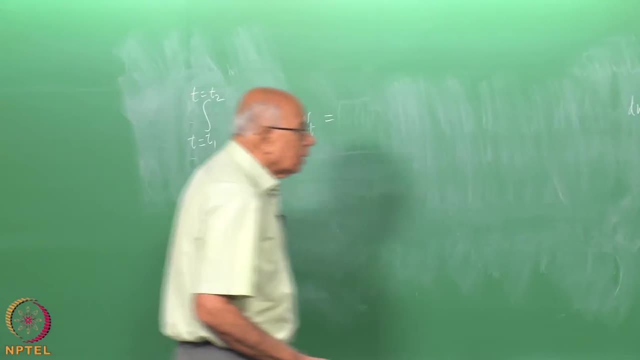 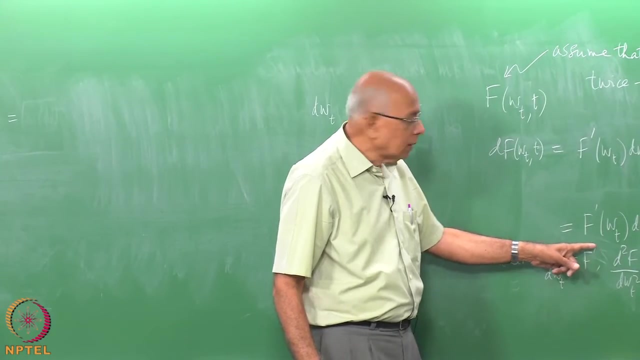 dependent. So you see what the correction is: d W t. What is this guy equal to? Well, we are integrating both sides of this. Ok, We are integrating both sides of this equation here And we are asking: what is this fellow? 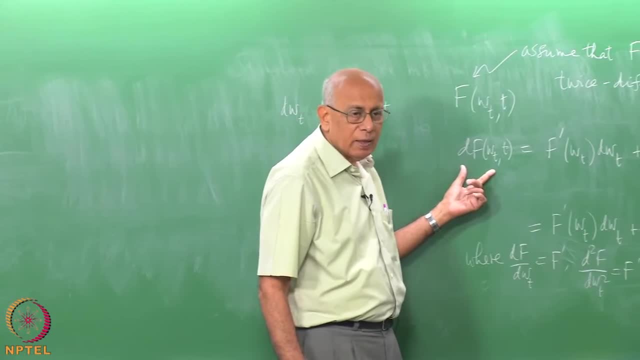 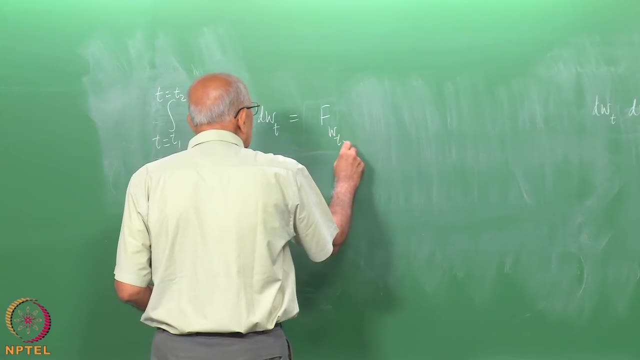 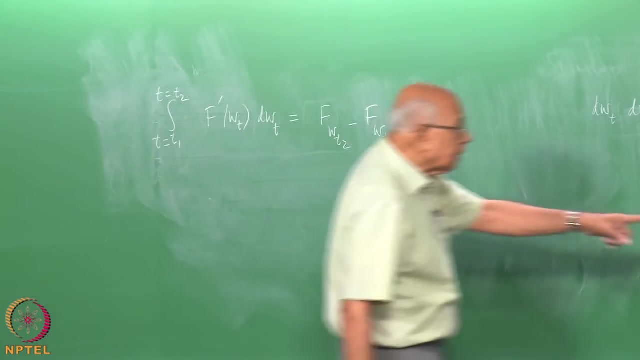 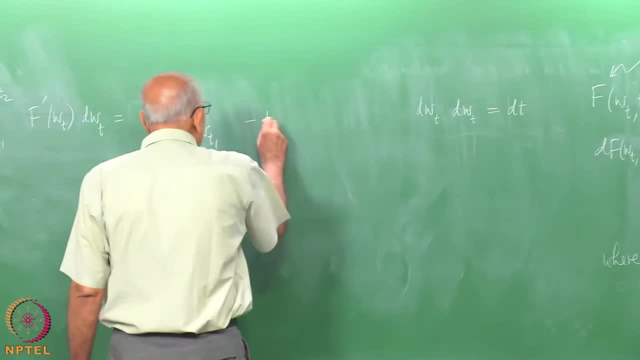 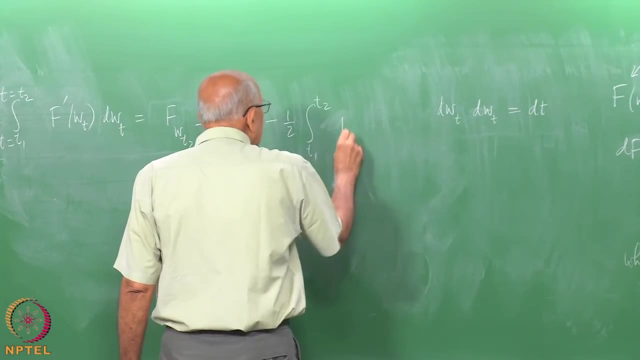 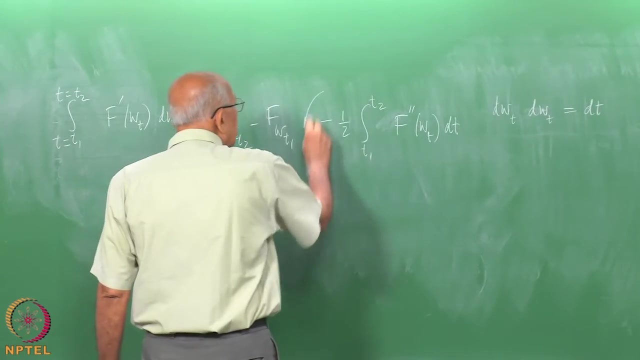 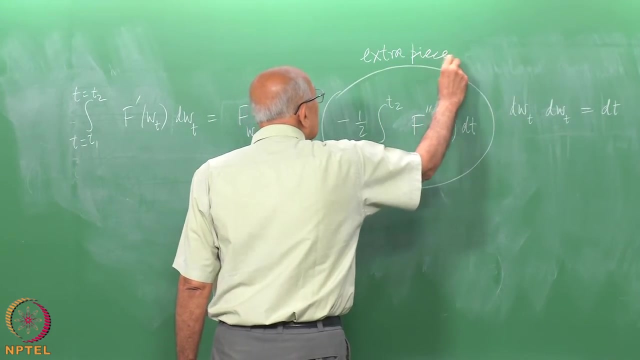 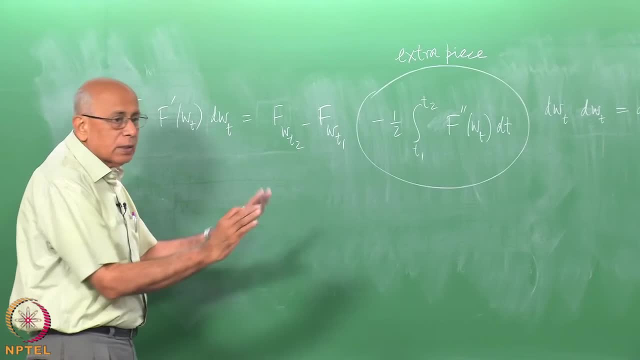 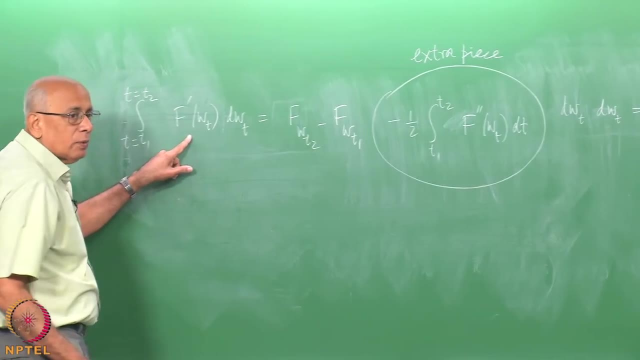 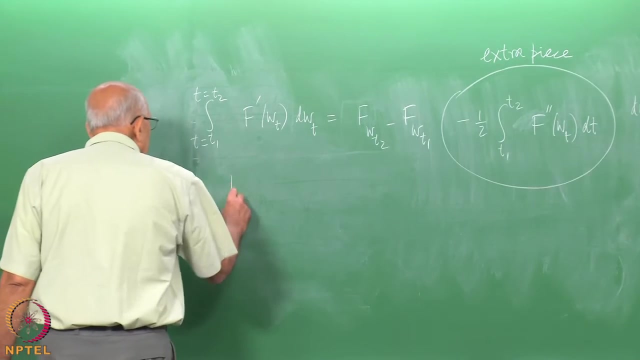 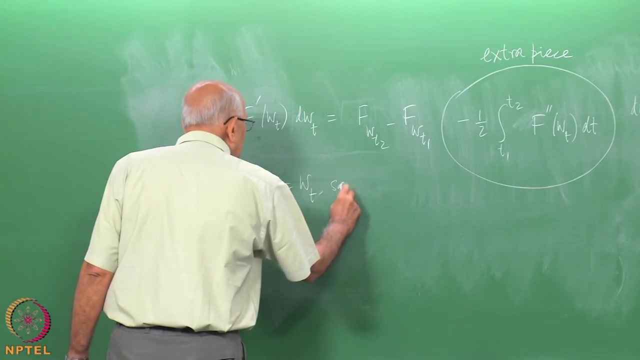 this. Ok, Ok, Ok. Let's see what this is doing for us, what it implies. Let's first look at a case where this f prime of W t, let's say, is W t itself. Then it tells you that integral t 1 to t 2. 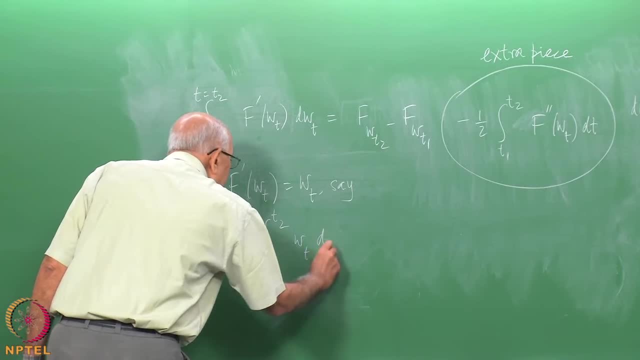 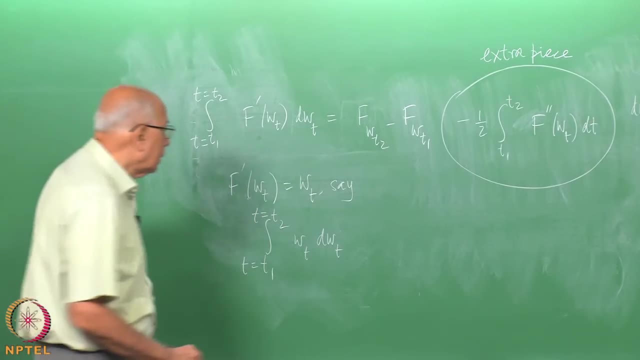 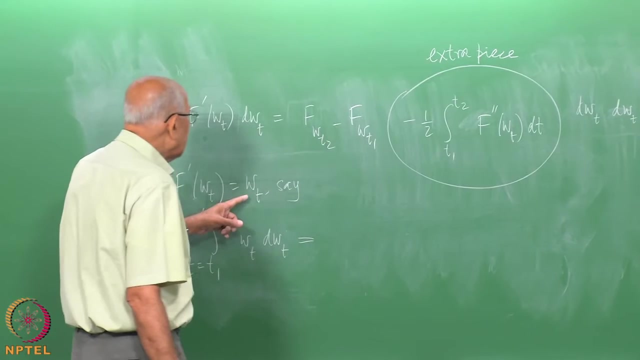 in time. Ok, W t d W t. I should write t equal to t 1, t equal to this is equal to. by this, applying this theorem, applying this blindly, it is the integral of this fellow, which is W? t squared. 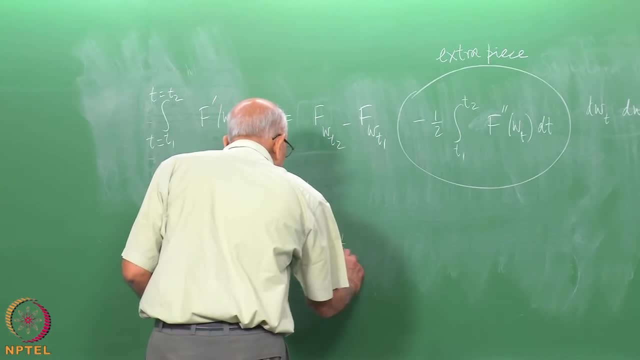 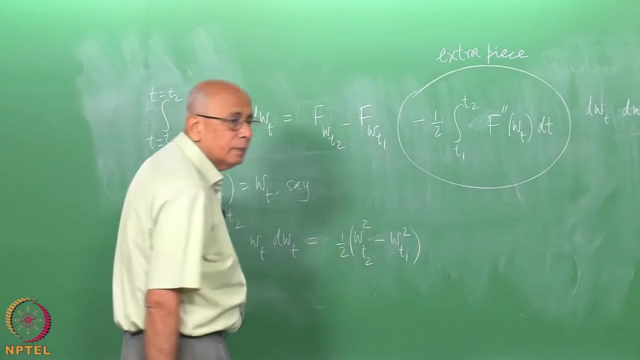 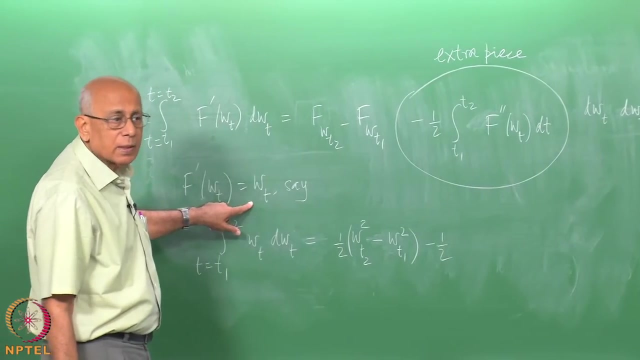 over 2.. So it is half W t 2 squared minus half half comes out minus half. half comes out minus W t 1 squared minus half. well, f double prime is 1 in this case. So it is. 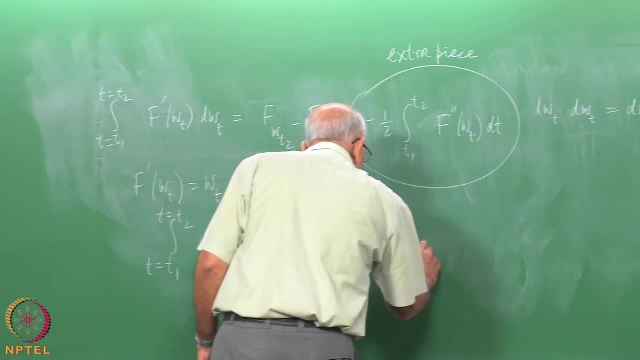 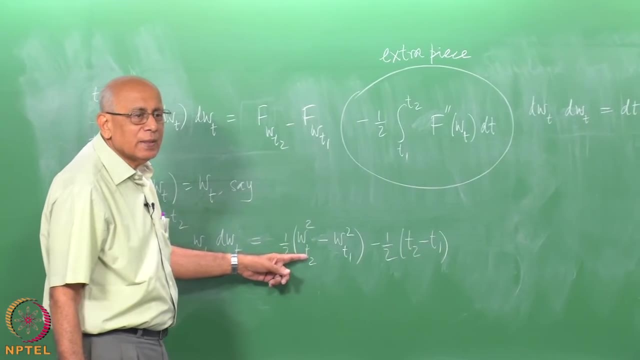 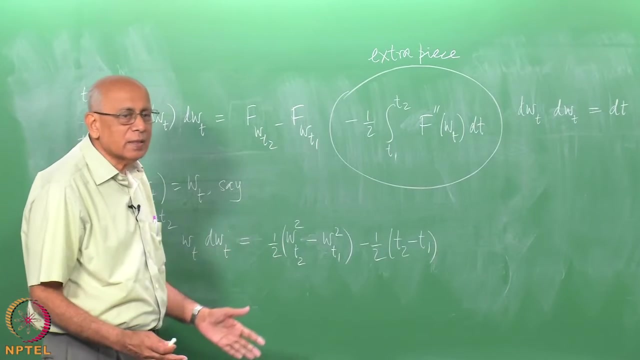 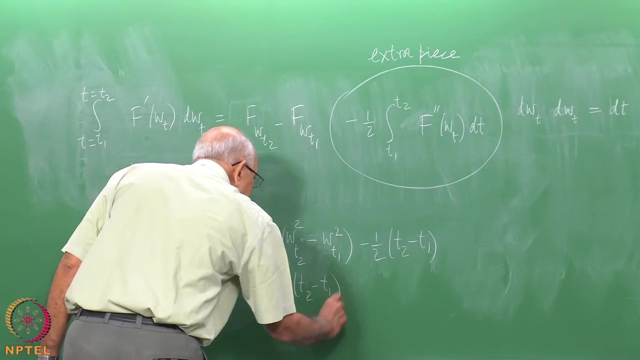 just t 2 minus t 1.. Ok, But this is equal to t 2, right? We already had that overlap rule, And so this, And so the square of W t squared is t itself. So this is equal to half t 2 minus t 1 minus. 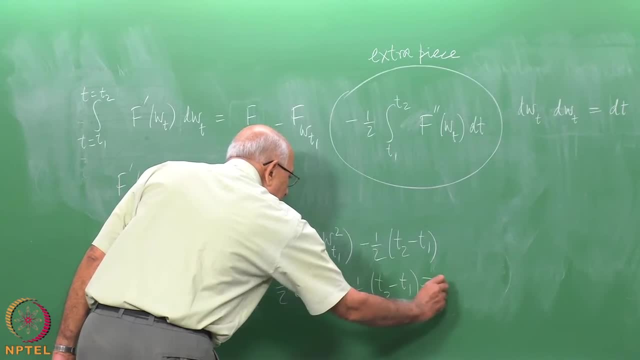 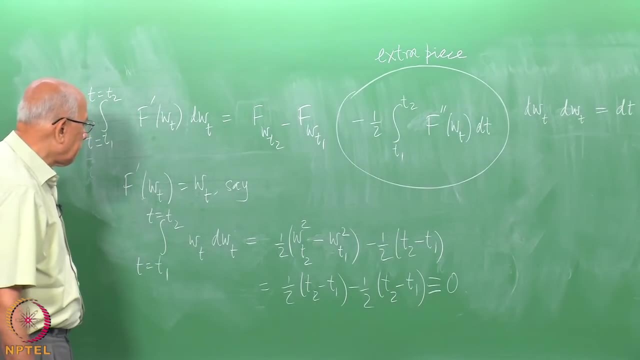 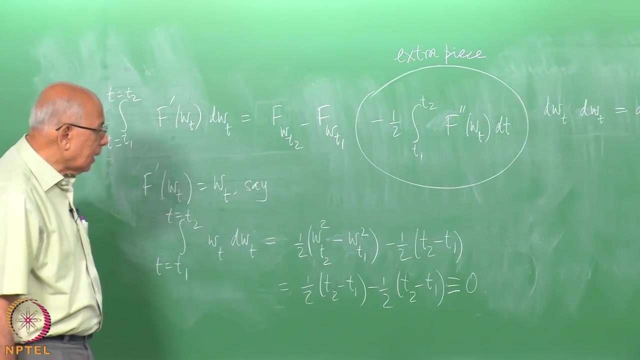 half minus t, 1 is equal to 0, is identically equal to 0.. Ok, Because of the way this Ito calculus works. Now what does that actually mean? I mean, this is actually a very simple, very simple question. 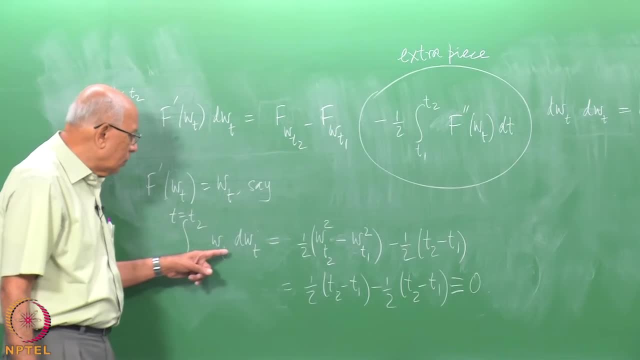 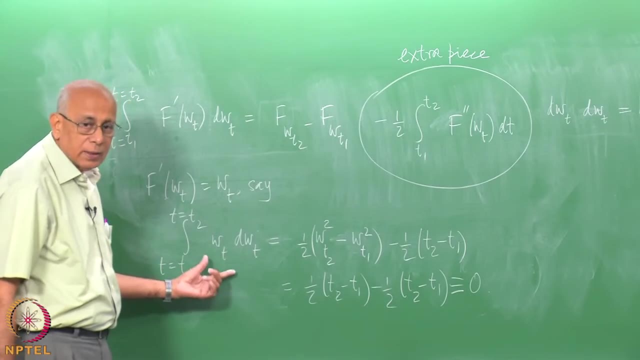 because there is no such thing as total theta. this is felt in the respect of, you know, is an important result because it tells you this thing tells you that there is a specific interpretation being given to this, this process here, this integral here. So it says that: 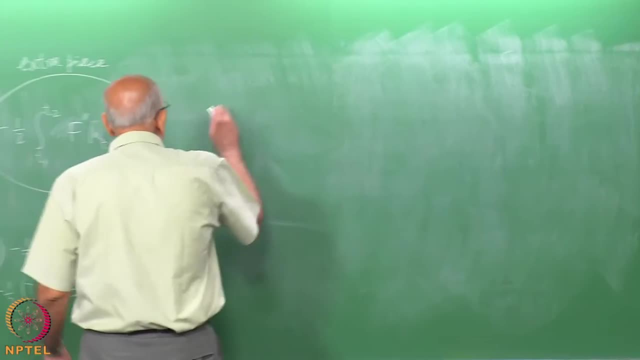 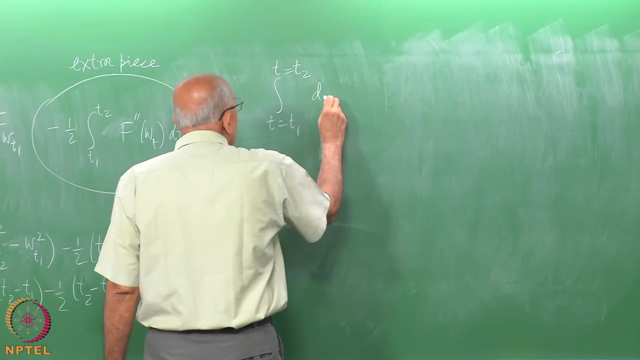 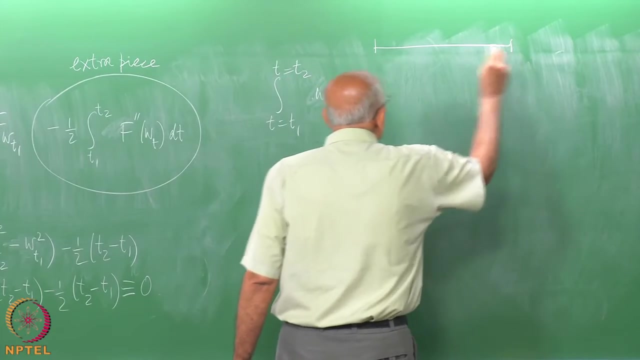 what we mean by that integral. so since we can write t equal to t1 to t equal to t2, dW t can be written in the following way: So I start with time t, time 0, time t and I break this up into n parts. So there is time tn and time tn plus 1 equal to t and this 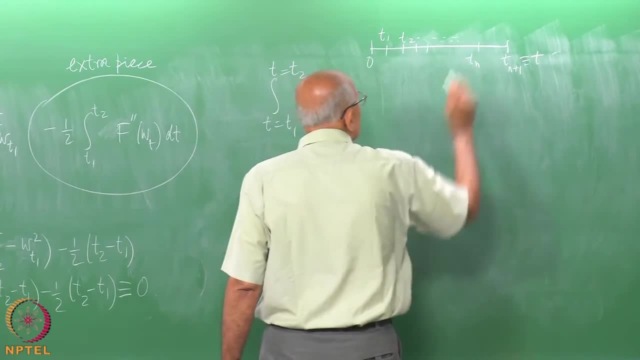 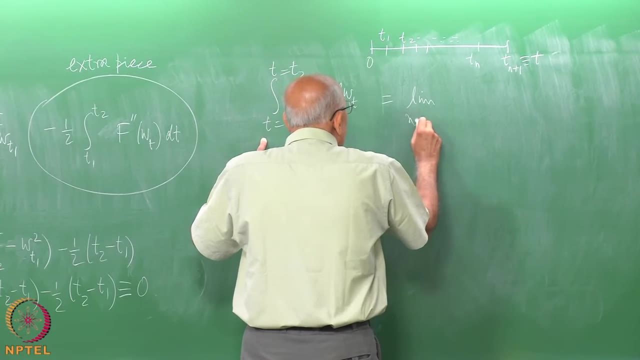 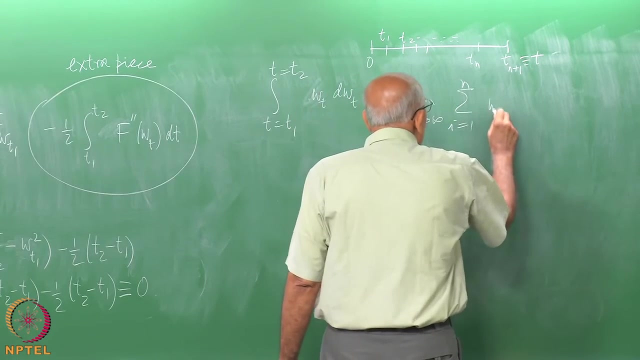 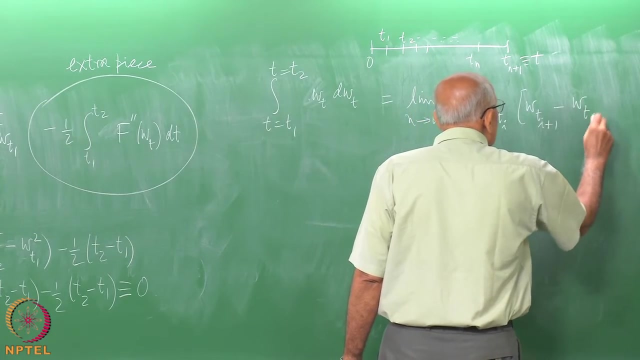 is 0. So this is t1,, this is t2, etc. break it up, Then this is equal to limit. n tends to infinity. Summation from I i equal to 1 to n times w t i times d w. but this d w is w t i plus 1 minus w t sub i here. 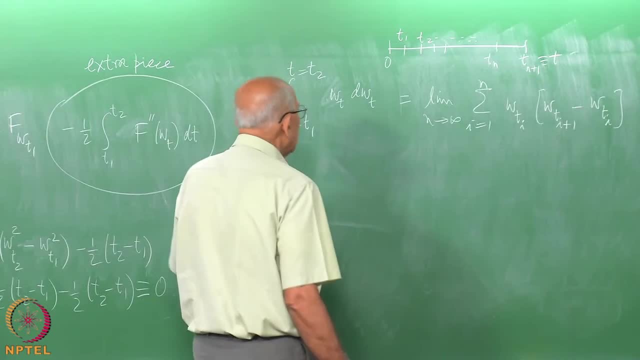 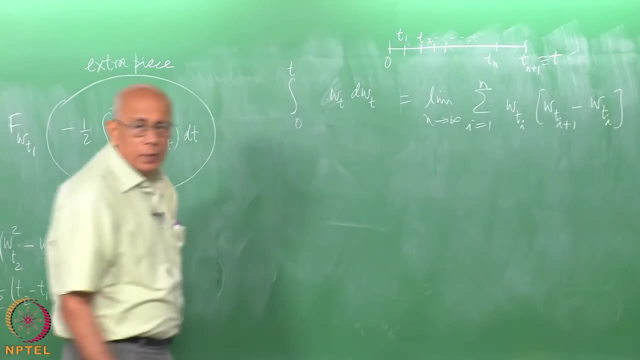 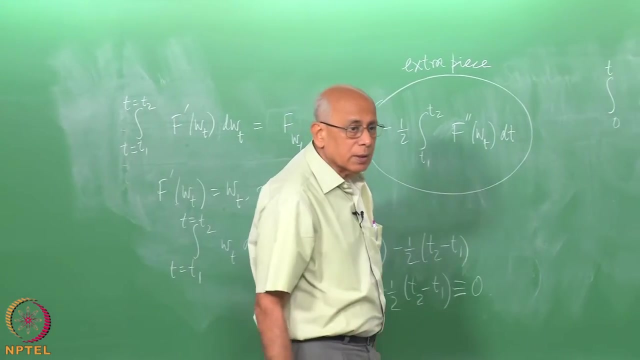 It is the forward difference. oh sorry, I am sorry. yeah, I chose it to be 0,. yeah, I started with 0.. This is a general result. this fellow is a general result here, but you can start at any point in this process. I start from 0 and it is the meaning of this. So it is. 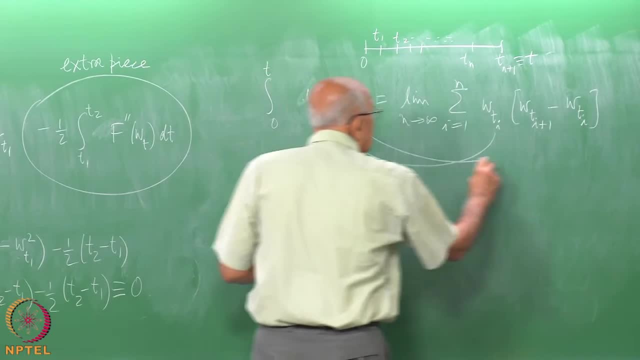 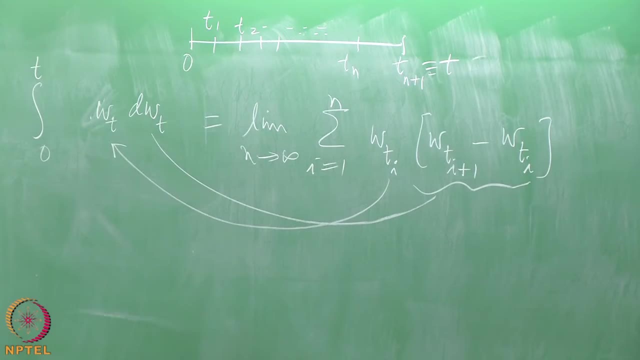 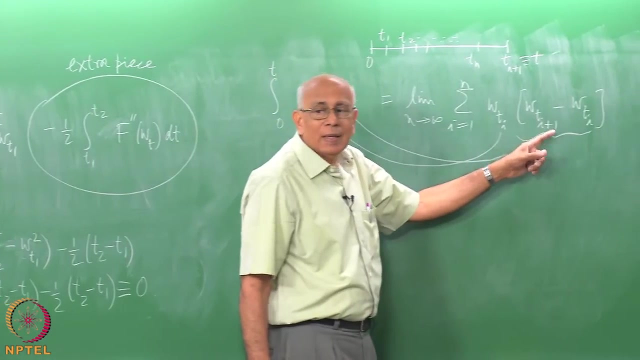 this quantity that has been written there and this fellow is this difference here in the limit, As the number of intervals, number of subdivisions, becomes infinity. Now, this is the forward increment and this is the current value of the variable. We know that the overlap between 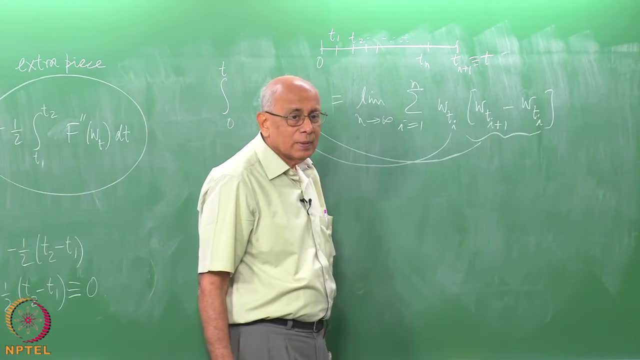 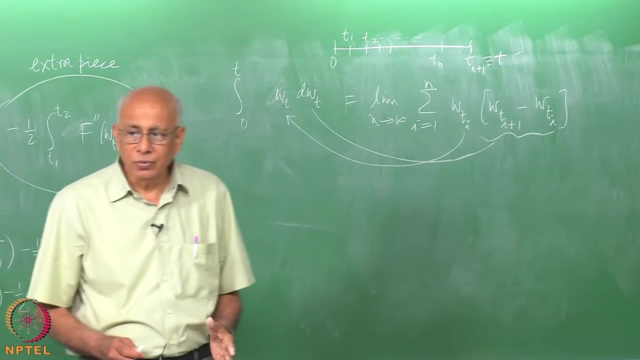 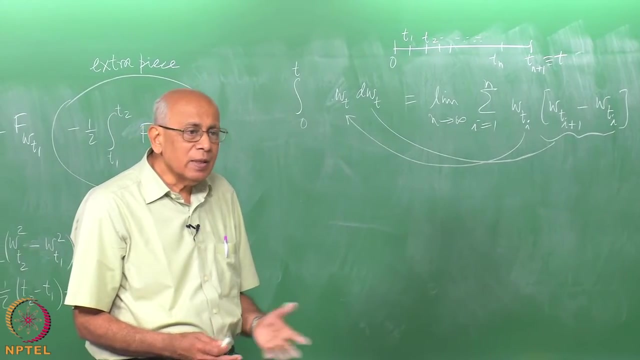 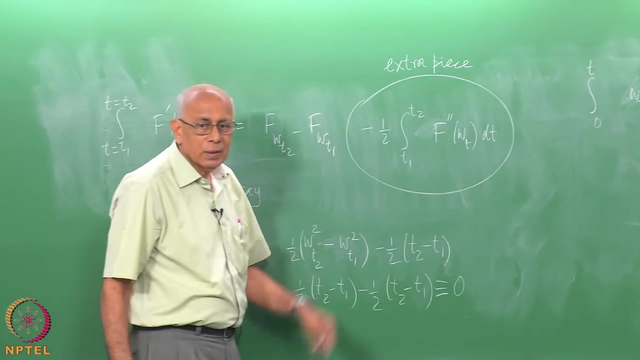 these two is 0 because this goes up to t i and this goes beyond that. There is no overlap between these two integrals and these two factors. Therefore, by our basic rule for Brown ian parts this: they are independent. This is 0.. That explains why you get 0 here. 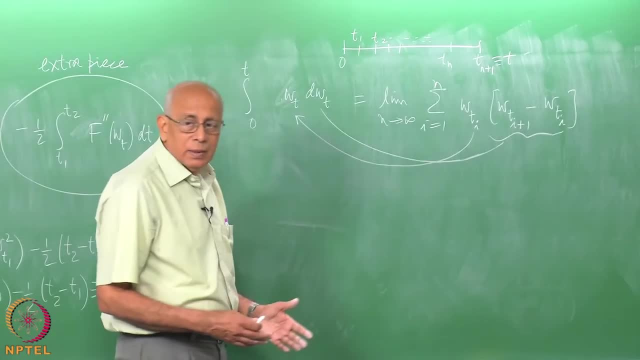 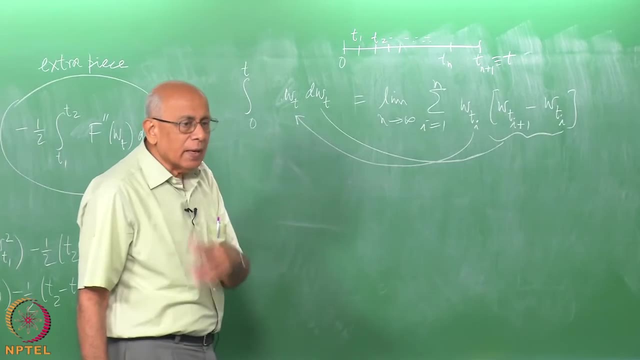 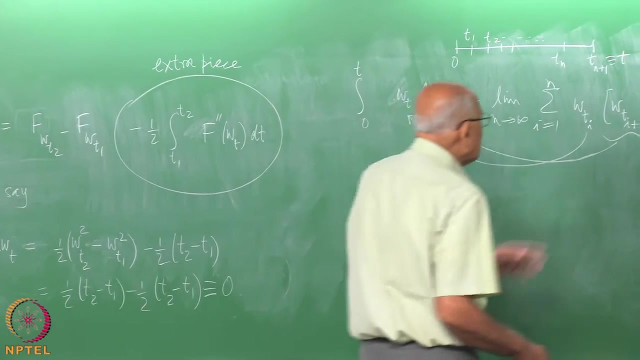 Now you could have interpreted it differently. when you do normal integration from a summation, you convert it in integration. There is no reason. so you normally write f of x, d, x, etc. Now you write it as a sum. this d x is say x plus delta, x minus w t i times w t i minus. 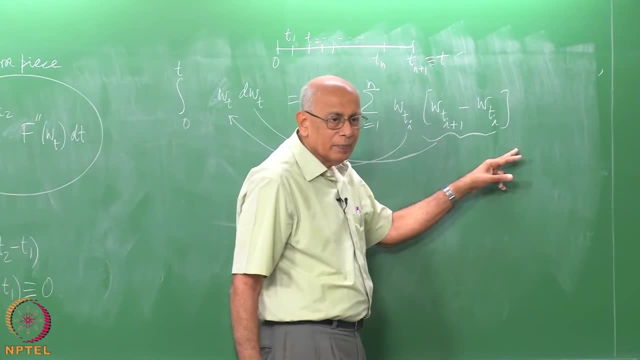 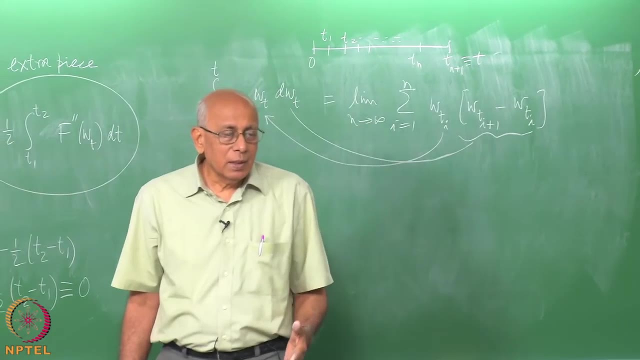 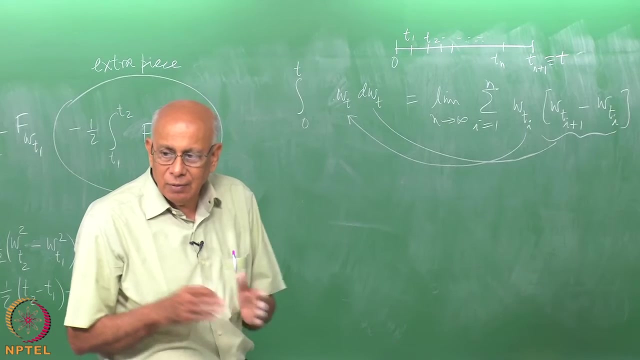 delta x minus x. but this quantity here, f of x, is x, at which point It could be at x plus delta x over 2. It could be at any combination of f at x and f of x plus delta x. So this is Ito's choice. 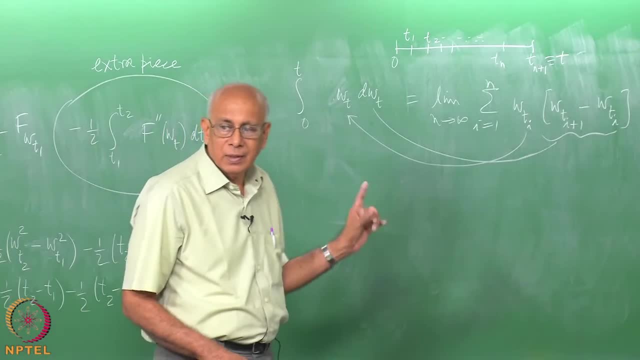 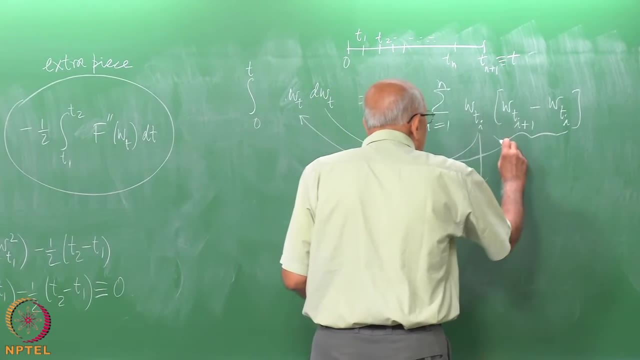 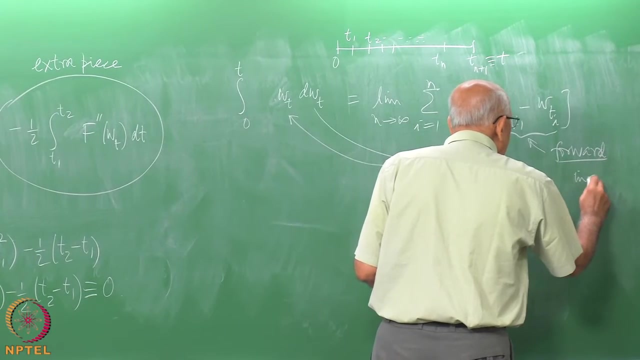 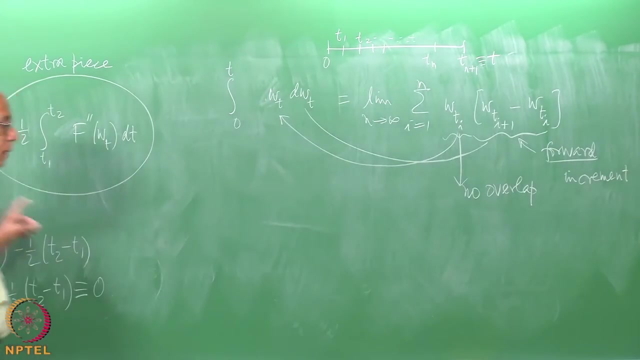 This is a specific choice of the way this integral is interpreted. the interpretation So this: this: the fact that these 2 factors no overlap. and this guy here is the forward increment. it is this that is gives you the Ito calculus and all the other properties. 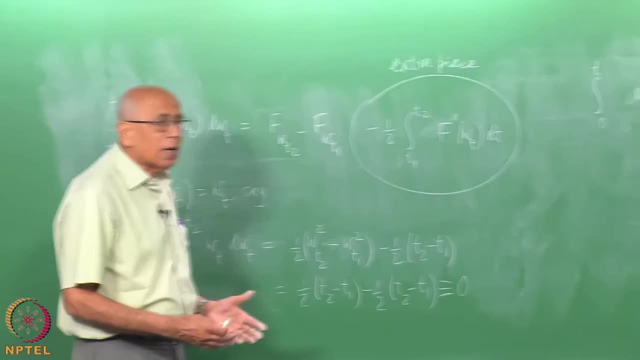 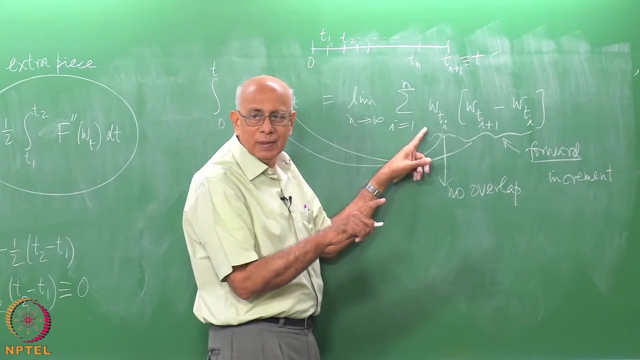 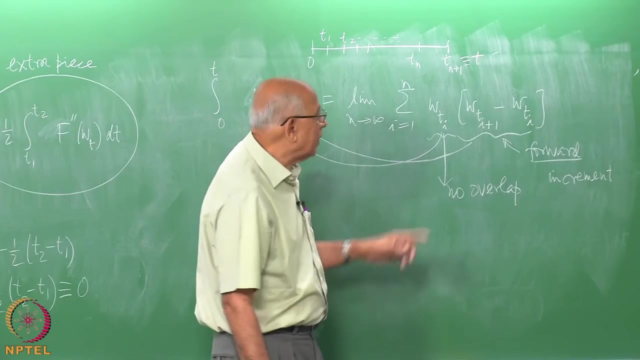 that I wrote down So clearly. it says that there are other choices. What choice is possible? You could choose this to be t? i plus 1, for example, or you could choose it to be t? i plus t i plus 1 divided by 2.. So you have any number of choices here. 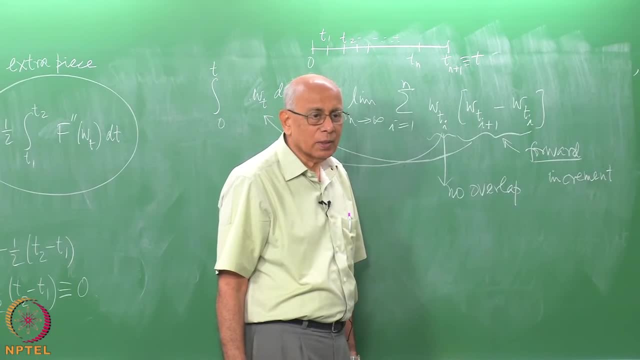 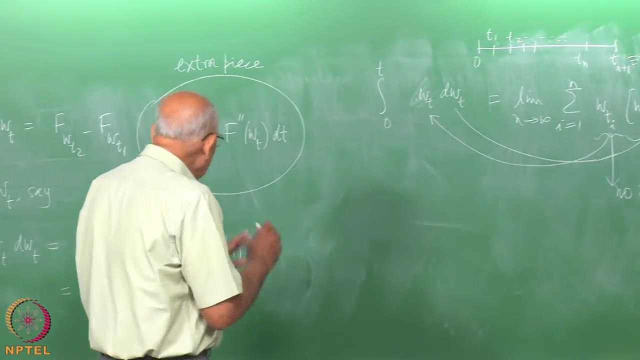 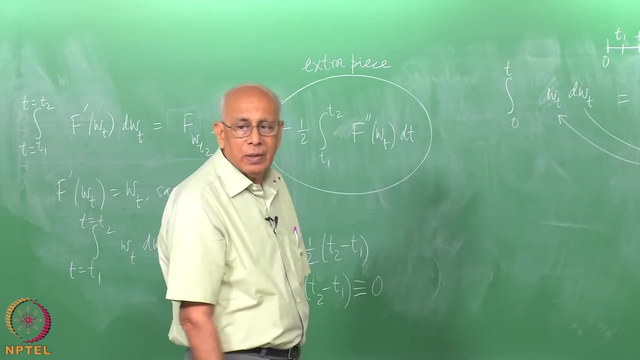 and each time you get a stochastic calculus. Ok, Now if you choose the Ito interpretation and you have this feature, then, and only then does it turn out that the interpretation is correct. So the interpretation we have for the general Langevin equation or general Ito equation: 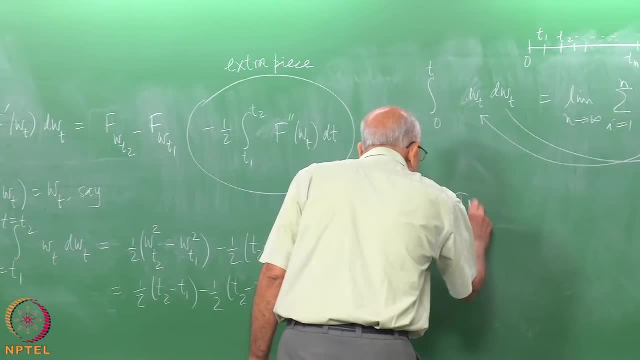 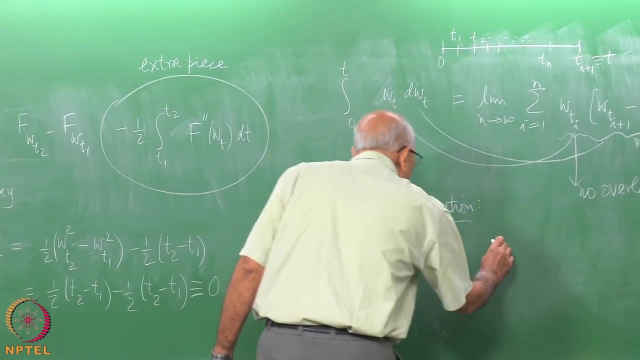 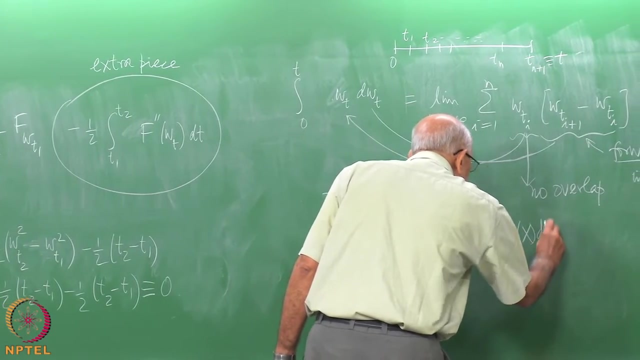 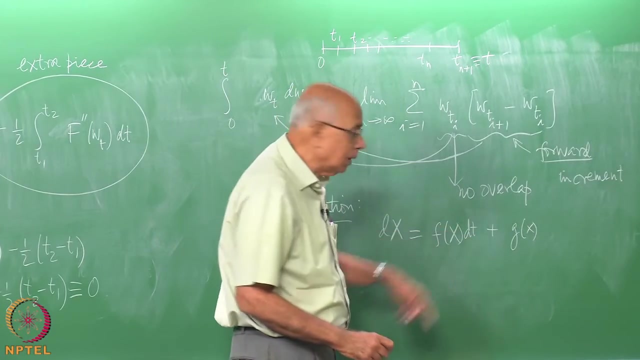 now. So our general Ito equation, stochastic equation, I shouldn't call it Langevin anymore. This is of the form. some process d x is equal to some f of x, d t plus g of x. remember the Langevin equation that we wrote down with the drift term and the diffusion term There. 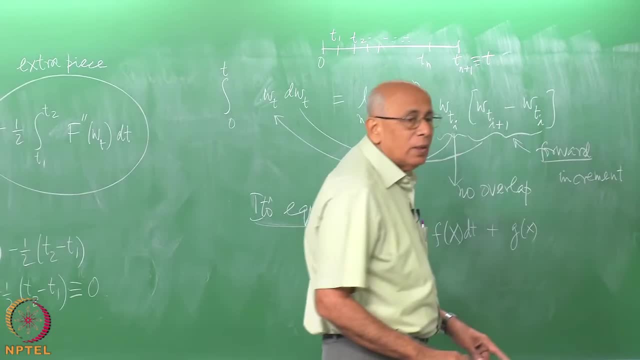 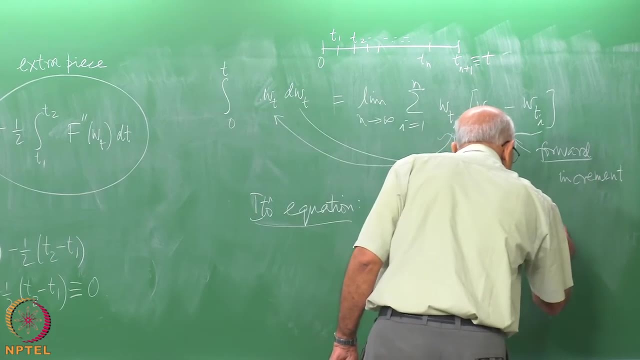 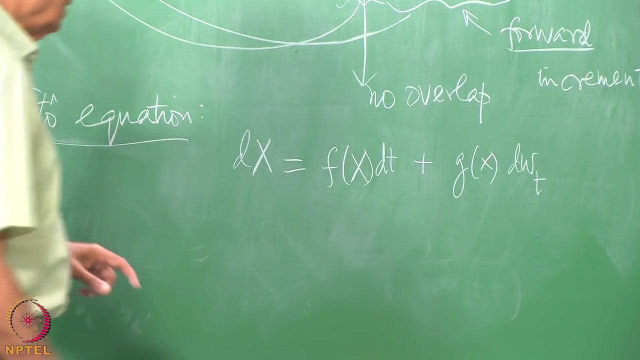 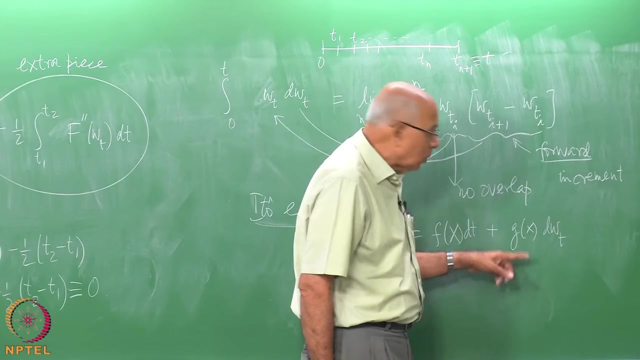 was a g of x times. we called it white noise and put this as x dot. but the correct way of writing it is with the d t here and this is d w in this fashion. This is an Ito equation. This is to be understood in the sense of Ito. So the x here and if it was time dependent. 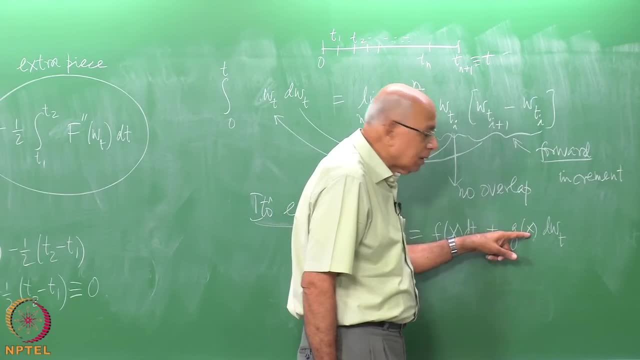 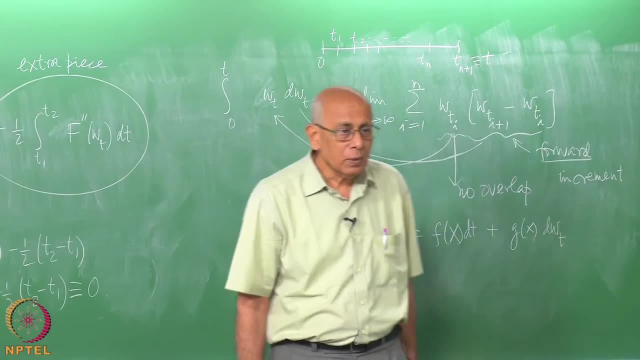 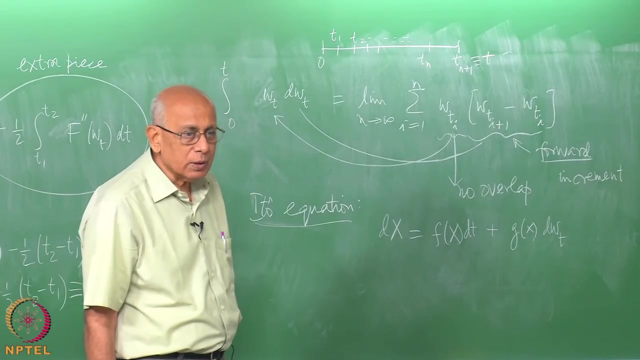 the t is such that this is the x at instant t and this is the forward increment in the Wiener process. okay, You need that interpretation, otherwise it is ambiguous. multiplicative stochastic process is definitely ambiguous. So the question is: you have a noise in physical terms. you 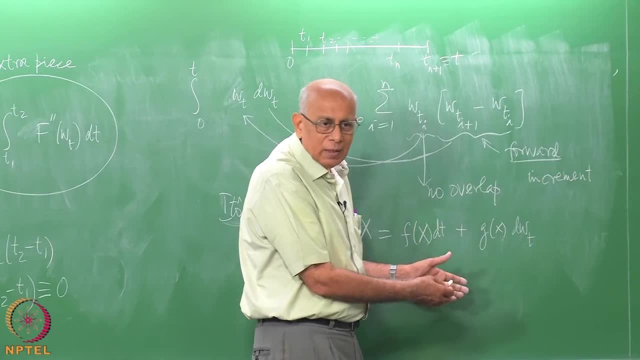 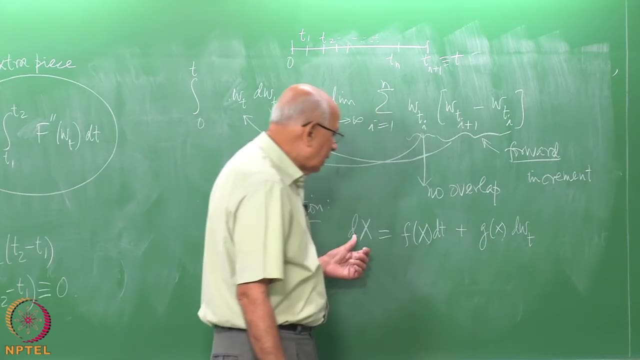 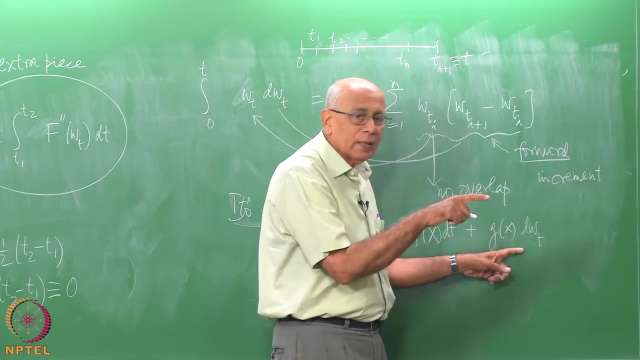 have a noise that is dependent on the state variable itself. The question is: state variable at what time? It is the state variable. when you write the increment in x, it is the state variable at time. t, where this d W, t is the forward increment between t plus delta t and. 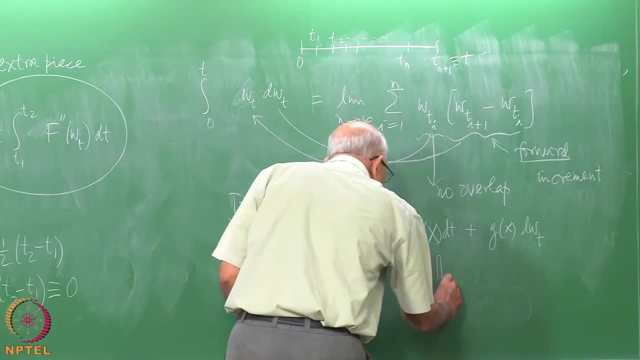 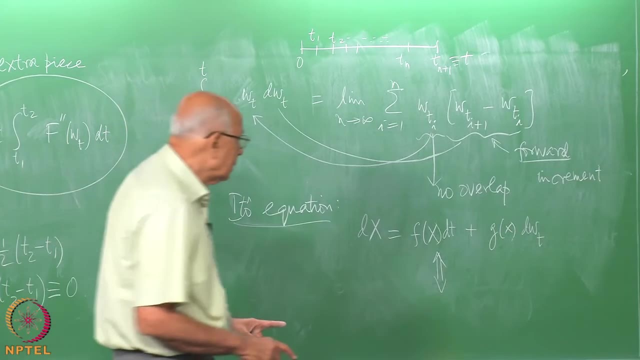 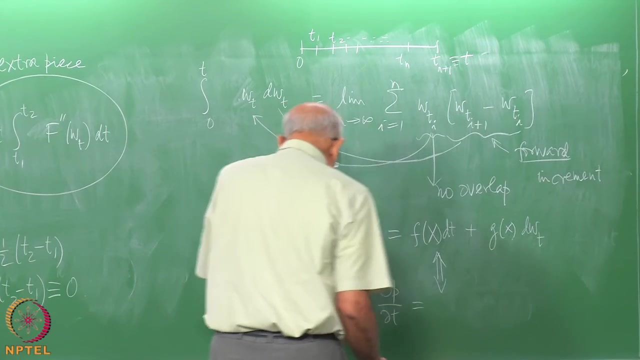 t. okay, Then this implies, and is implied by the Fokker-Planck equation that we wrote down for this process. It implies that the probability, then density, of this thing is delta p over delta t is equal to this fellow here, is equal to: 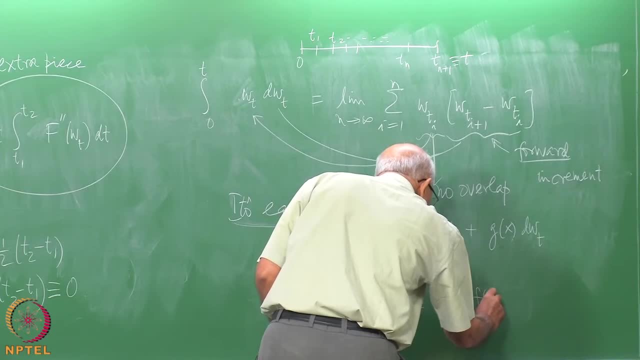 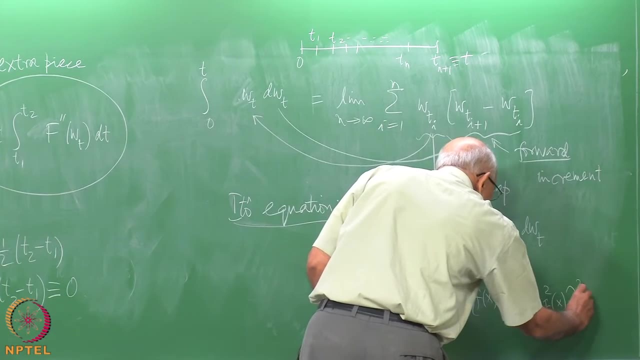 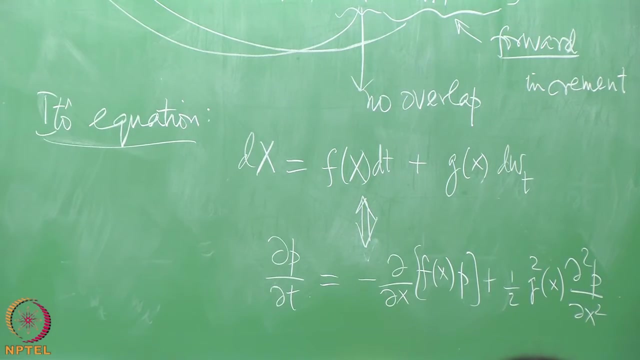 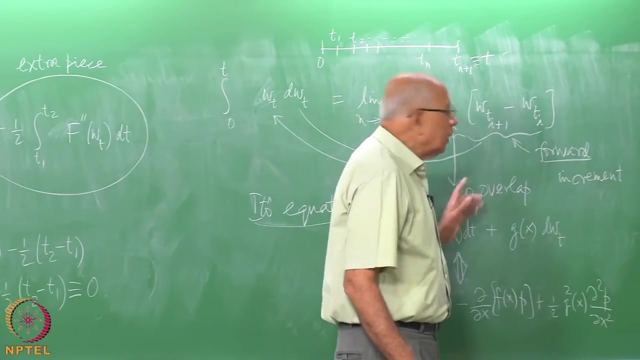 minus delta over delta x, f of x p, plus half g square of x, d, 2 p over d x 2. okay, So when you have a non- trivial noise, a multiplicative noise, you have to interpret it in the Ito sense. and 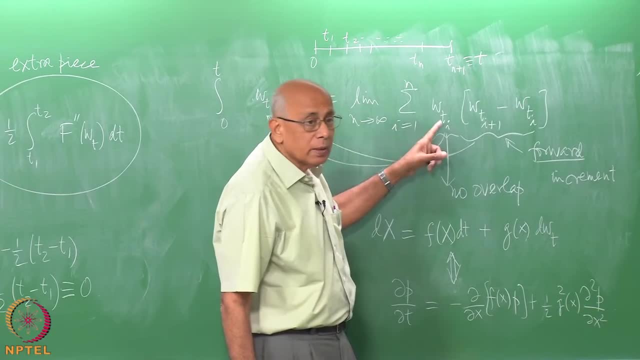 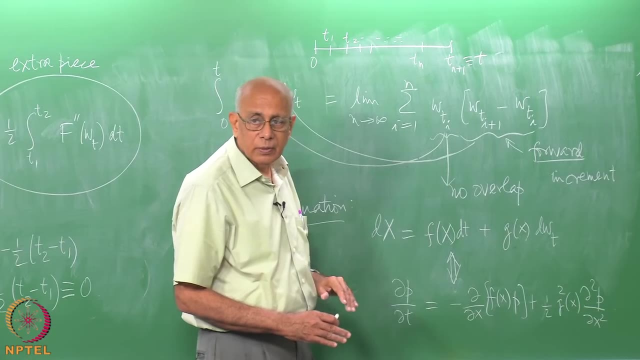 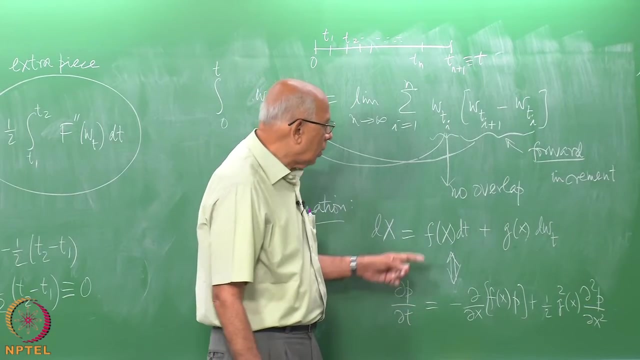 then this is true, The Statenowicz interpretation, where this would be t i plus 1, would give you a different Fokker-Planck equation for the same stochastic differential equation. interpreted in that sense, The point is that the physics has to be the same in both cases. 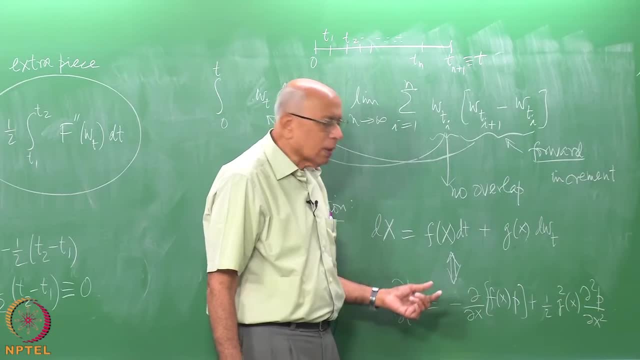 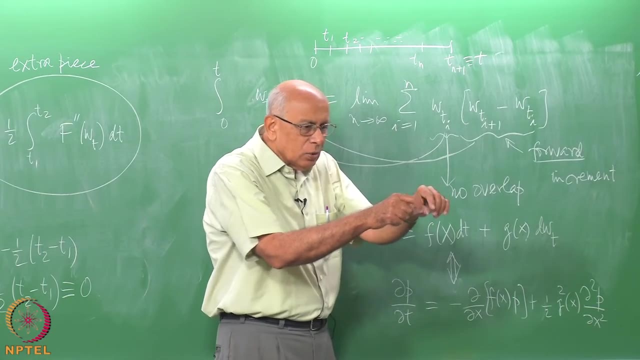 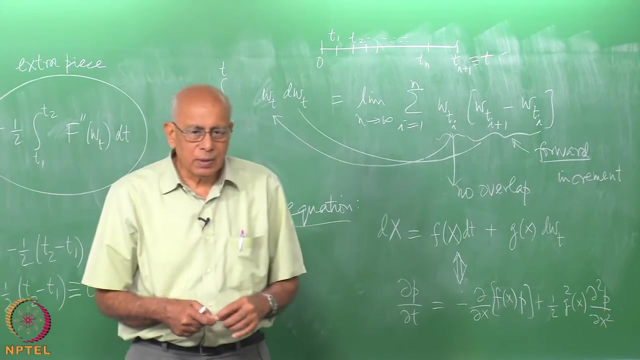 So what would happen there is that you would have what is called a spurious drift term. So in going from the, you go from the engineering equation to two different stochastic differential equations so as to get the same master equation once again for the random variable. because that 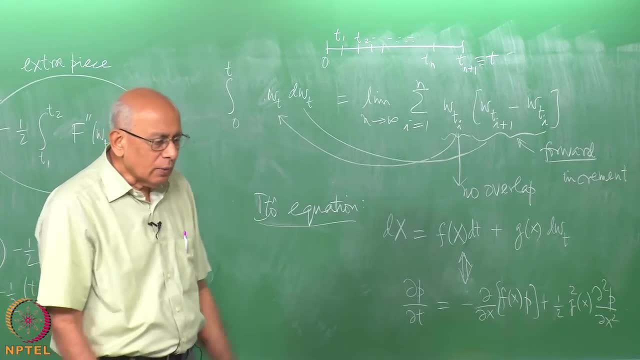 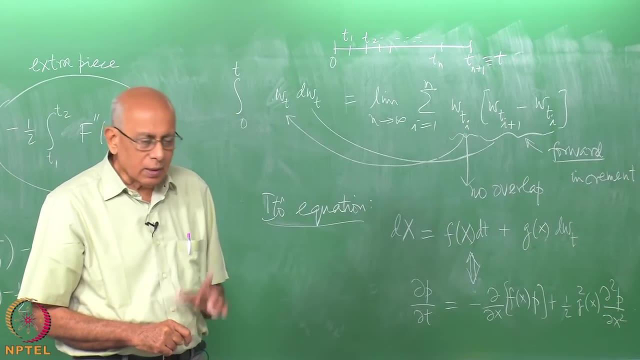 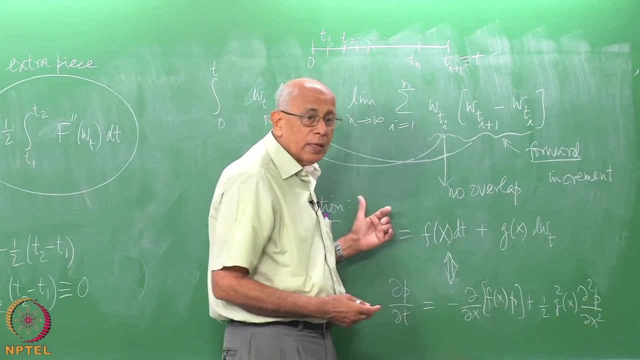 is, its moments are physically measurable. So you start with an equation between averages, the so called engineering equation. You add noise to it, If it happens to be stochastic, multiplicative noise. you have to then specify: is the equation this equation in the Ito sense? 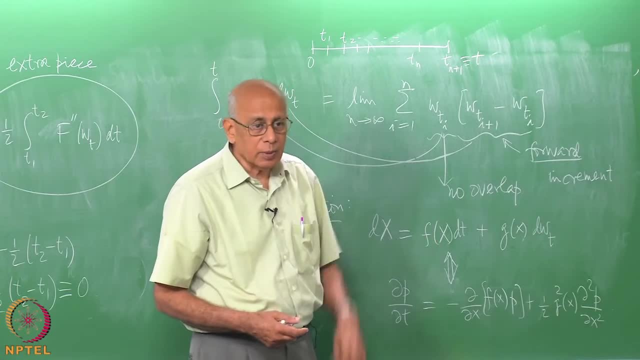 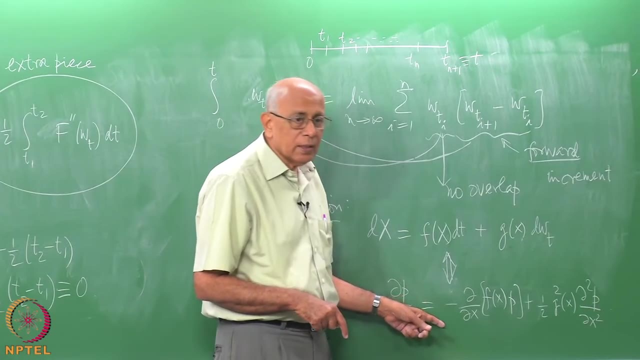 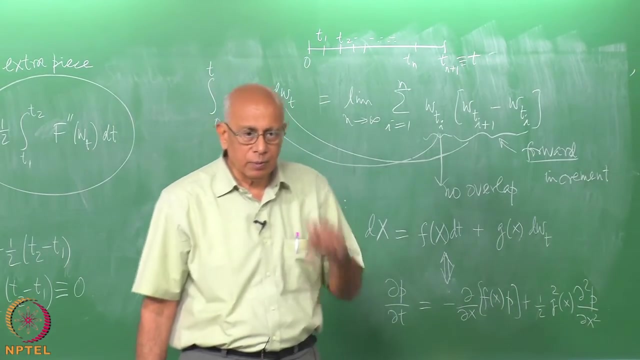 or in the Statenowicz sense or anything in between. there are other interpretations, and then each time the prescription to go from the stochastic differential equation to the master equation changes in such a way that the final master equation is exactly the same for a given physical process. okay, 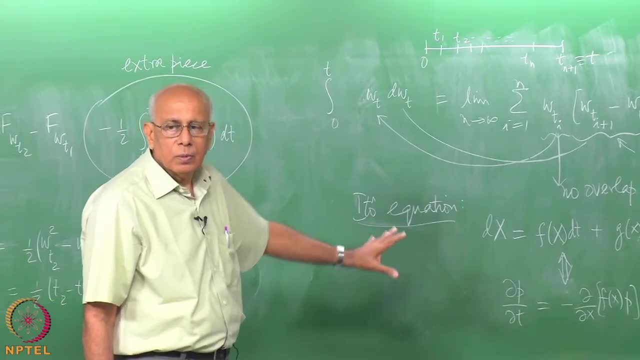 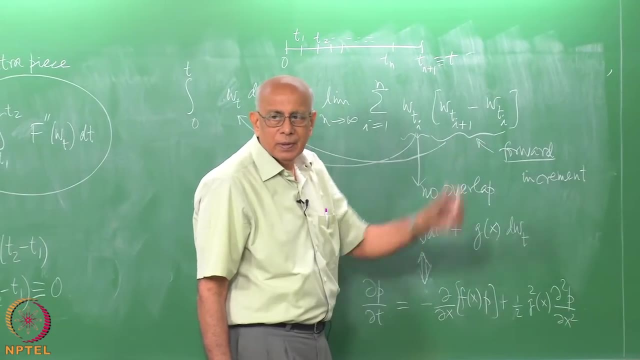 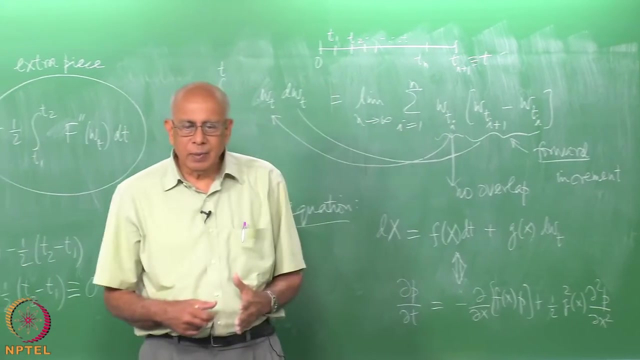 We have used, all the while I have used the Ito interpretation. It is sort of satisfying because of this That it is not anticipatory. 2, That is, the current dependence on the rate at the, on the state variable at the current time, and then the forward increment. Ok, But it is not sacred. it is not sacred, In fact. 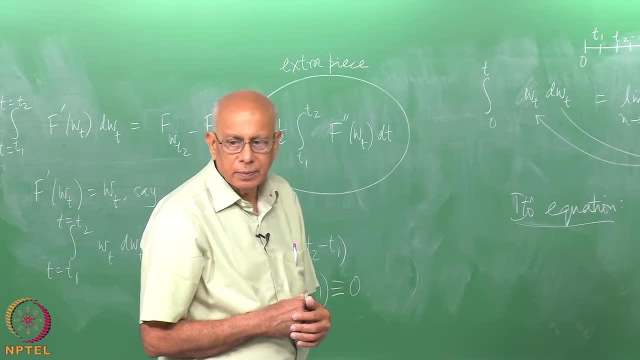 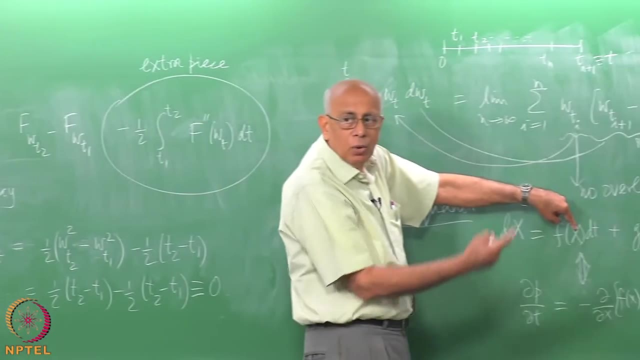 in physics very often one uses the Stratonowicz interpretation. Ok, But then you have what is called the spurious drift term. There is a correction to this fellow here and the prescription to go from here to the stochastic, to the Fokker-Planck equation changes in the 2 cases. 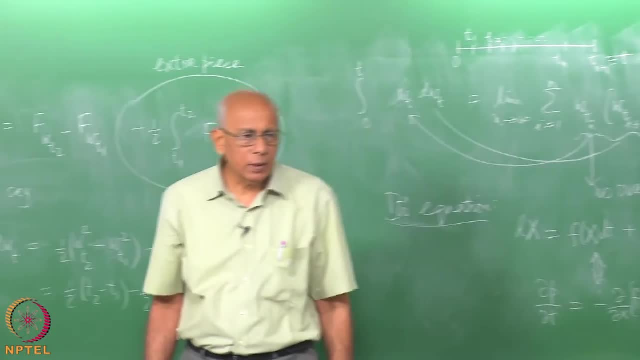 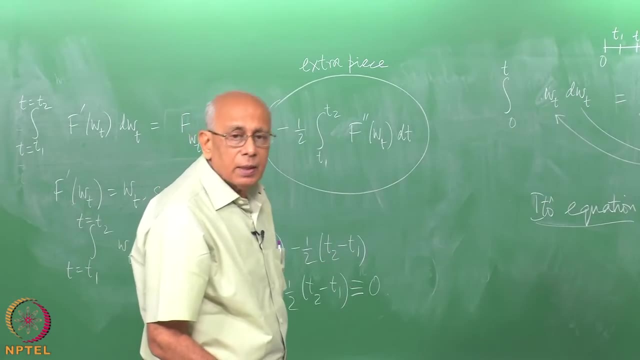 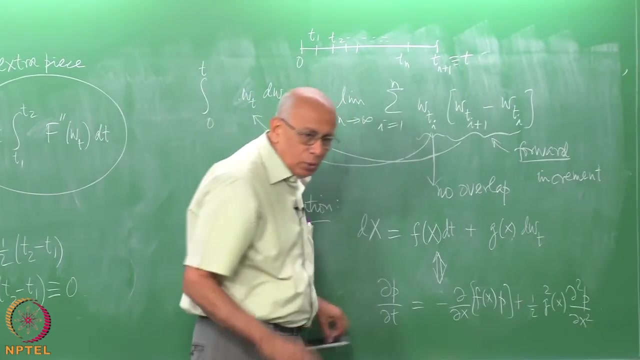 So you consistently use the Ito equation. Ok. Now, of course, if you, if you use the calculus carefully, then questions of uniqueness come for solutions of this process, questions of uniqueness arise, And here is an example, due to Ito himself, by the way. I should give a reference to this whole business. It's 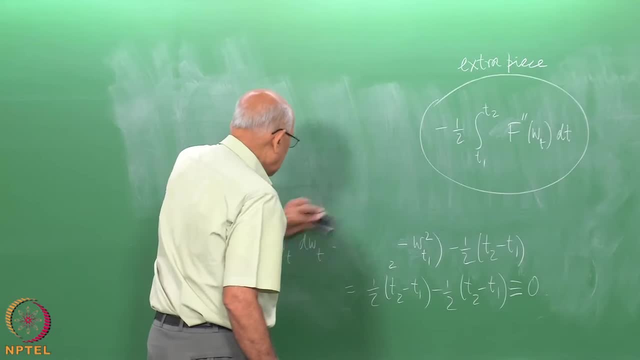 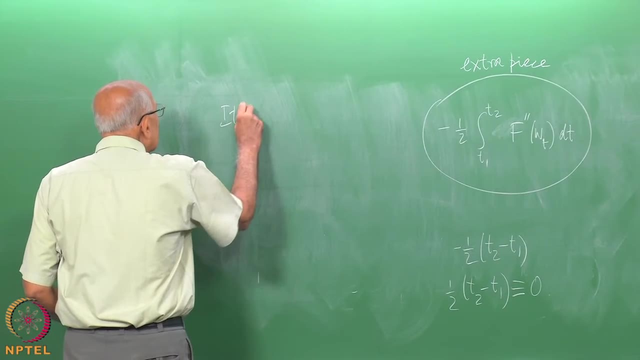 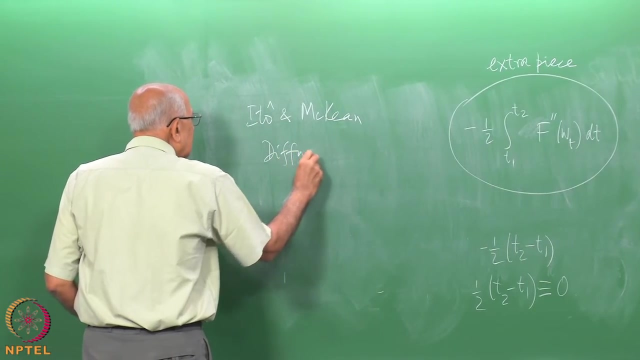 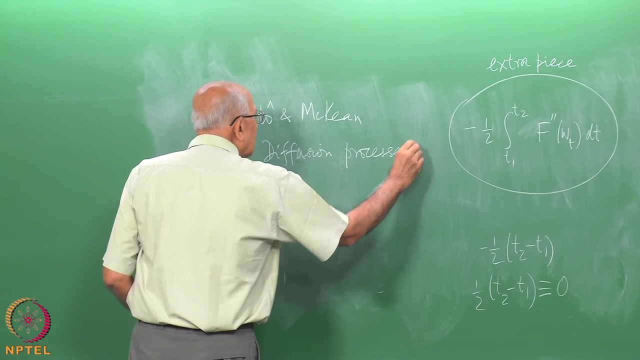 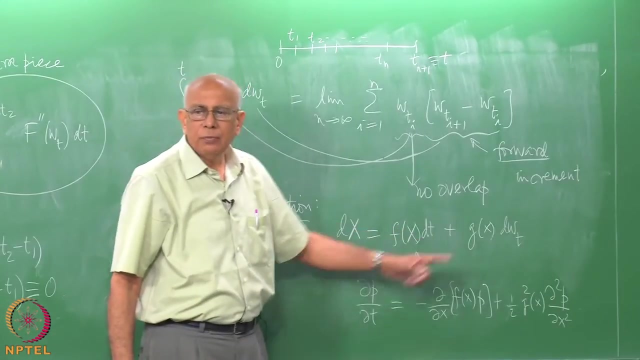 the mathematical treatment can be made very rigorous, and one of the best places for it is the original book by Ito Ito himself. so, Ito and McKean, it is called diffusion processes. Recall that. we called an equation like this a diffusion process. we called X a diffusion process. Ok, And you? 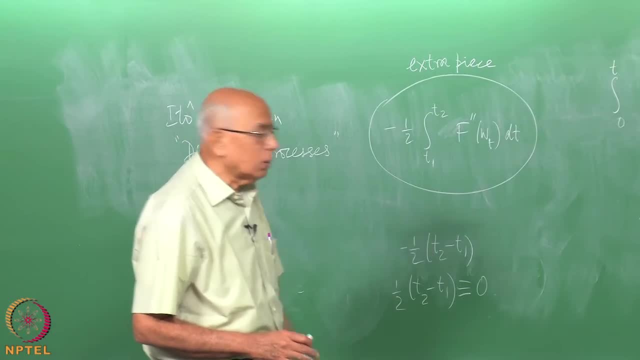 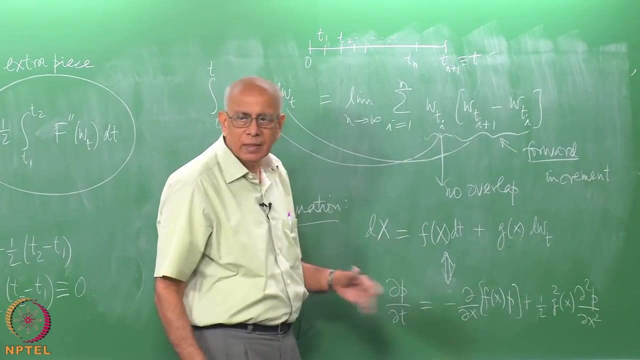 have to. you have to worry about the uniqueness of the solution to this sort of equation. We solved this for the on-screen Nuremberg case. it was completely trivial. this was a constant that one was linear in X, and then it didn't matter. we wrote down the solution. 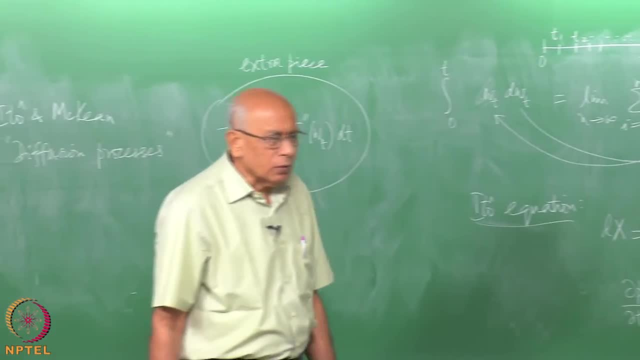 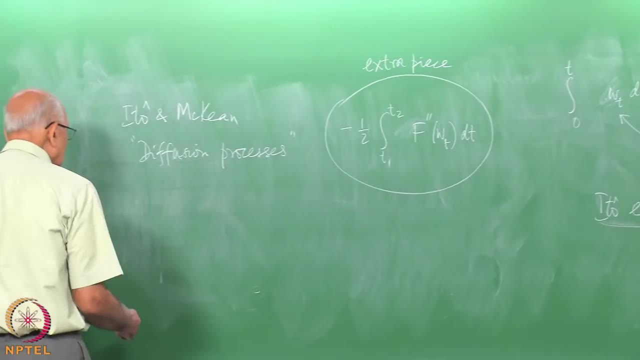 But if you do it rigorously, properly, then you have to be a little careful, because you could have non-uniqueness- And here is an example- due to Ito himself. We will work backwards to write the equation down. So if you have an example, this is due to. this is due to. 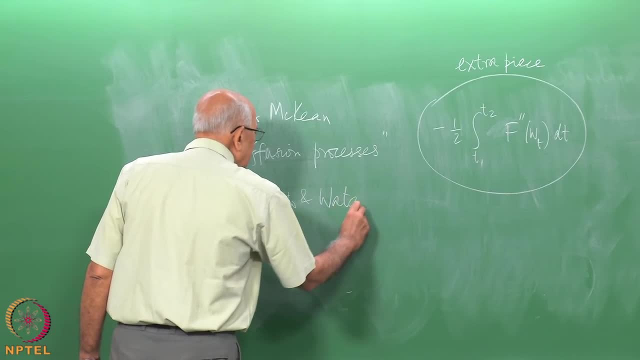 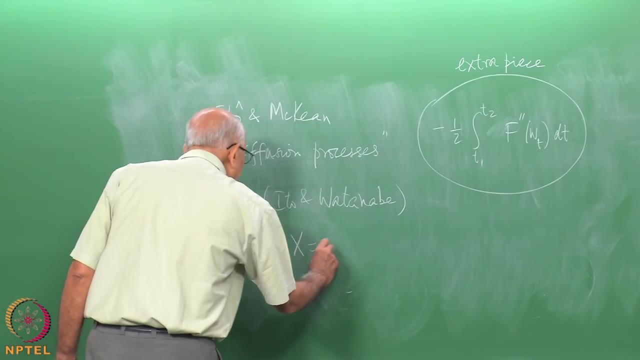 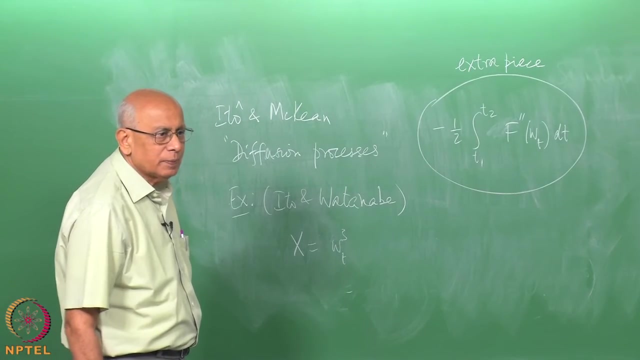 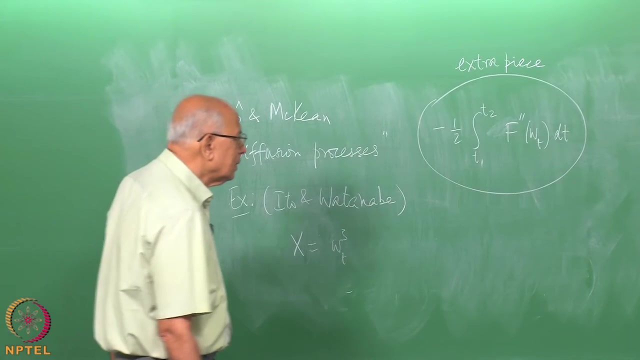 Ito and Watanabe. And the equation is the following: X equal to W t cubed, for example, It took. take this again: it is a nice functional of Brownian motion, right? Then what does the equation give you? It says dx equal to f of t, right? So this is the, this is the. 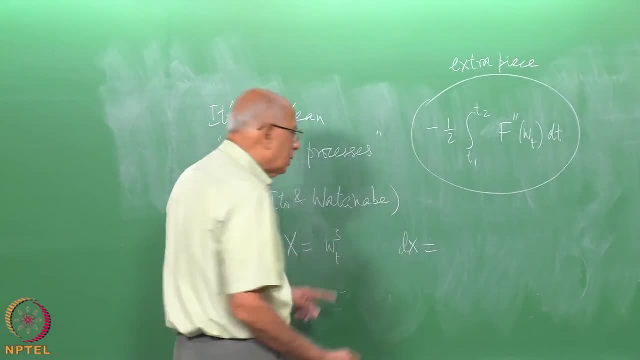 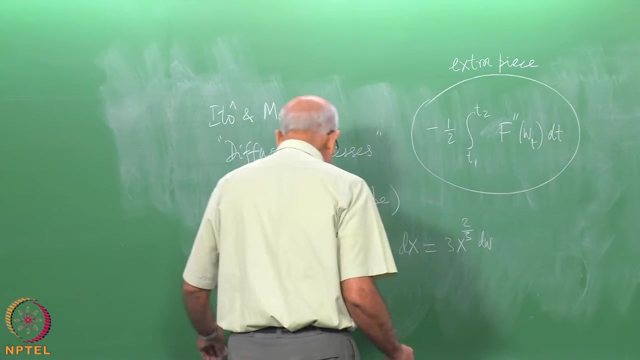 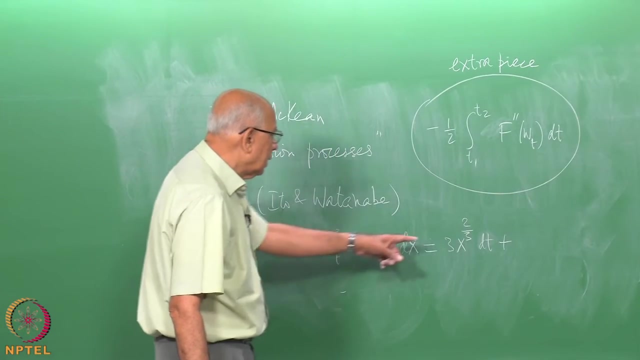 equation. So f of x, that is 3 W t squared. so it is 3 times x to the power, 2 thirds dW, dt plus the second derivative. you have to differentiate this. this is 3 x squared, 3 W squared and. 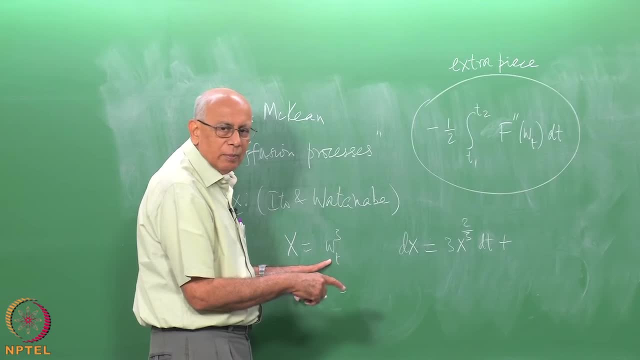 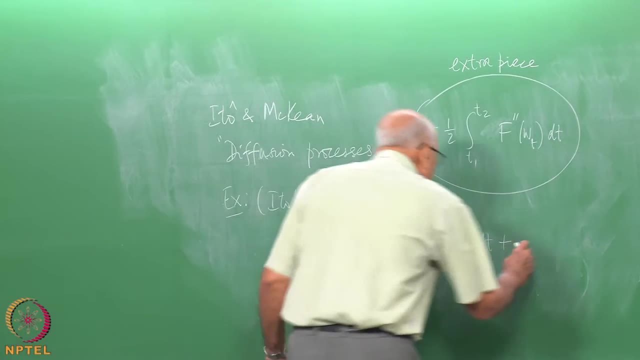 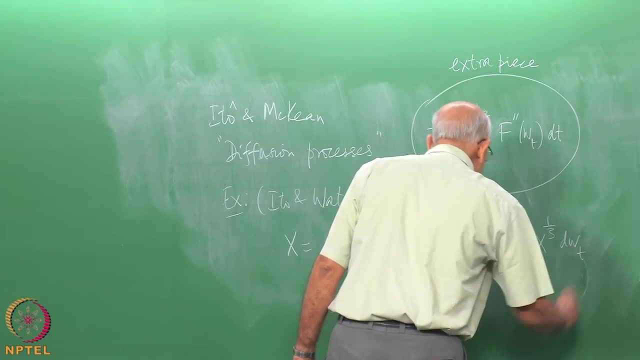 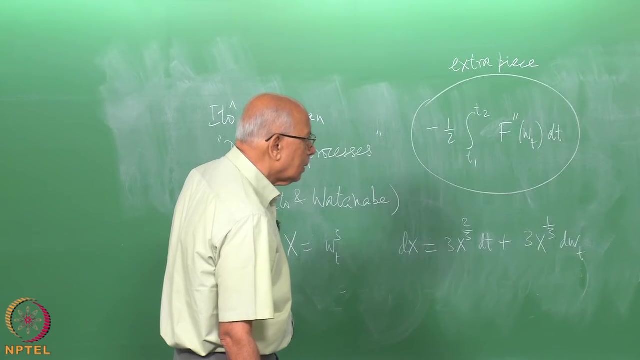 that is equal to 6 W divided by 2, and W is x to the 1 third and the 2 goes away in the second derivative. So get plus 3 times x to the 1 third, dW, t. Sorry, that is the coefficient of. how did 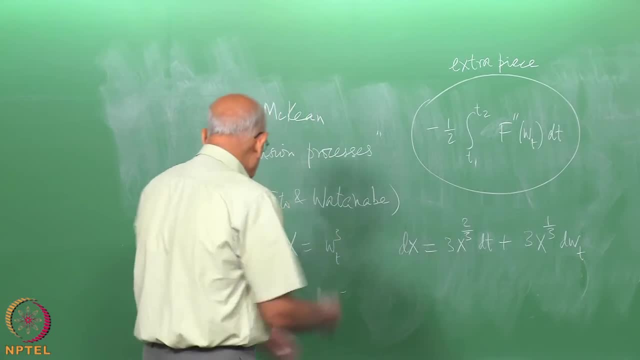 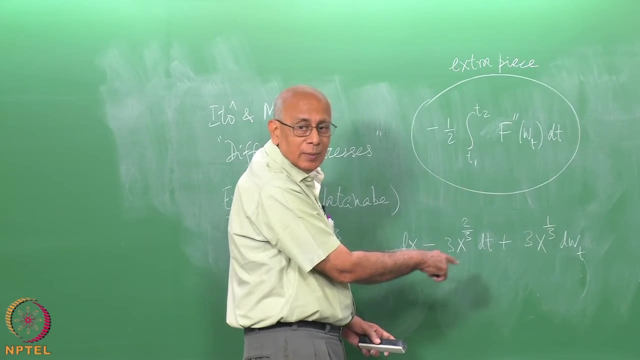 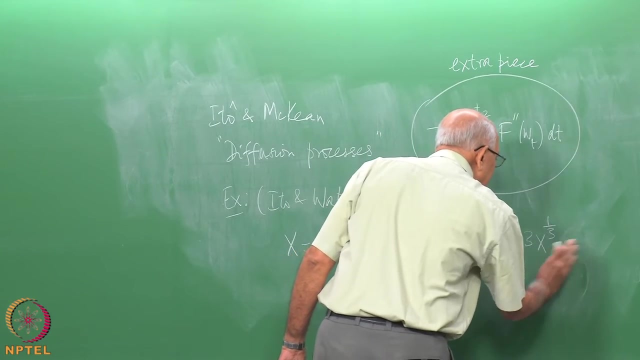 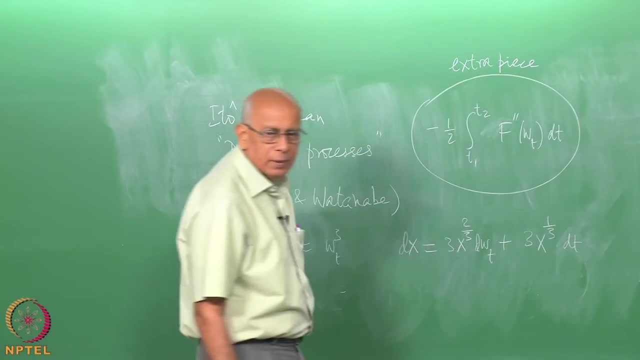 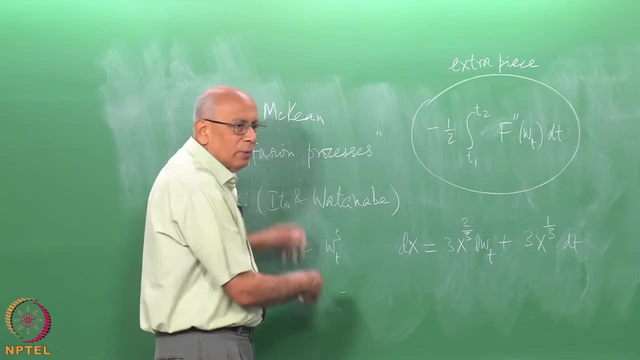 So it was. This is dt the correction part. So if I ask: what is the solution to this equation? we know this because we work backwards to get this equation. So if I ask: what process is this? x? you would say it is W? t cubed from this guy. 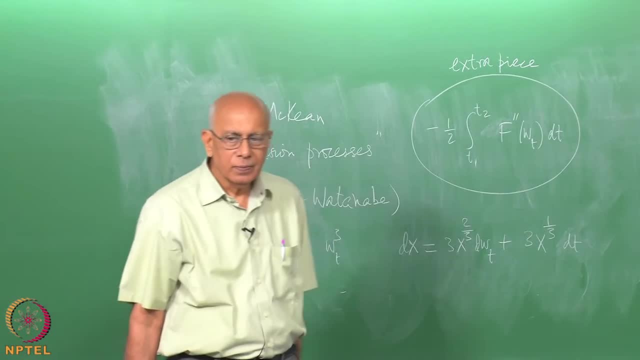 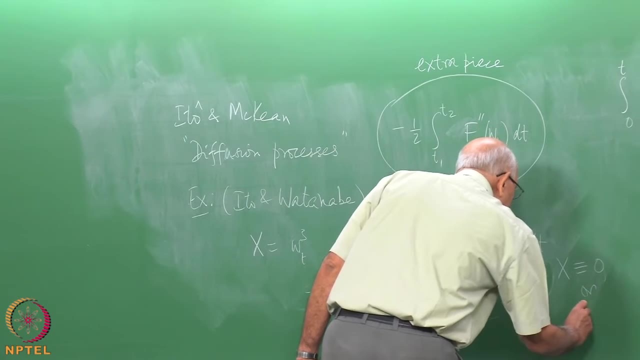 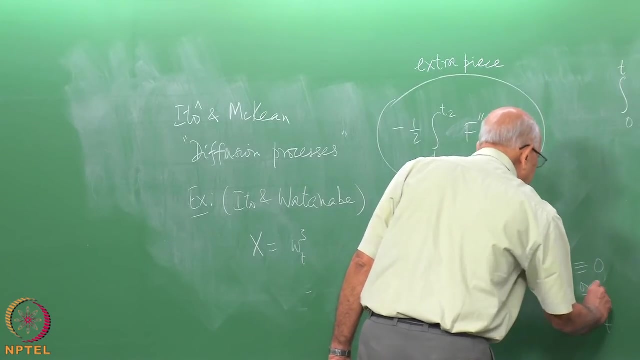 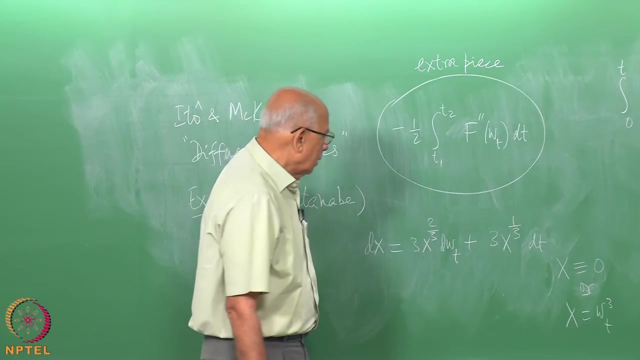 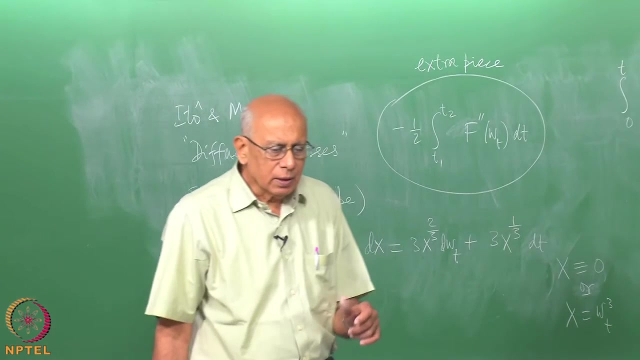 But you could put 0 there and it gives you a solution. Ok, So you have this or that. Therefore, the uniqueness of solutions is not guaranteed. Fortunately, this is a kind of academic example. fortunately, it turns out that if you put in sufficient, 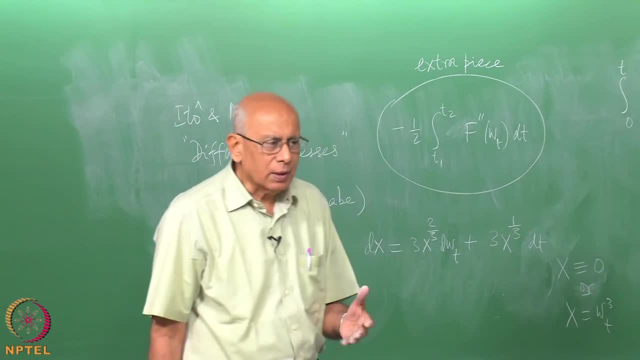 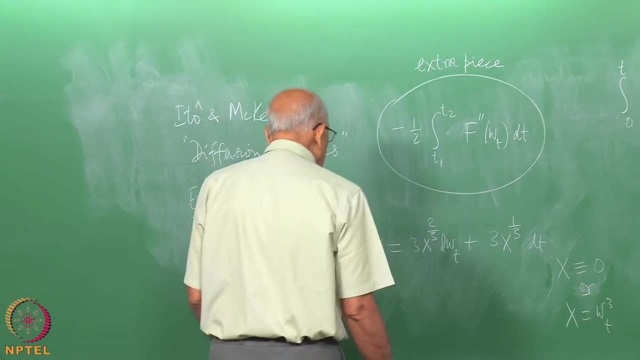 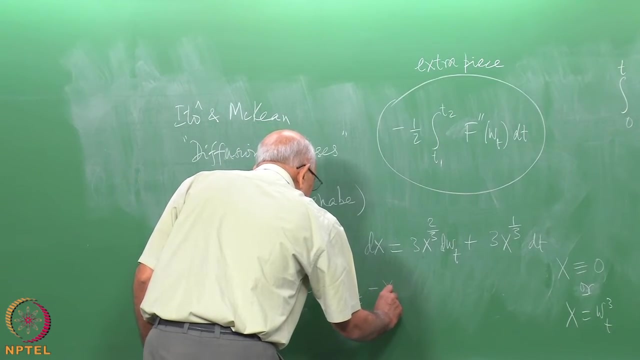 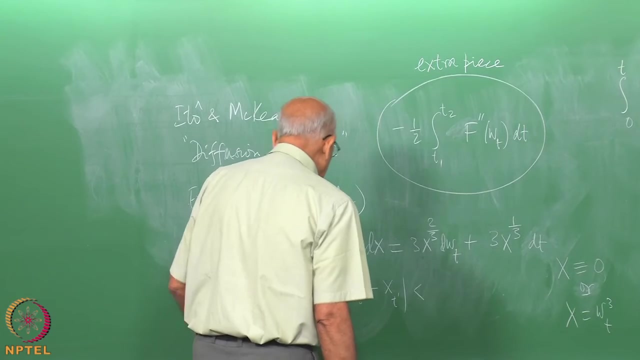 holder conditions on the continuity of this process, then you get unique solutions. For instance, if you can show that mod x at some time, t minus x at time, t prime is less than sorry the function. So if this fellow is some function x of t, 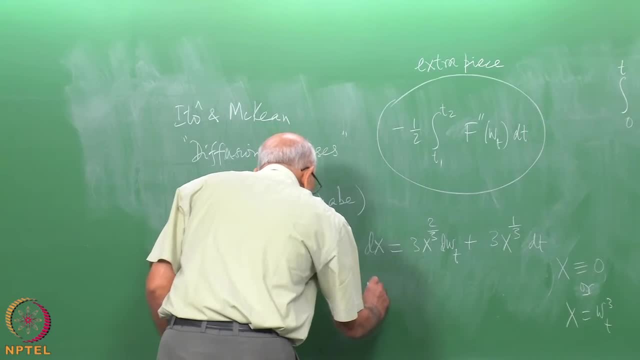 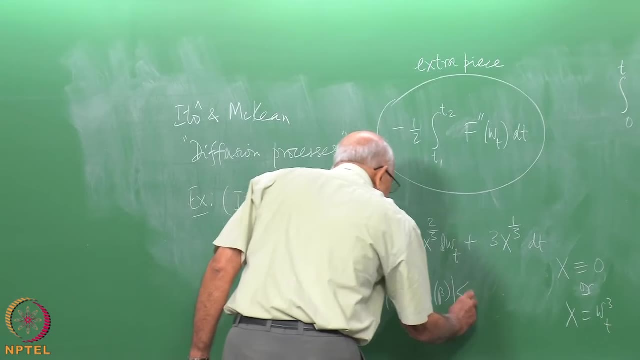 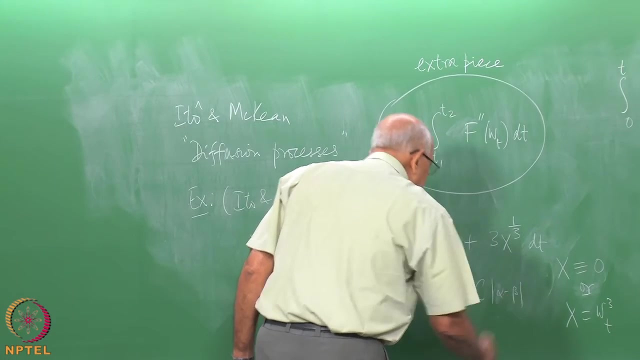 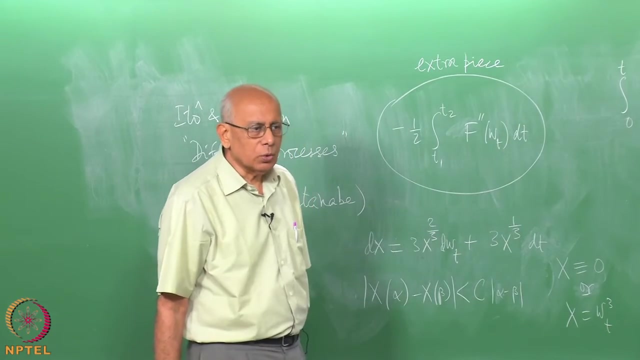 If you can show that x of in some alpha minus x of some beta modulus is less than some constant times modulus of alpha minus beta, for all alpha and beta, all argument, then that suffices to show that the solution is unique. This is not. this doesn't satisfy that. 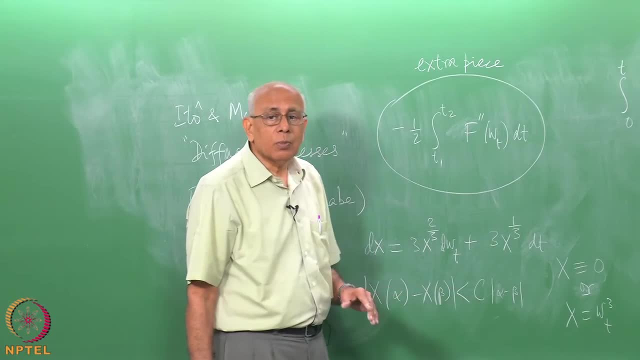 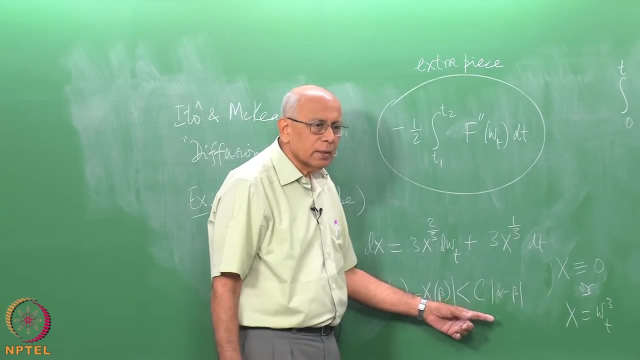 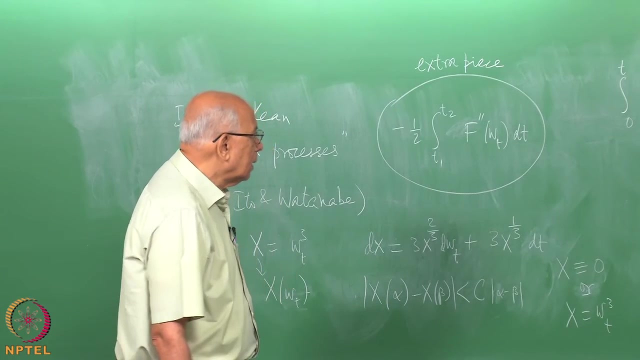 These two guys are not smooth enough at the origin, They are too singular at the origin. But if you have something milder like this, then the solution is unique and that is what happens in most physical examples. Now you can ask: can this whole thing be generalized? 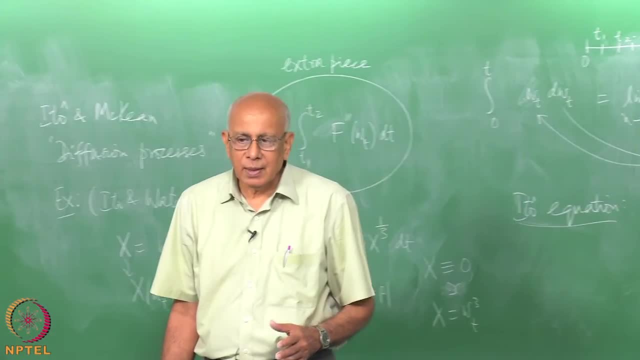 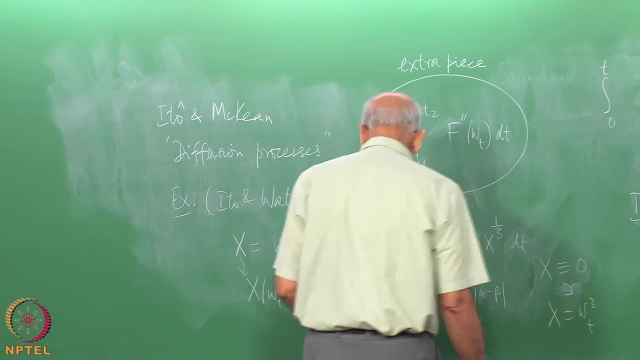 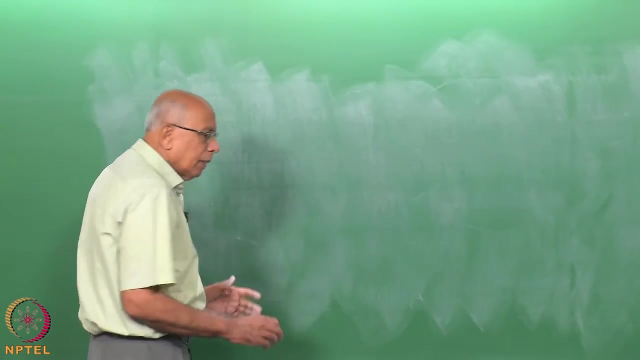 But before that, let me point out- I think I have run out of time, but I should point out This is what Descartes formula is, at the very least. Ok, This requires a bit of a preamble, Let me. let me again motivate this on physical grounds. So let me give a little preamble. 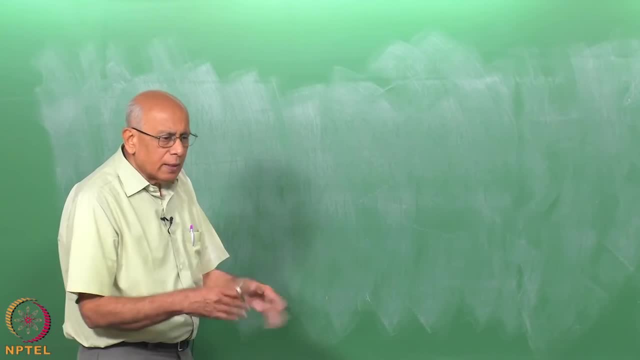 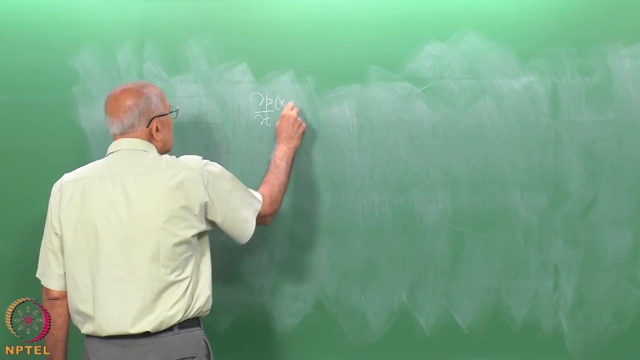 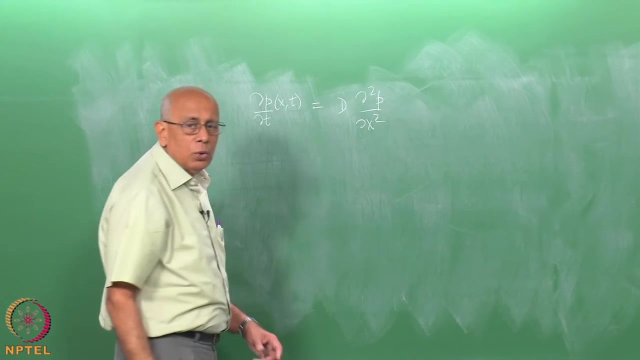 to this. Recall that the original diffusion equation, so let's write it in the physics notation. Our original diffusion equation was of the form delta p over delta t for the position of a Brownian particle: d, d, t. Ok, And you can ask what's the solution to this equation for some given initial distribution. 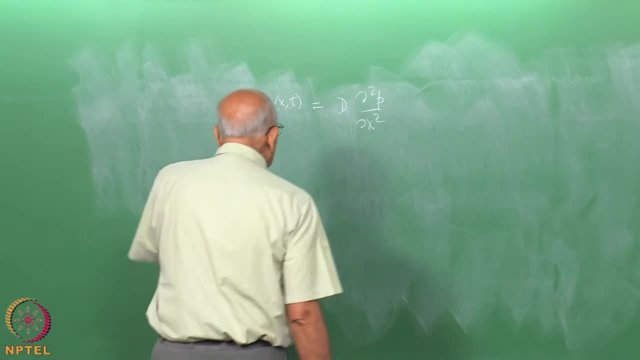 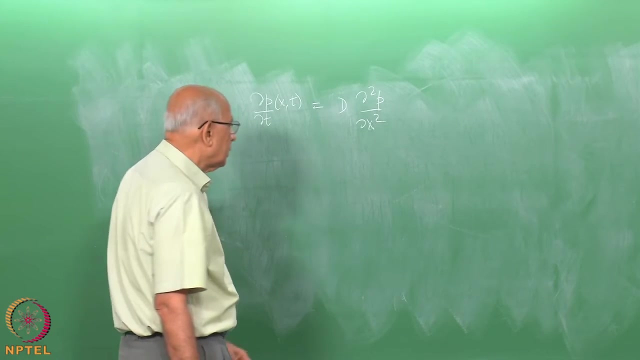 not necessarily a delta function. Then of course you take the original Gaussian solution, use that as a kernel for the green function for the operator differential operator, and you integrate over the initial distribution, whatever it is. So you would write the solution: p of x, t equal to 1 over delta, p over delta t. 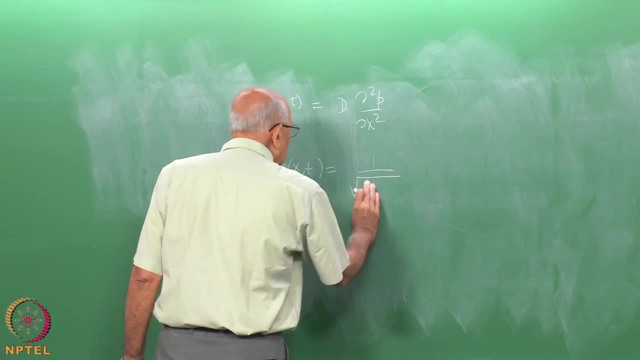 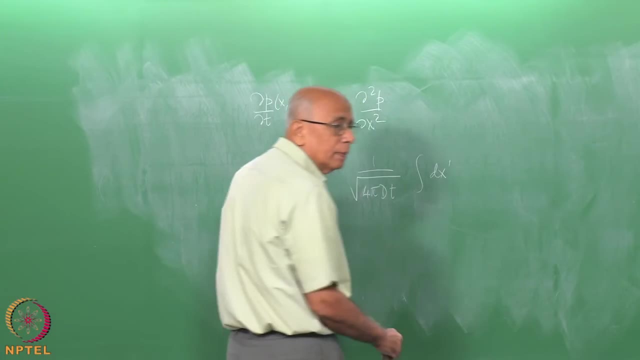 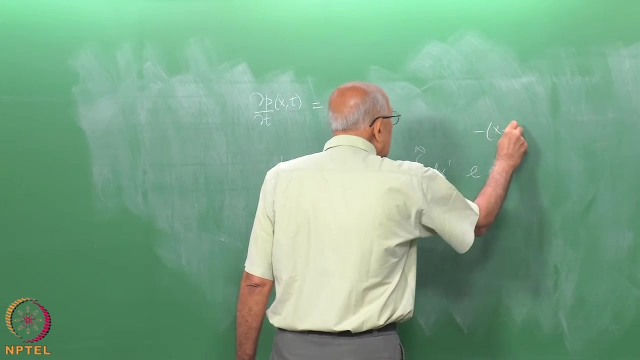 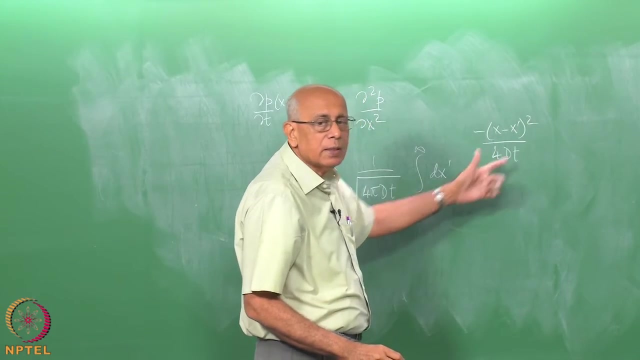 Ok, This is equal to 1 over square root of 4 pi d t. an integral d x prime over all x prime, infinity e to the minus x minus x prime whole squared over 4 d t. You could have started at any point, t minus t, not in the initial time. You could have replaced this by t minus. t not. So we are talking about processes starting at any point- t minus t, not in the initial time. You could have replaced this by t minus t not. So we are talking about processes starting at any point- t minus t, not in the initial time. You could have replaced this by t minus. 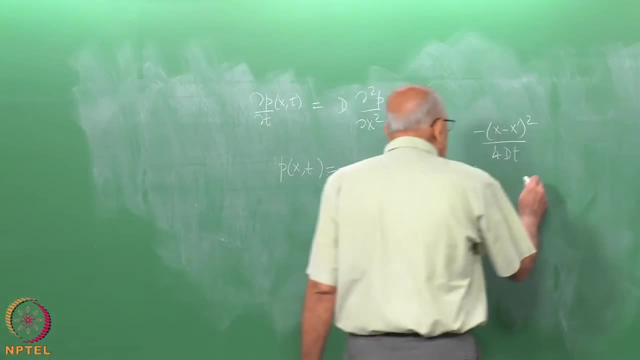 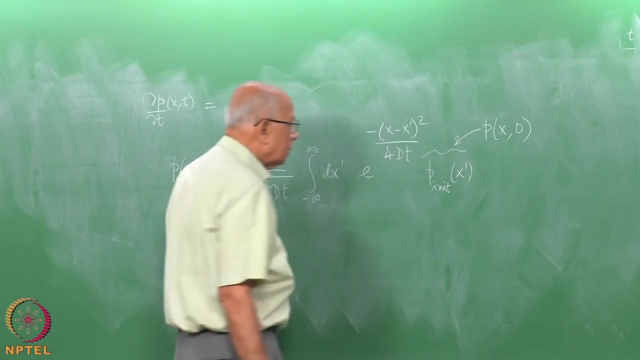 t, not in the initial time. So we are talking about processes starting from the specified at x equal to 0. This multiplied by p, whatever be the initial of x prime, This was p of x at 0. Ok, It acts as a green function here. Now the Schrodinger equation for a free particle. 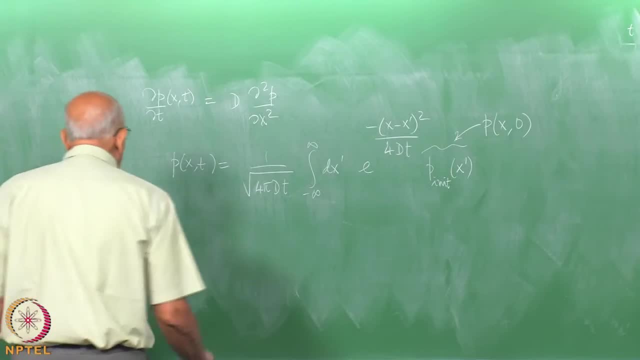 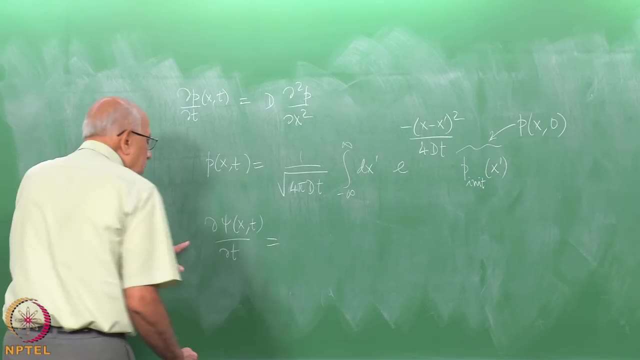 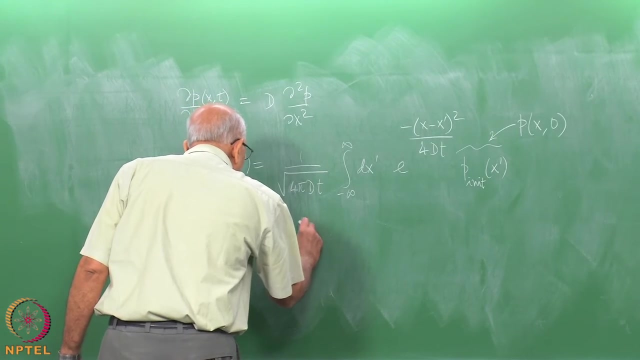 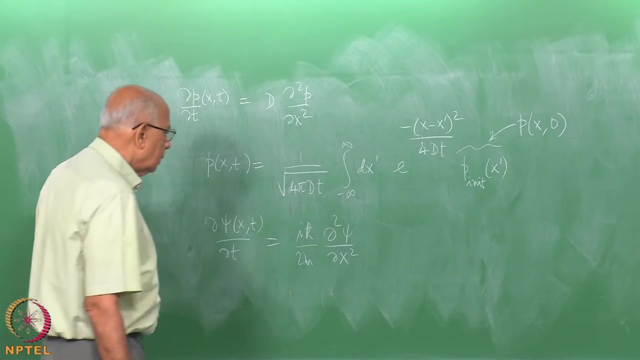 has exactly the same behaviour. Ok, Right, Ok. Psi of xt over delta t equal to ih cross times. that is minus h cross squared. so write that as minus ih cross whole squared. so this is equal to ih cross by 2m d2. Psi over dx2.. 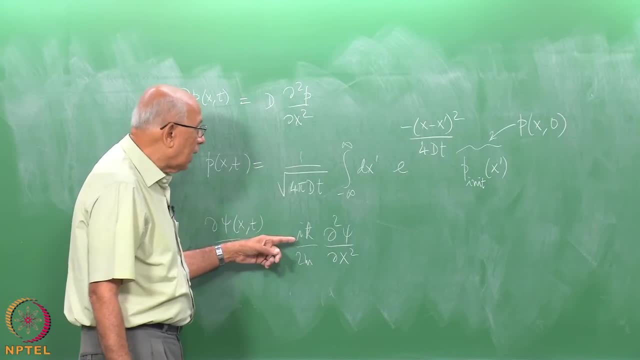 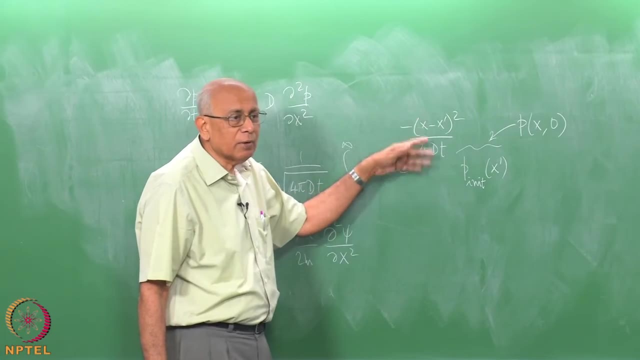 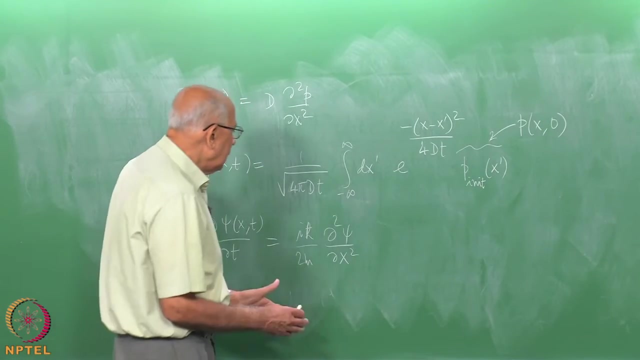 This 2 has a similar solution, except there is this i, so it is as if the d were an imaginary quantity. and then it is not clear if this is an oscillatory function. in that case it is not clear if this thing converges. but formally, if you do a wick rotation here in time go. 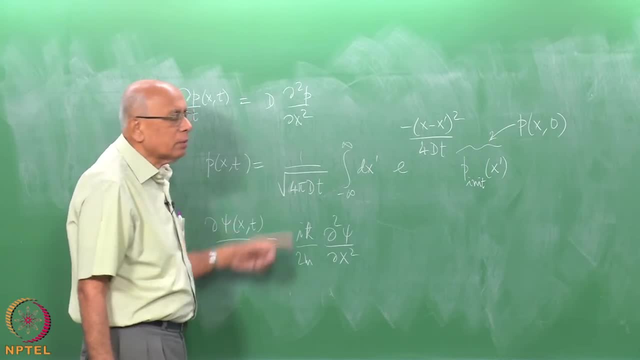 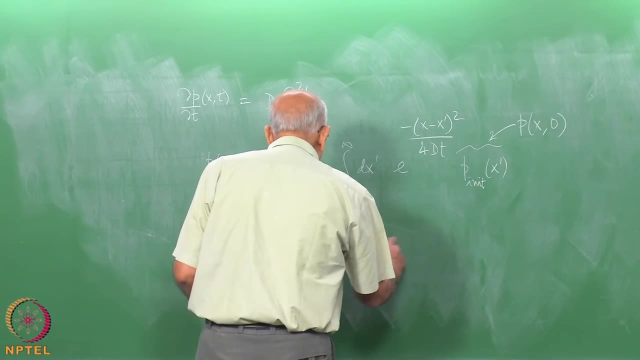 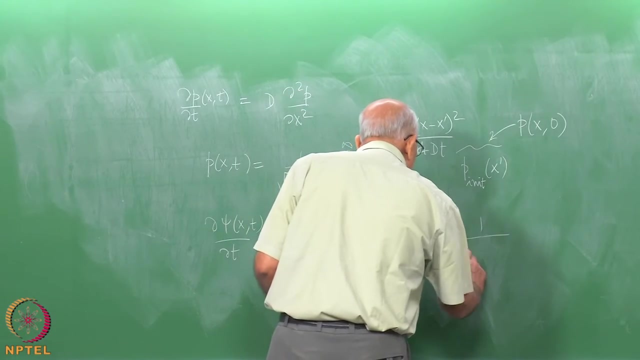 to imaginary time. i times t, then the 2 problems are mathematically equivalent and well defined, So you have exactly the same sort of solution. This would imply that Psi of x, t is equal to 1 over square root of 4pi, and then instead: 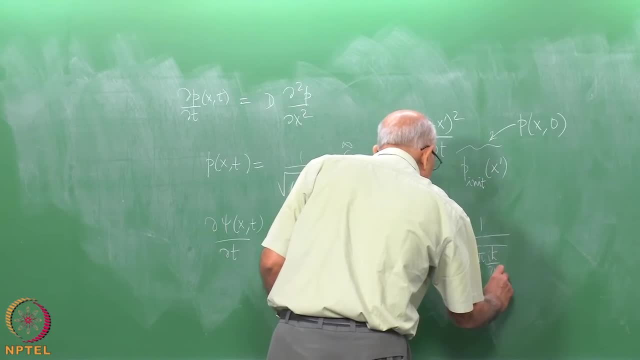 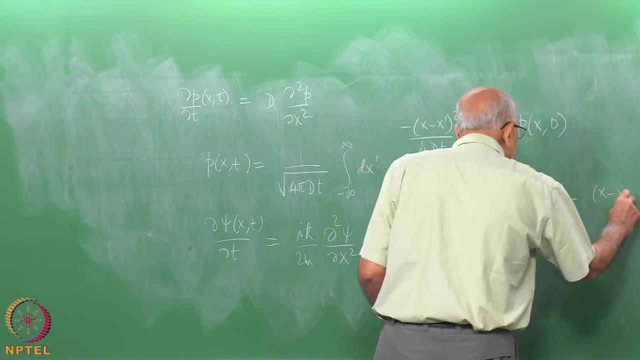 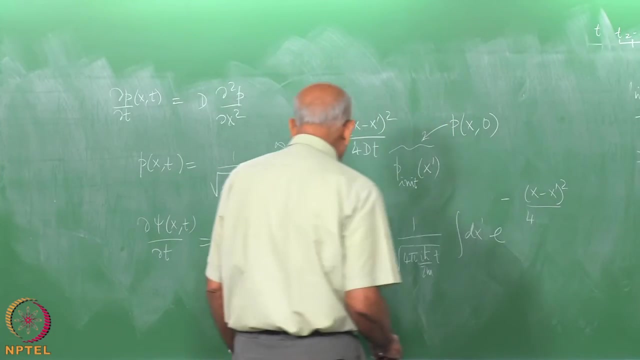 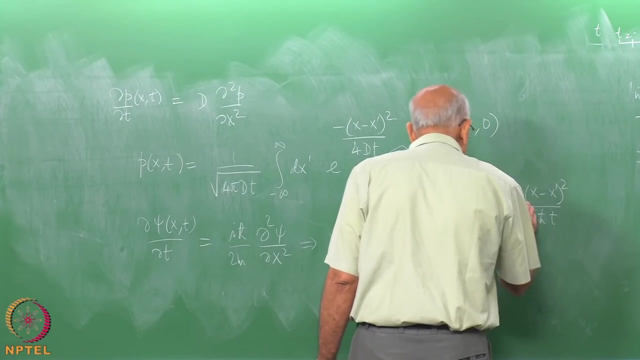 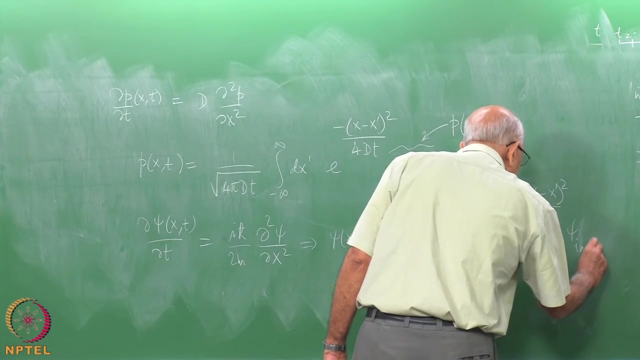 of d, you would replace it by ih cross over 2m t integral dx prime e to the minus x, minus x prime whole squared divided by whatever it is, 4 times d. What is this? So twice 2 ih cross t and then an m or something like that times Psi initial of x prime and. 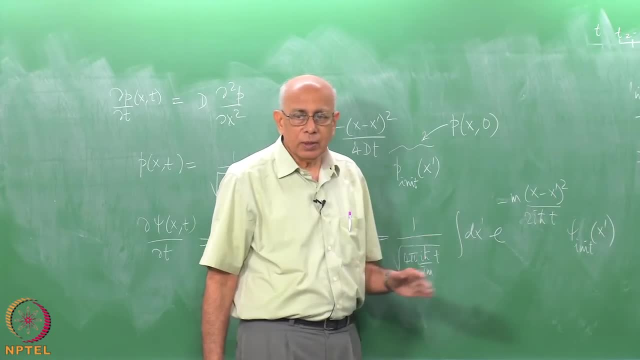 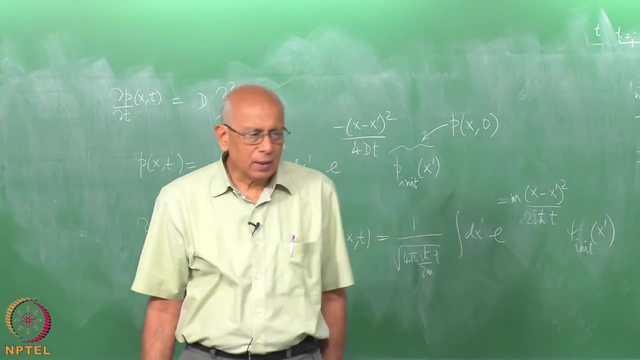 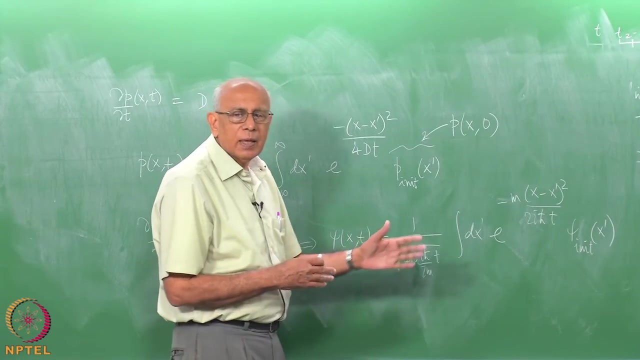 if you recall, this is the starting point of the path integral formulation of quantum mechanics. Then you do time slicing and stuff like that and you get the path integral formulation of quantum mechanics right Now. Mark Katz noticed this and said: now this operates in 2 different can give a form gave. 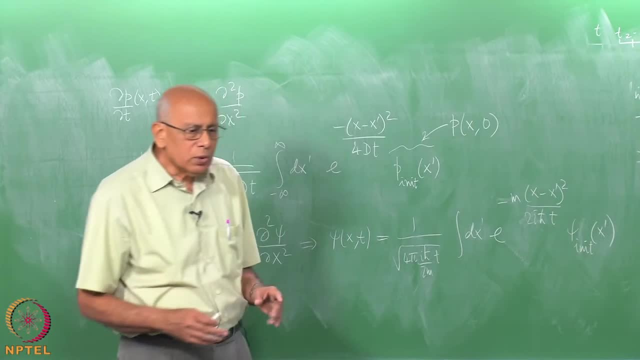 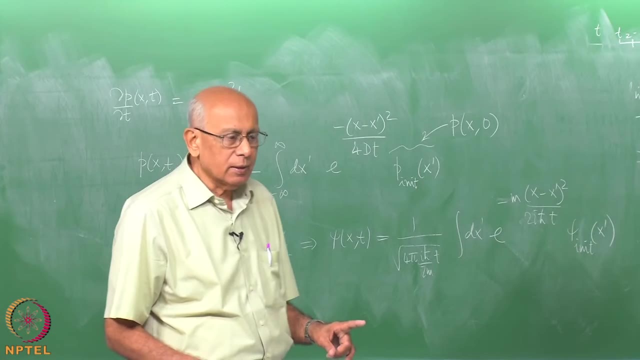 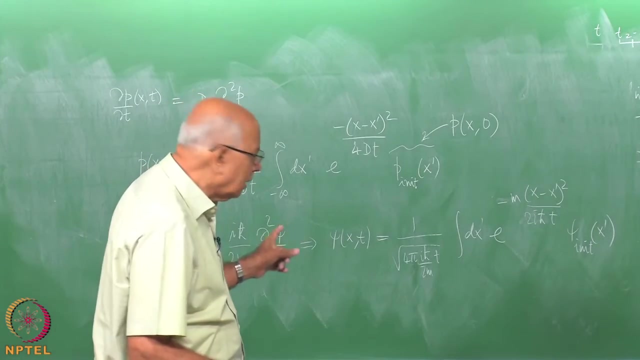 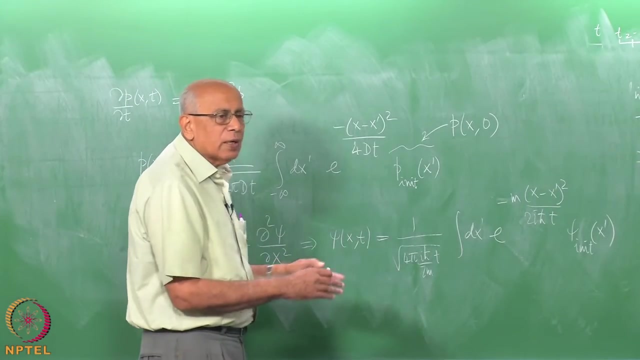 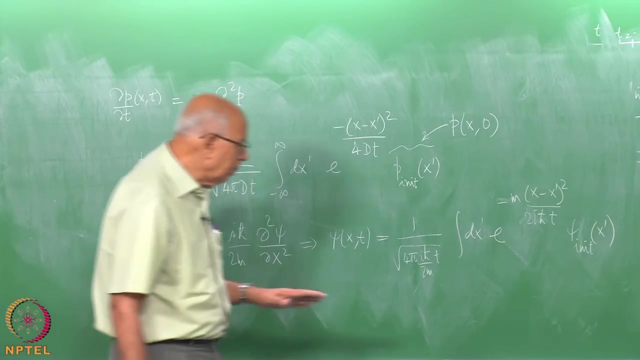 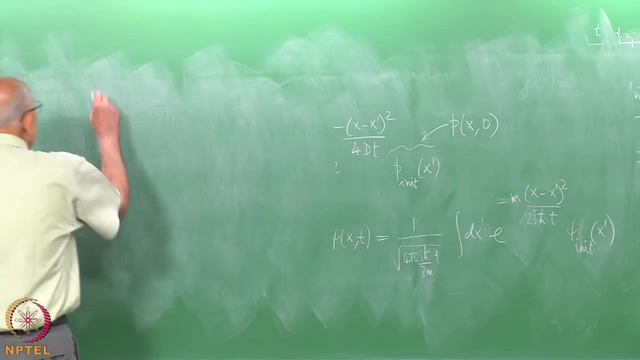 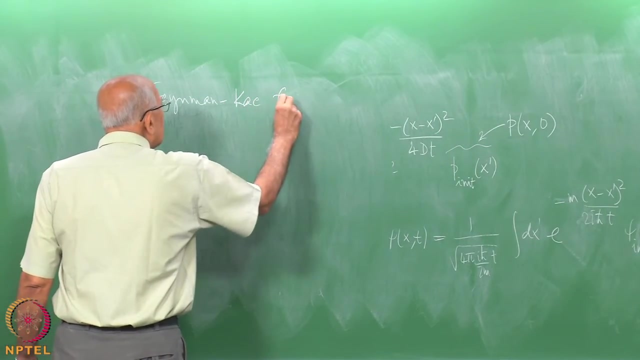 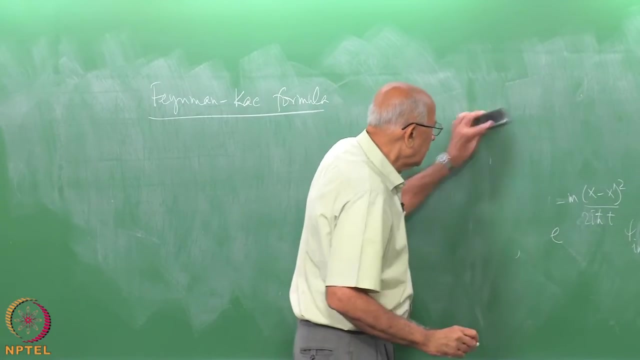 a clever formula which essentially says that you can use this fact, the fundamental Gaussian solution, in order to write down solutions to some deterministic equations or, conversely, starting with the deterministic differential equation, which is essentially the diffusion equation, with a potential term on it. It is got all kinds of generalizations, higher dimensions, etc. but here is what it looks. 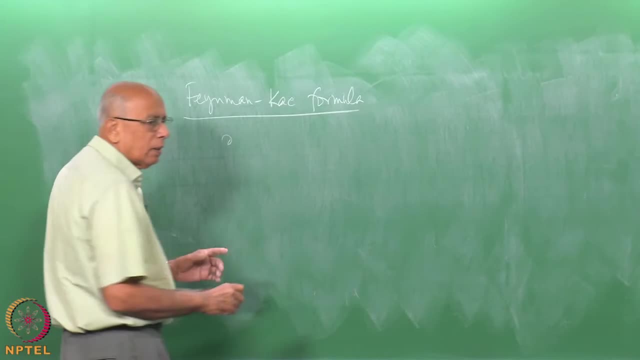 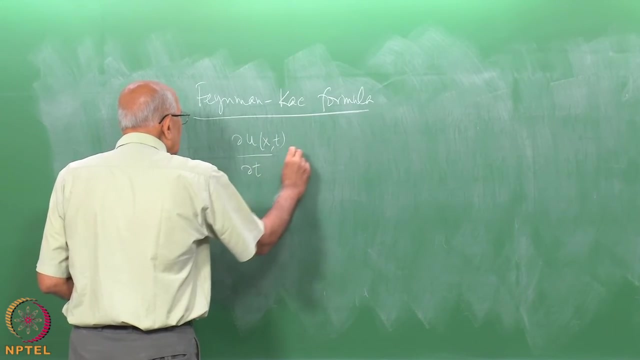 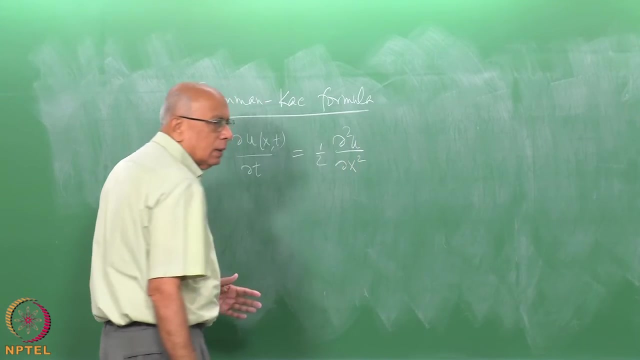 like. Suppose you have a partial differential equation, a parabolic partial differential equation in one space dimension and one time dimension equal to. let's write the standard diffusion equation down. Ok, This is the PDF of a Wiener process, if you like, but along 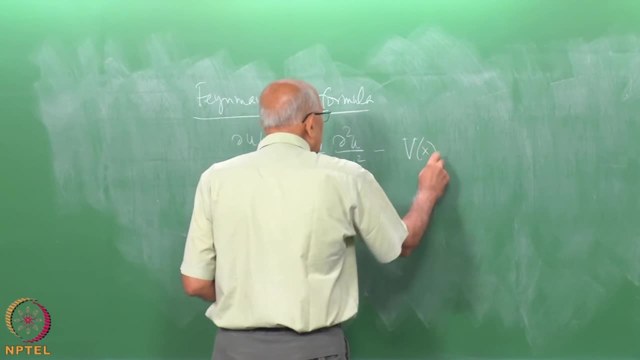 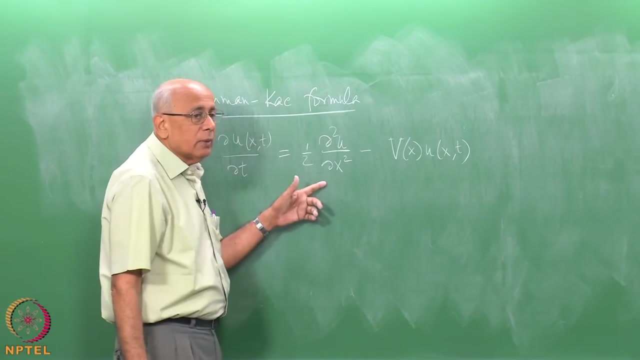 with that. let's suppose there is an extra term v of x times u of x comma t. If this were the heat conduction equation, it is like there is some external cooling which is state dependent, x dependent here or in the context of the Schrodinger equations, like a potential. 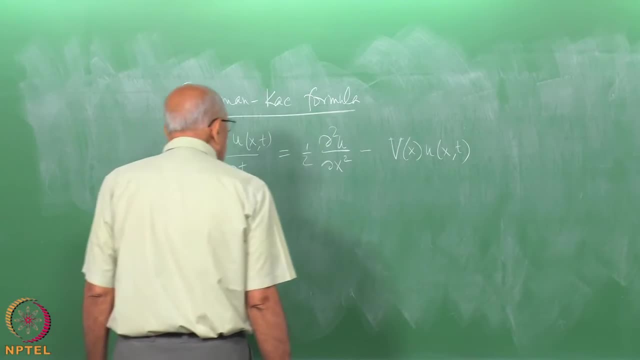 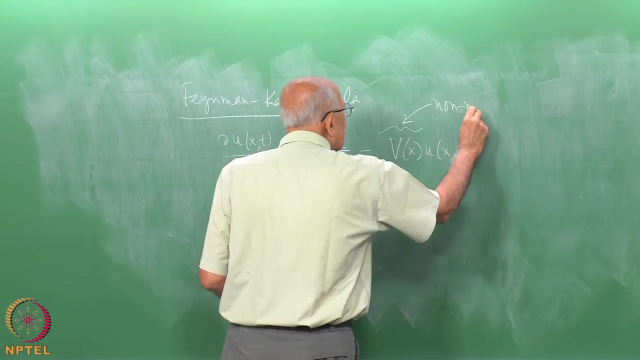 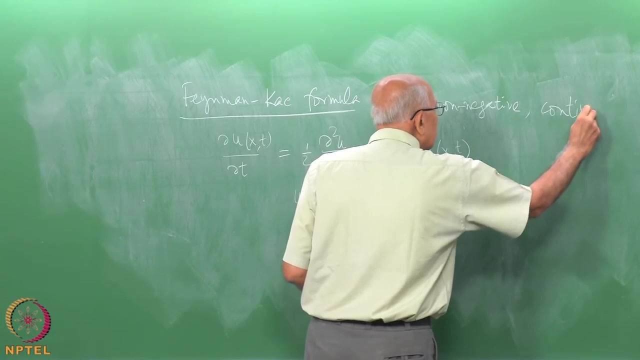 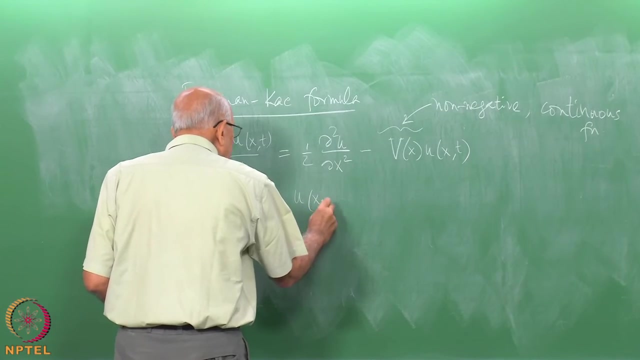 somewhere. Then the question is: what is the solution? You have to specify an initial condition, And the initial condition is, so some conditions are put on this. this is a non-negative continuous function And u of x- zero is equal to some specified initial function. So this is U, not of x, and 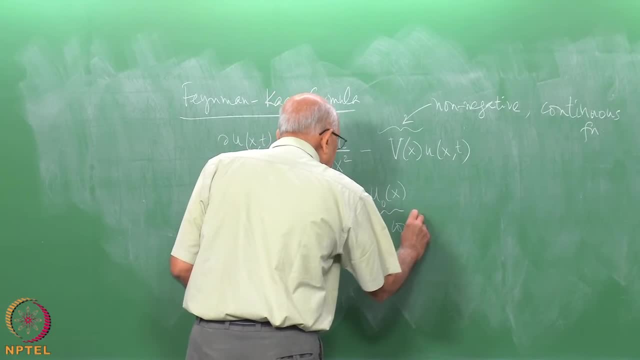 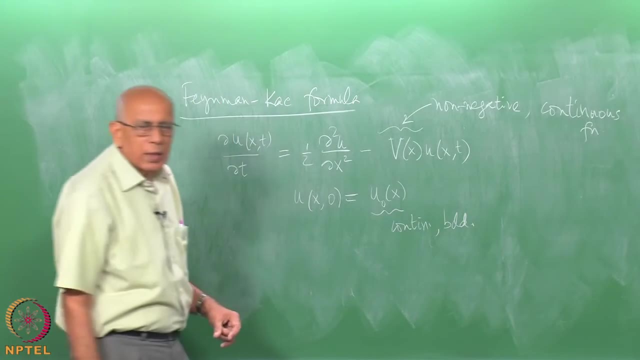 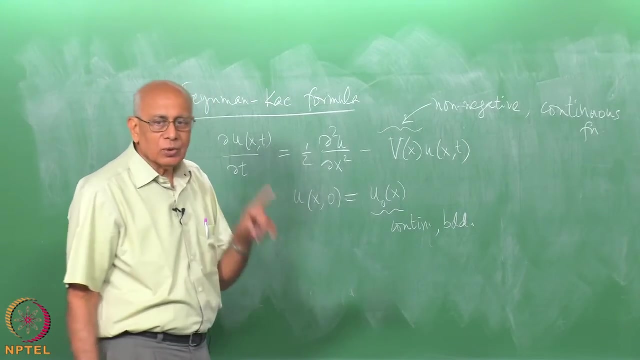 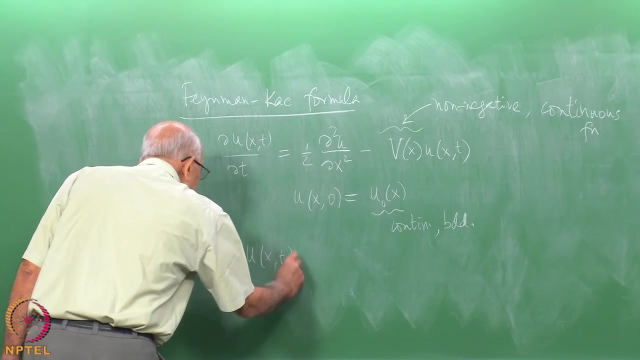 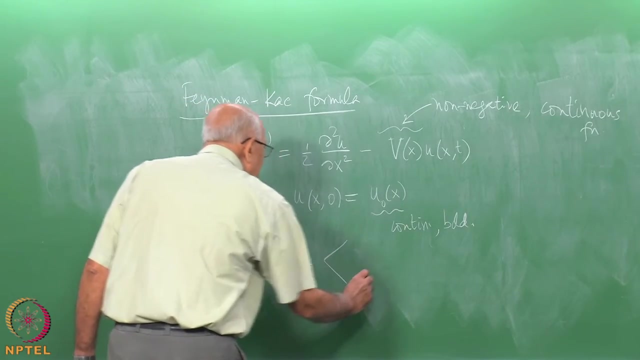 and we will assume this to be continuous bounded, So it is a continuous bounded function. Then the statement is that the solution of this, the unique solution of this, has the following form: It is equal to the average value of e, to the power minus integral. 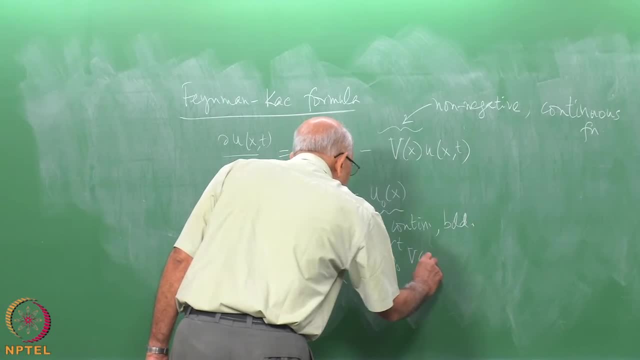 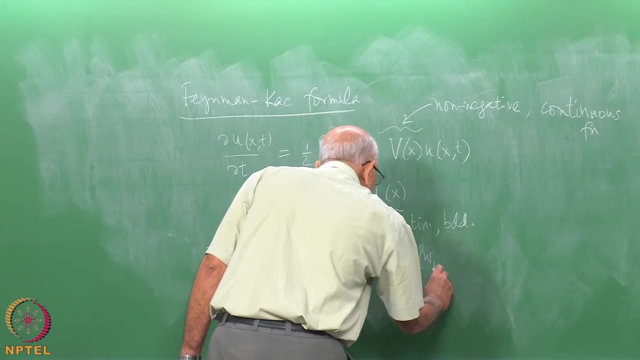 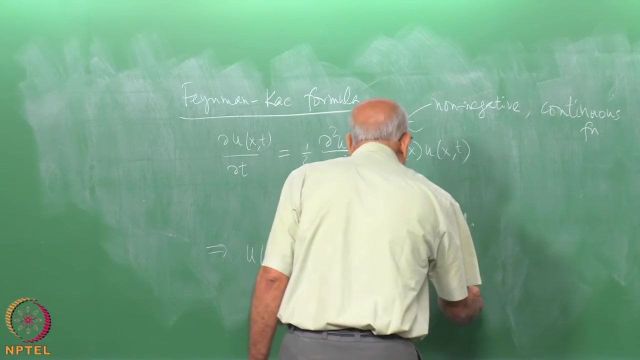 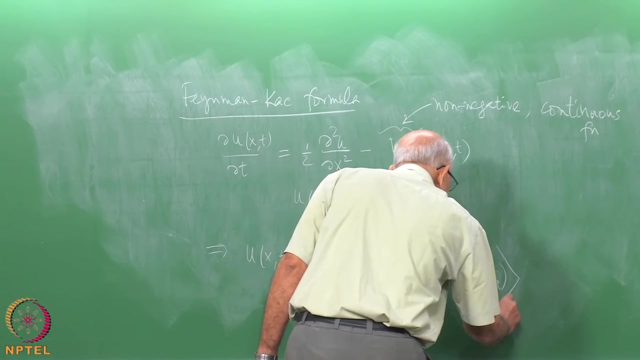 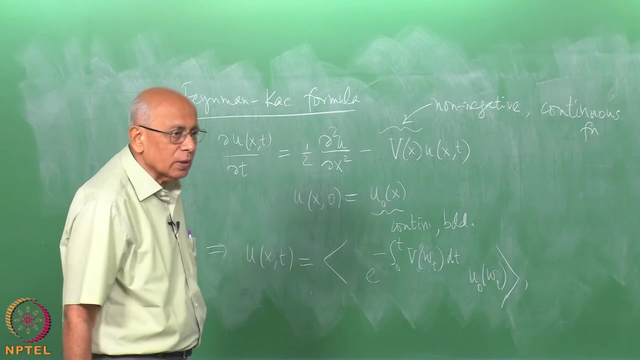 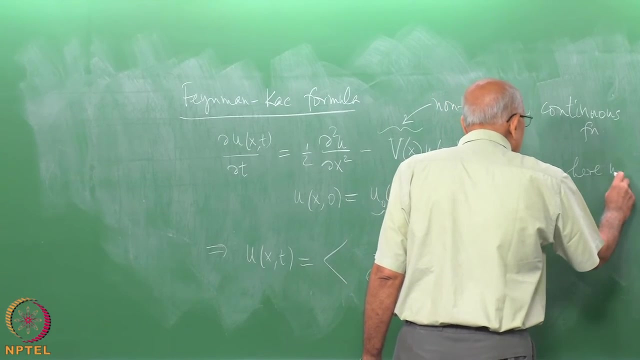 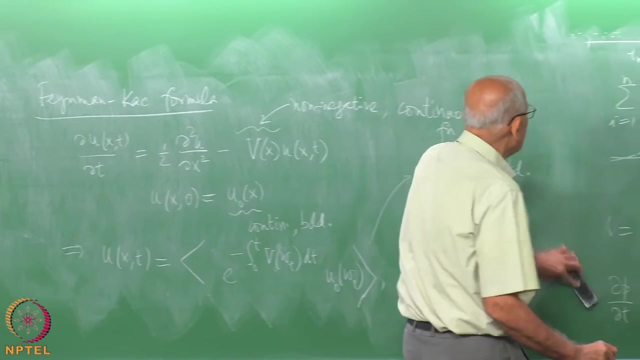 0 to t. v of x v of w t. dt times u naught of w t where I have to say what is w t and what this average is over. where w t equal to standard Wiener process or Brownian motion. 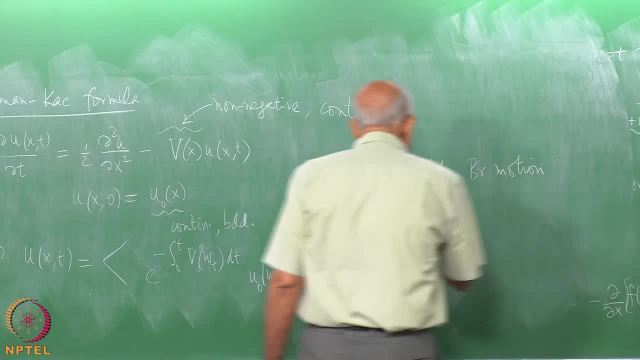 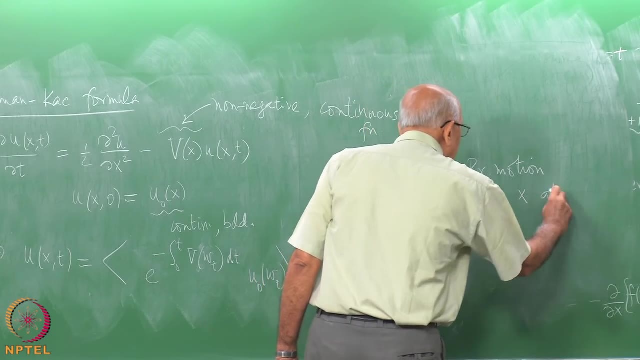 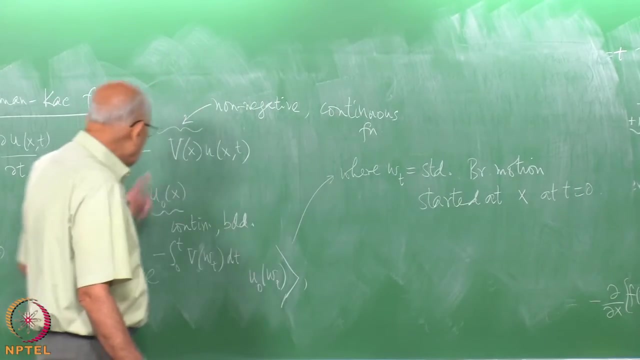 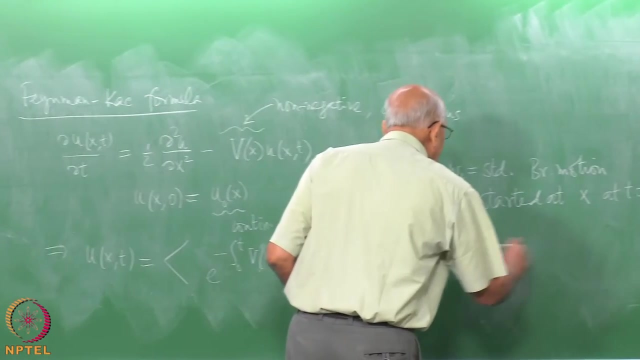 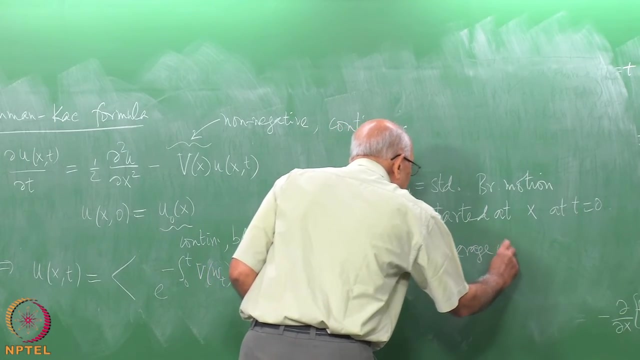 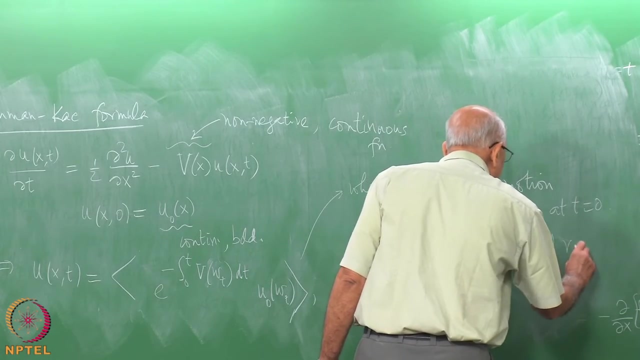 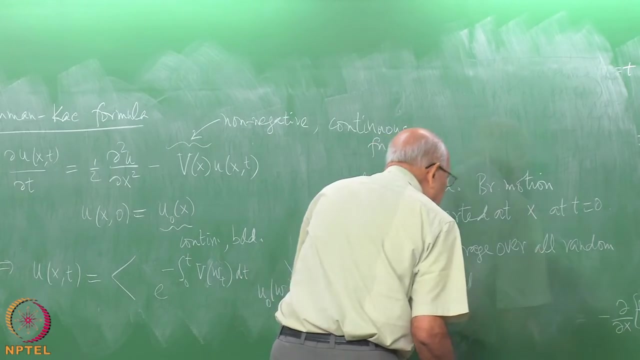 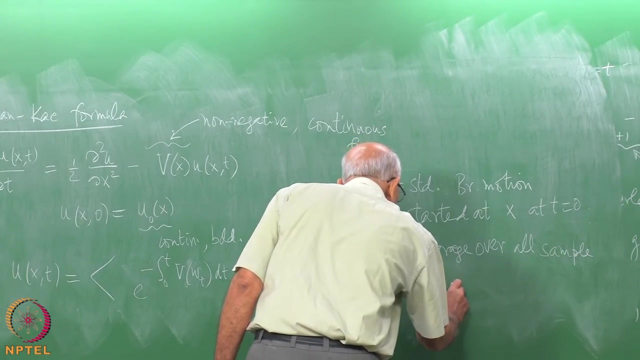 The Brownian motion started at x, at t, equal to 0.. So you have Brownian motion started from wherever you want the solution, whichever point you wanted it, and then you let it go and equal to average The Brownian motion over all, all walks, all random walks, all sample paths subject to. 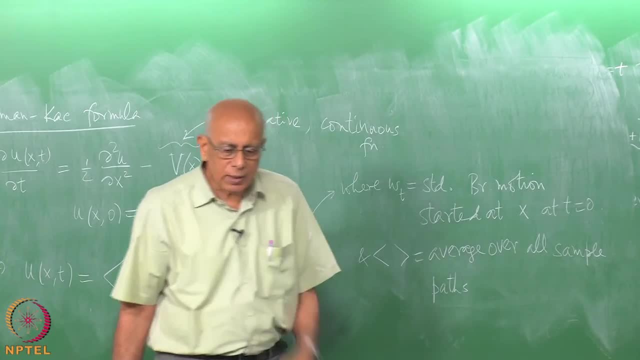 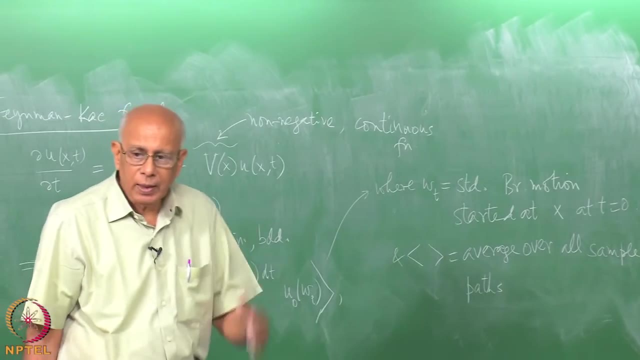 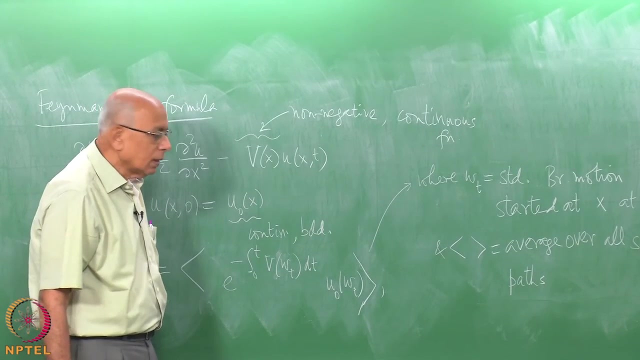 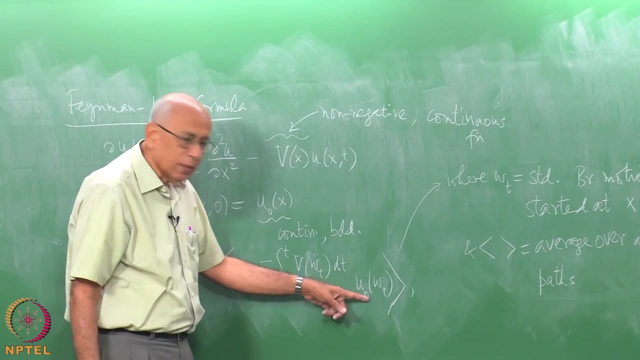 the above conditions, Namely all Brownian motions starting at x. This is going forward in time and then you do this integral. So this works both ways, If you want this, where you have an arbitrary functional out here and here some given functional. 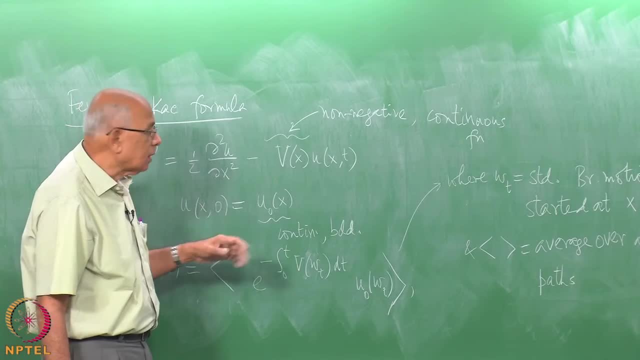 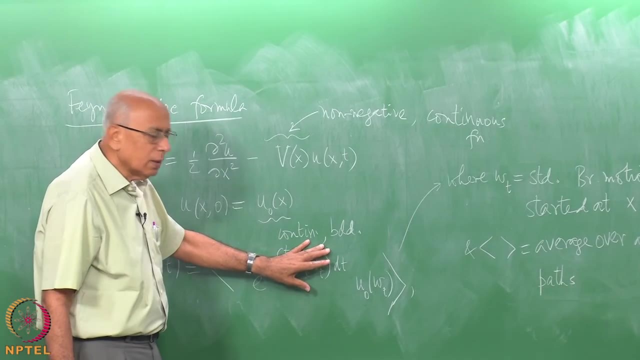 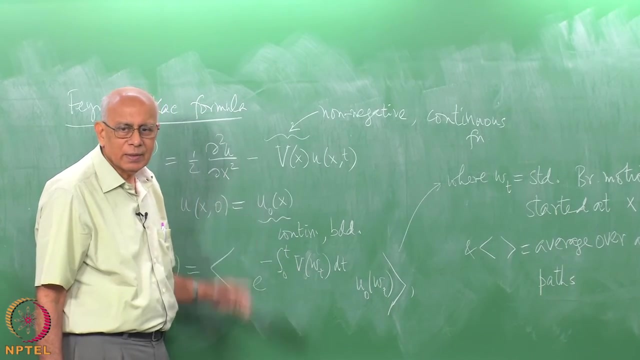 then you have this back again, Where the simplest case would be v equal to 0, then you see where this is coming from. You put v equal to 0, this goes away. You are going to take the initial point and you are going to put the Gaussian kernel and you are going to integrate. 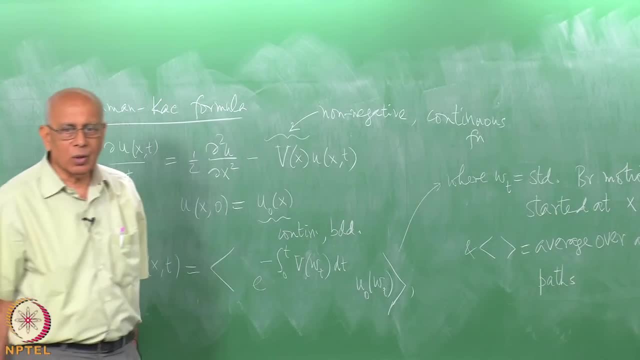 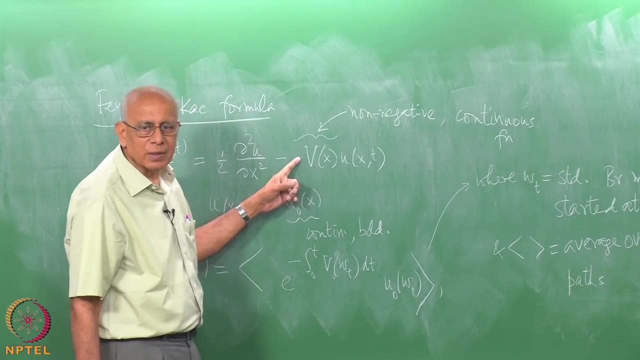 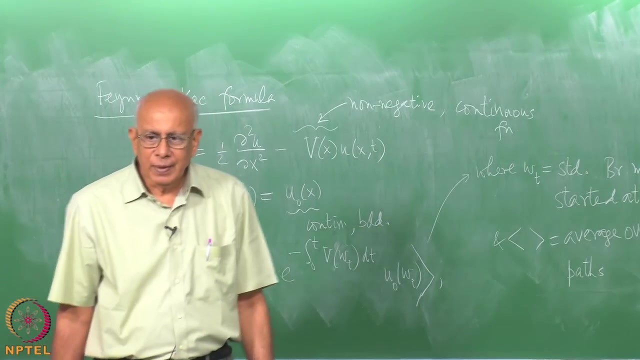 That would be one way of computing the average and that is exactly the solution we wrote down to the diffusion equation. But this generalizes it to the case of arbitrary functions here, subject to very mild conditions. Ok, And this is just the path. I mean, if you weak, rotate back. 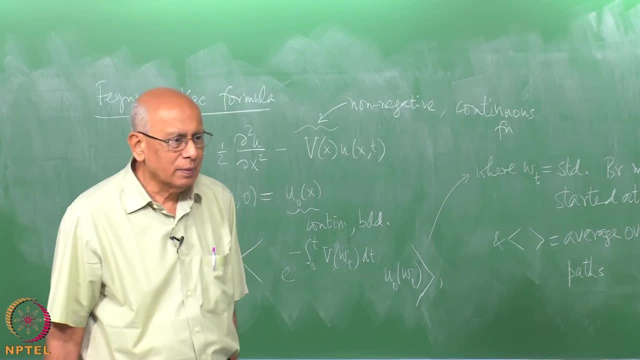 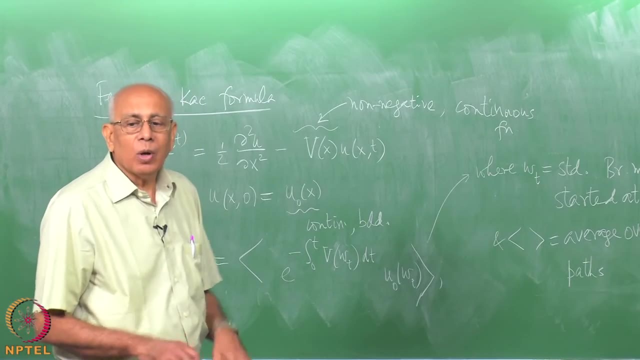 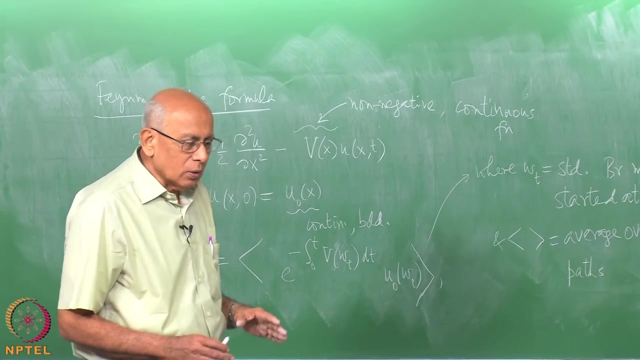 If you weak rotate back, it is just the path integral, Feynman path integral for the potential v of x, exactly. But what is interesting is this is capable of enormous generalization. First of all, to higher dimensional Brownian motion, for which we know how to write you. 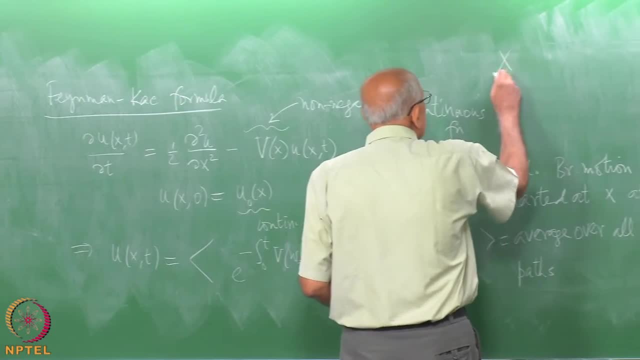 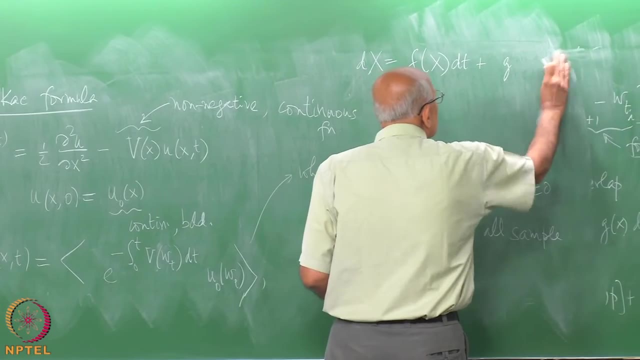 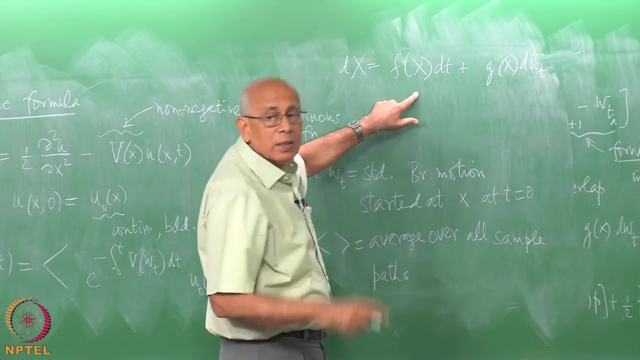 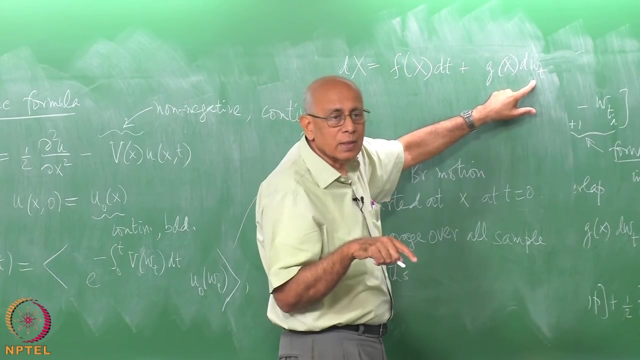 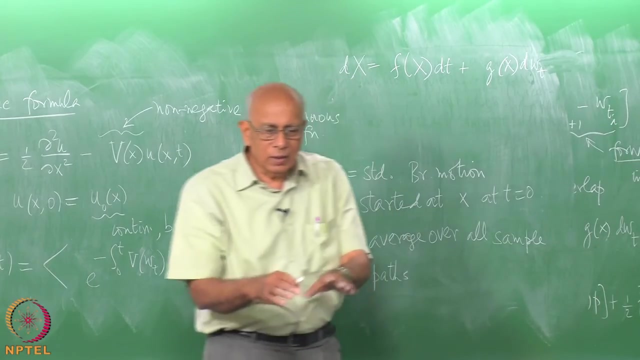 have a general equation of the form d, x equal to f, of x, d, t. Ok, Ok, Ok, So this is the n-dimensional vector. So is this: This is a new dimensional noise and this is an n times d matrix with suitable conditions on the g's. We know how to write. 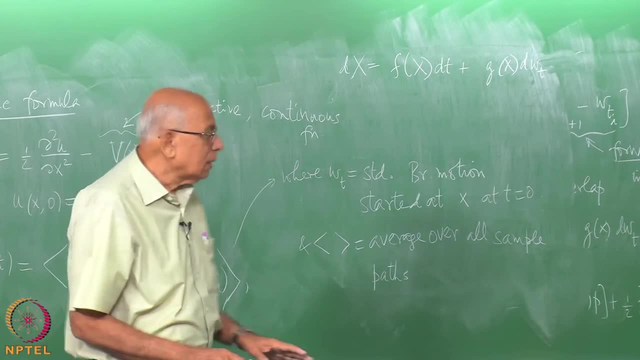 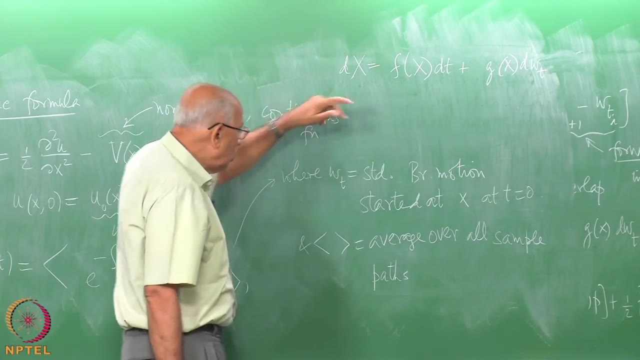 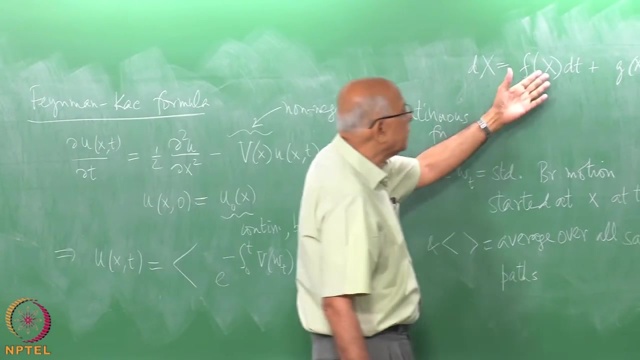 the Fokker-Planck equation down. Now for the process x. Ok, A general diffusion process x. You have an analog of this formula. It doesn't have to be standard Brownian motion alone. That would correspond to the case where F is 0 and g. 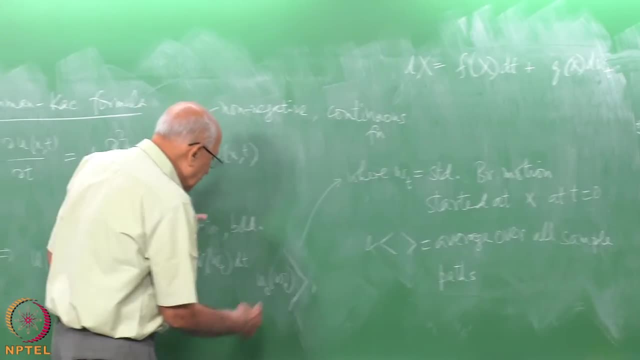 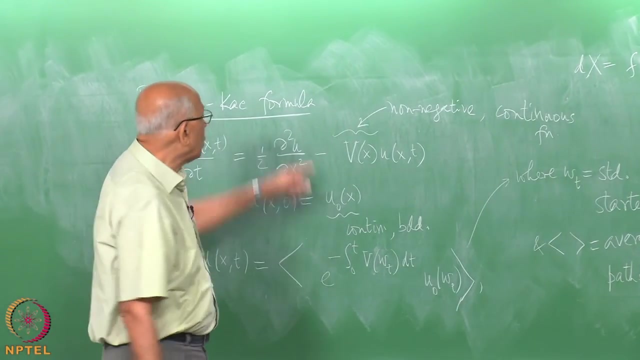 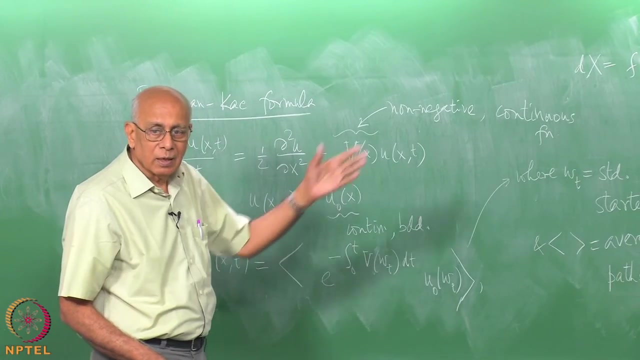 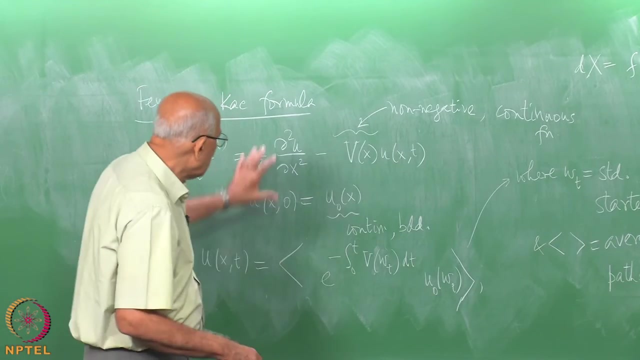 is 1.. But you can, instead of w, t, you can use x and you can write a generalized formula once again for a more complicated equation here, which involves the first derivative of this u with respect to x, with that drift term, And the second derivative with that diffusion term here. Ok, So, instead of this operator, 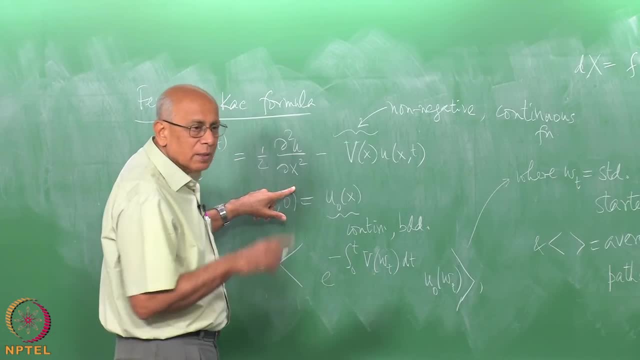 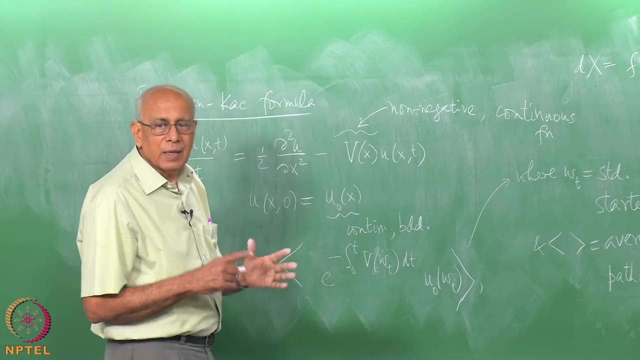 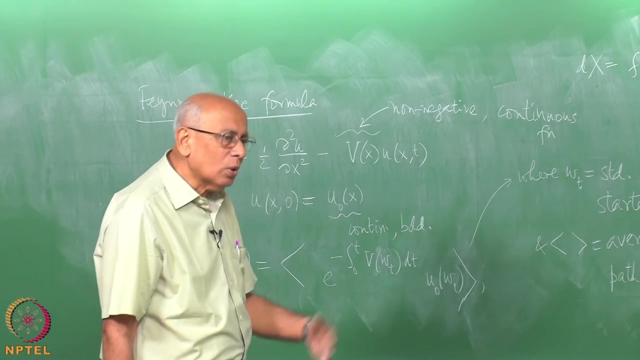 you replace it with g square times, this guy plus f times f of u, f of x, times the first derivative d? u over delta x, And it's still true. So higher dimensions, more complicated parabolic equations. it still works, this formula, And people have been understanding.